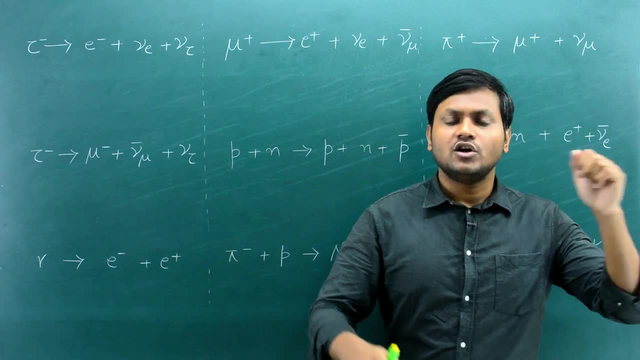 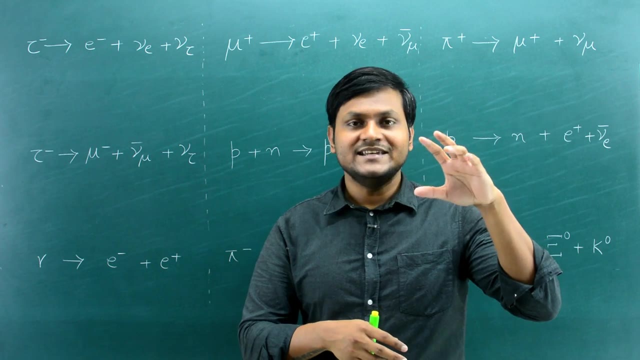 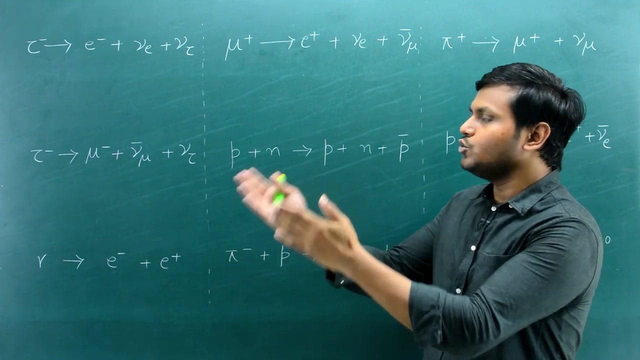 angular momentum and electronic charge, etc. etc. Apart from those conservation laws, as it turns out, when we are talking about interactions of elementary particles, then those interactions happen in such a manner that we can associate a certain set of numbers, namely the lepton quantum. 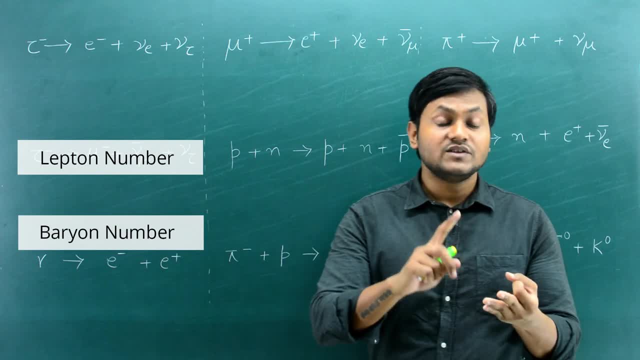 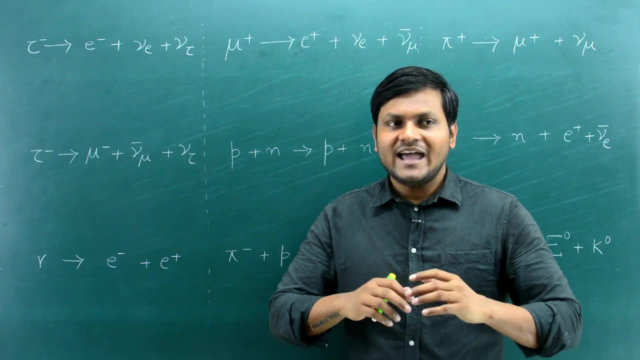 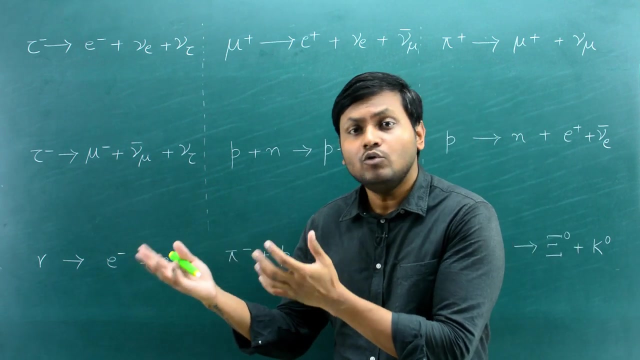 number, the baryon quantum number and the strangeness quantum number, which, as it turns out, is conserved in certain kinds of interactions And understanding. that will give us an idea about what kind of particle interactions are allowed in nature, what happen in nature and which of them do not happen. 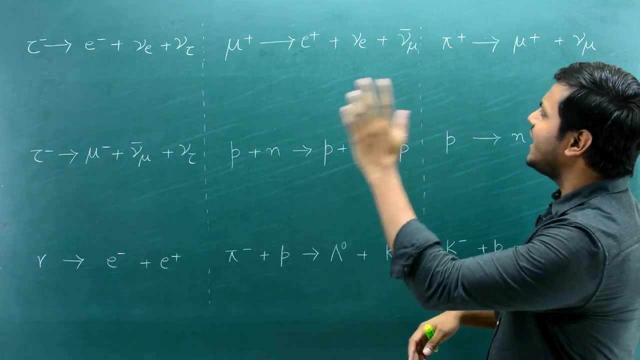 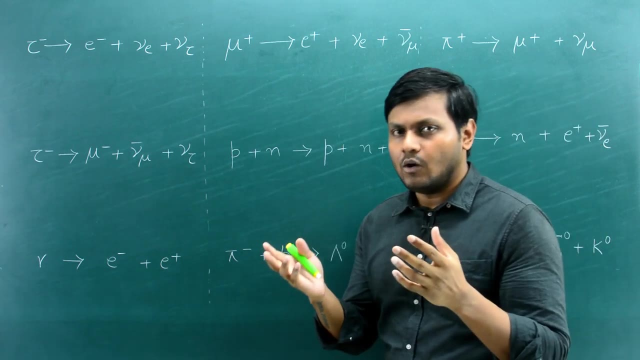 in nature. So, in a way, in this chaos of different kinds of particle interactions, you will have a little bit of an idea of which of them are allowed, which of them are not allowed. You will get a little bit of a confidence in this whole chaos of particle interactions. 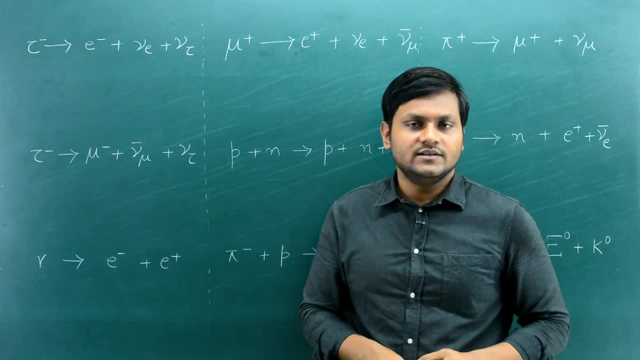 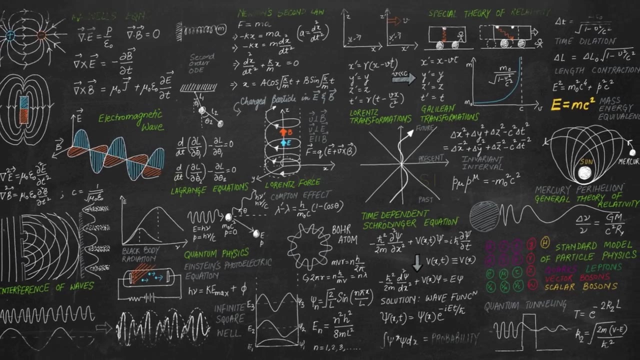 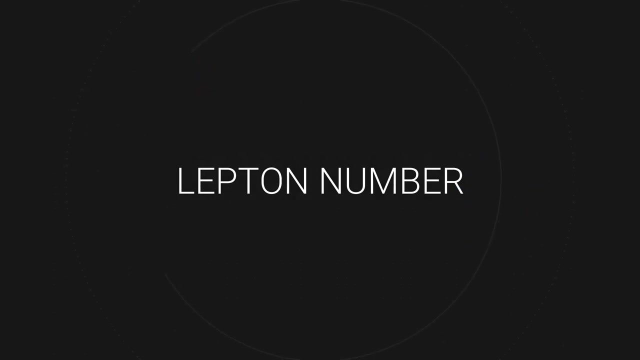 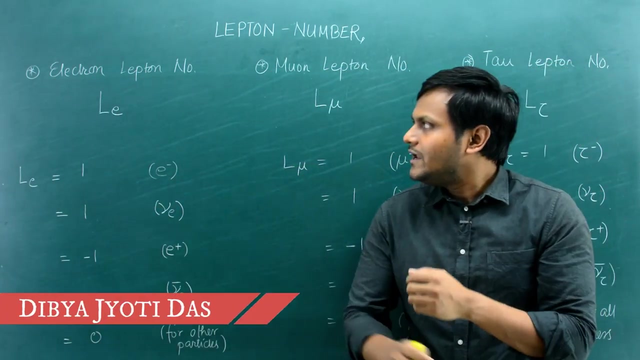 So that is what I'm going to talk about today in this video. So let us first talk about the lepton quantum number. So the lepton quantum number is a number that we can associate with particle interactions. So let us first talk about the lepton quantum. 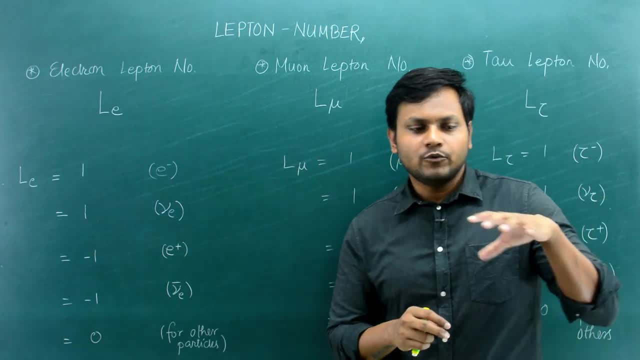 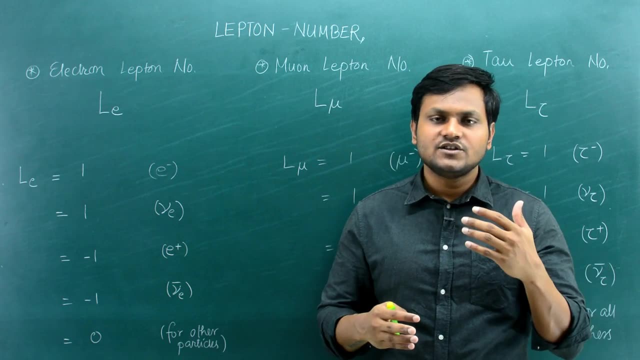 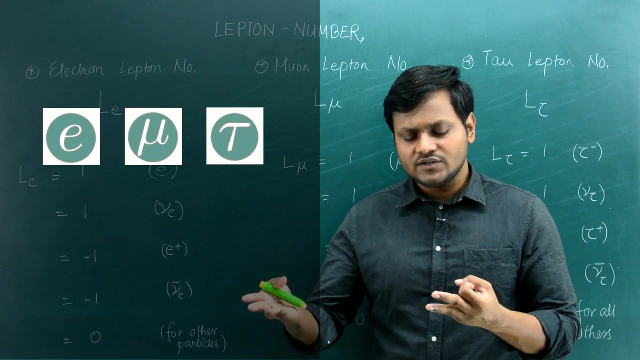 number. So let us first talk about the lepton quantum number. So let's first talk about the lepton number. Let us first talk about the lepton quantum number. So let us first talk about the lepton particles. Let's first talk about the. 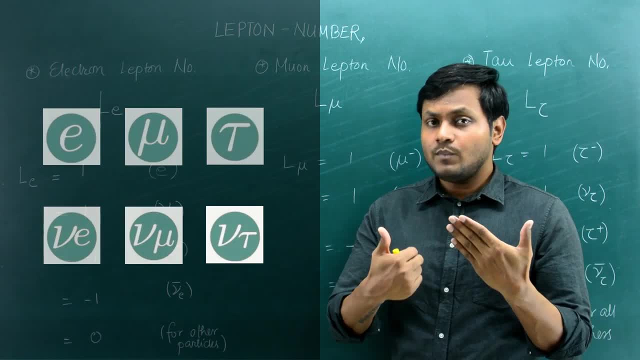 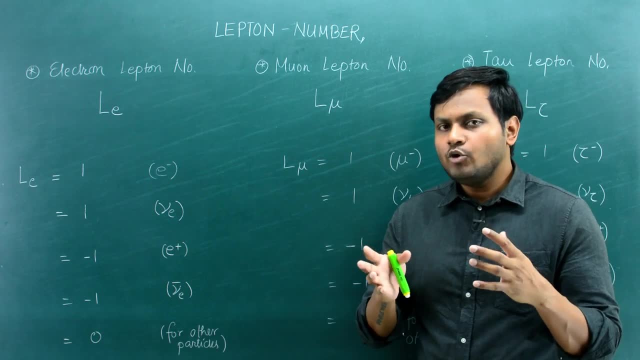 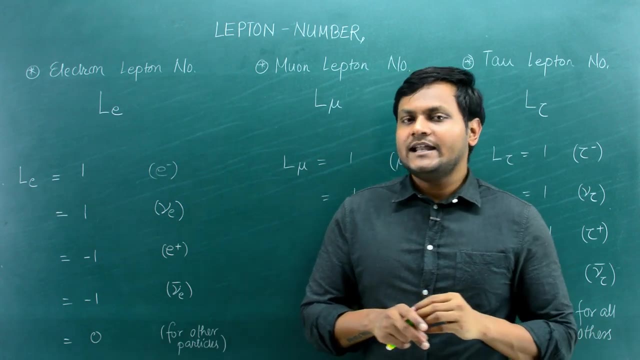 lepton particles. So we will see this in a bit which is the cardinal section. So after the lepton particles. Now, if you are interested in knowing more about leptons and their properties, I have made a video discussing leptons extensively. You can check out that particular video Here. I'm 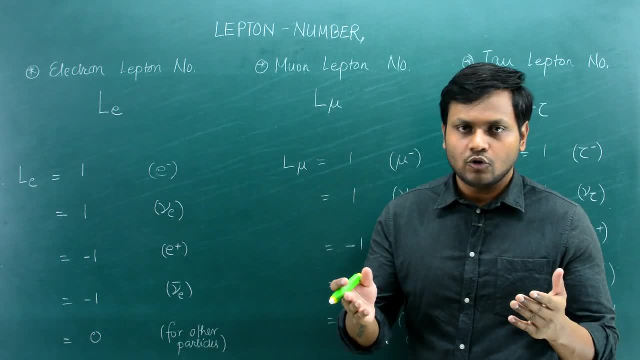 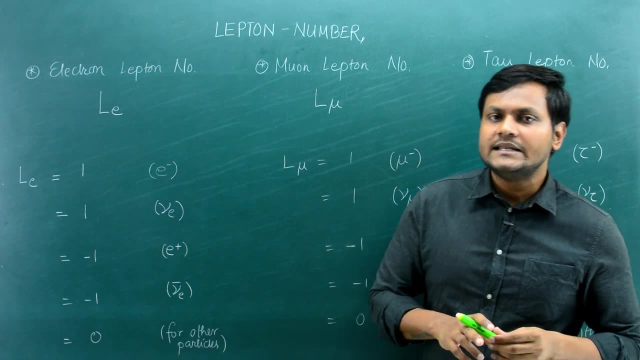 going to talk about particle interactions that involve these lepton particles. So the lepton particles either induce some kind of a particle reaction or they are the result of some kind of a particle decay. Now, as it turns out, whenever these particle interactions are taking place, 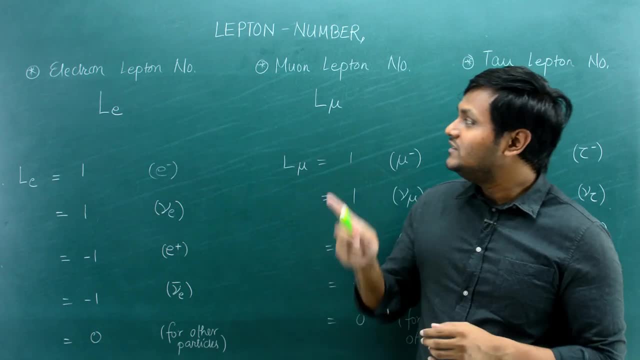 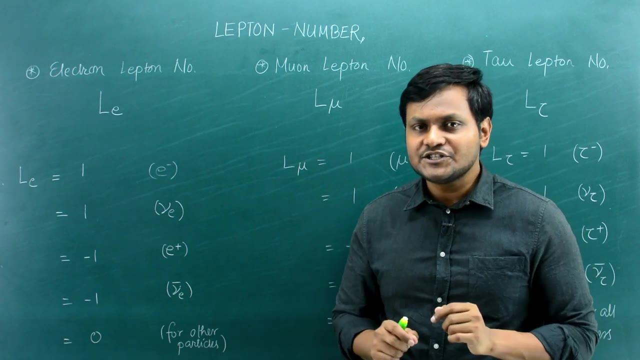 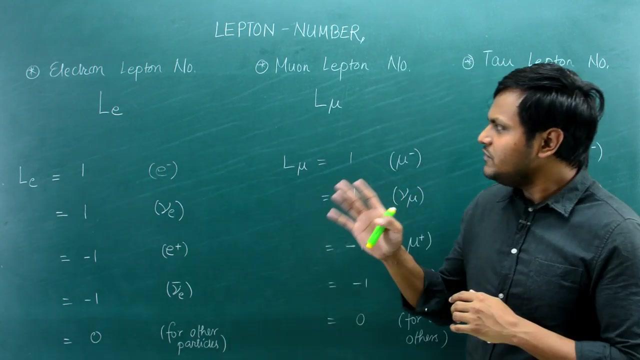 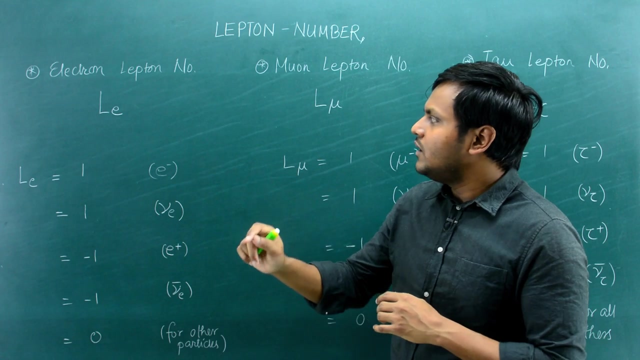 we can associate a number with these lepton particles, such that it turns out that these numbers, when added together before and after the interaction takes place, remains conserved. So before I talk about a couple of particle interactions, let me first define the values of these numbers. So I have three numbers: the electron lepton number associated with the 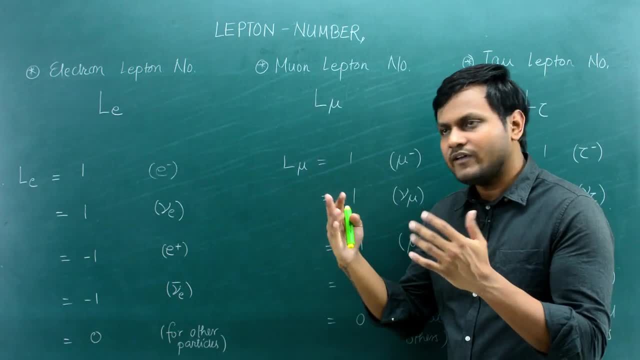 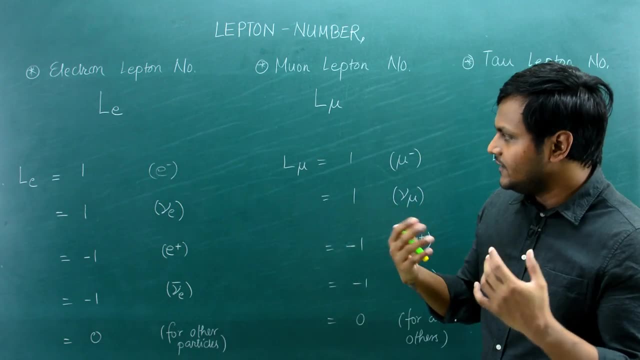 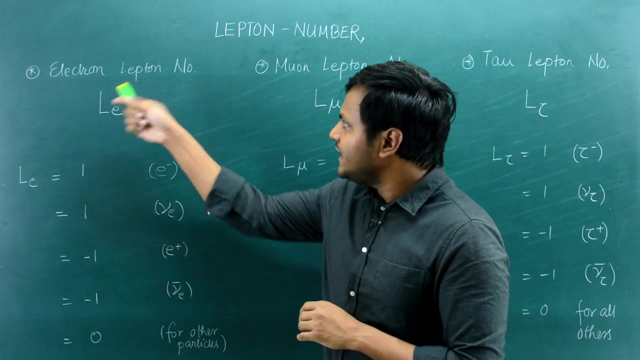 electron family, the muon lepton number associated with the muon family and the tau lepton number associated with the tau family, each distinct from one another, and we can associate values of 1, minus 1 or 0 for all particles, So, as it turns out, the electron 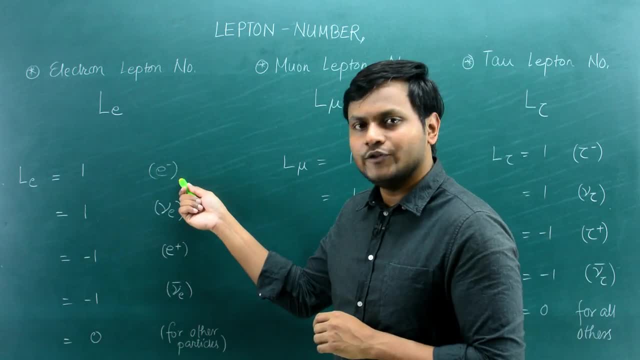 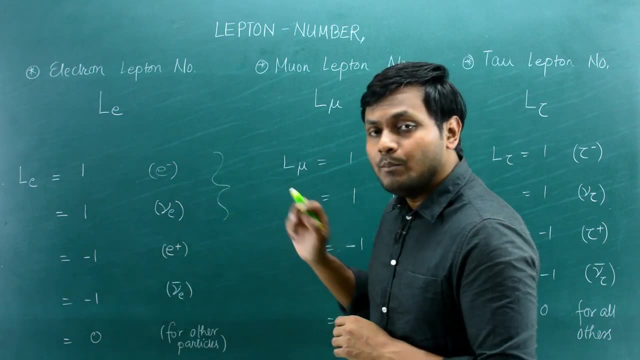 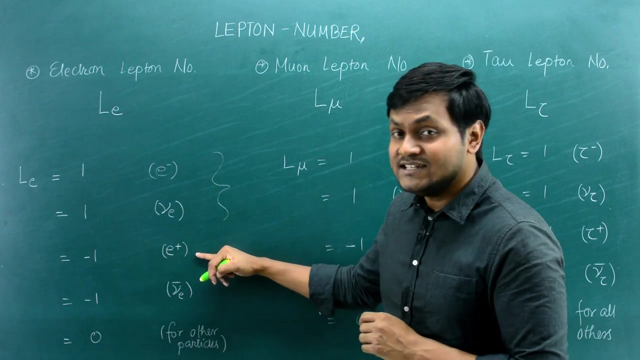 lepton number has a value of 1 for the electron. it has a value of 1 for the electron neutrino, but it has a value of minus 1 for their anti-particles. So it has a value of minus 1 for the anti-electron and it has a value of minus 1 for the anti-electron neutrino. 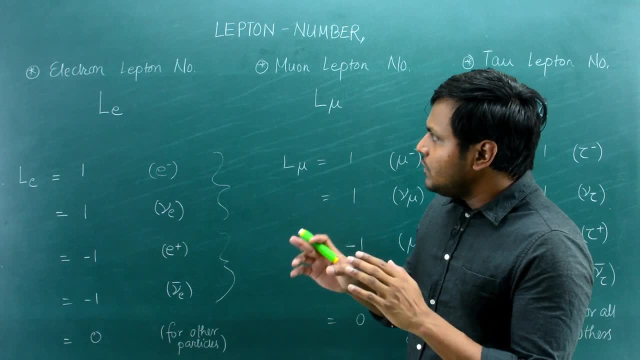 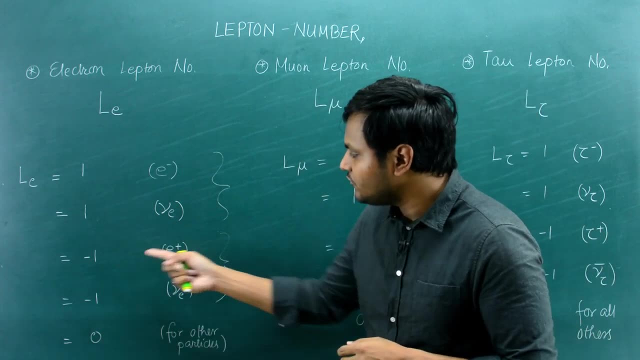 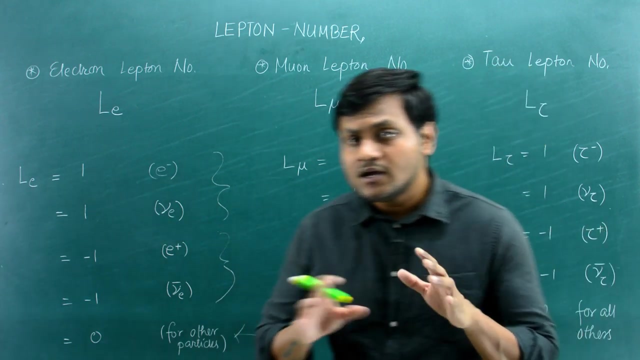 All right, let me repeat that again. the lepton number for the electrons has a value of 1 for the electron as well as the electron neutrino, but it has a value of minus 1 for the anti-electron as well as the anti-electron neutrino, while it has a value of 0 for all other particles. 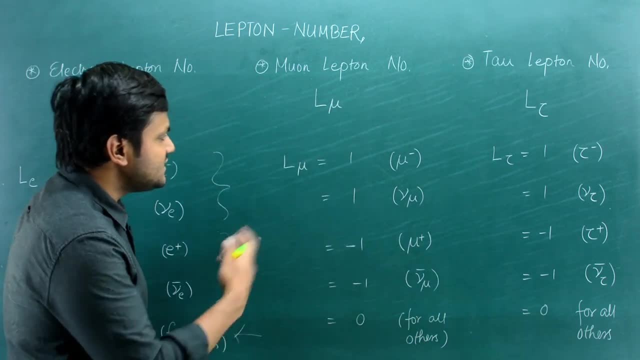 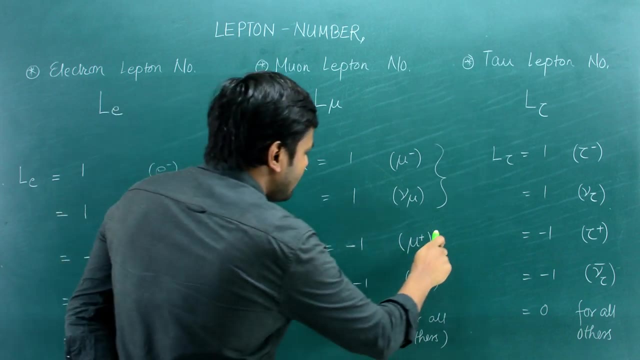 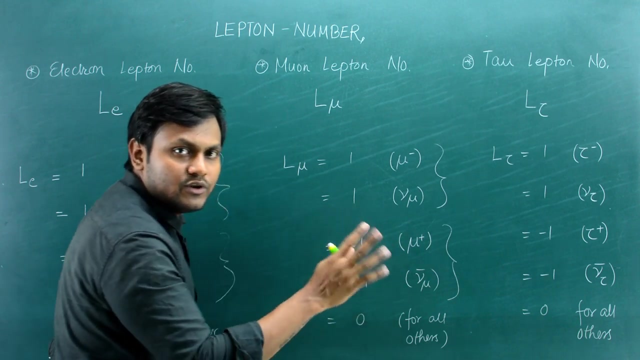 Similarly, we can associate a muon number which has a value of, in the same way, 1 for the muon particle and the muon neutrino, but it has a value of minus 1 for the anti-muon particle and the anti-muon neutrino, All right, and it has a value of 0 for all other particles. 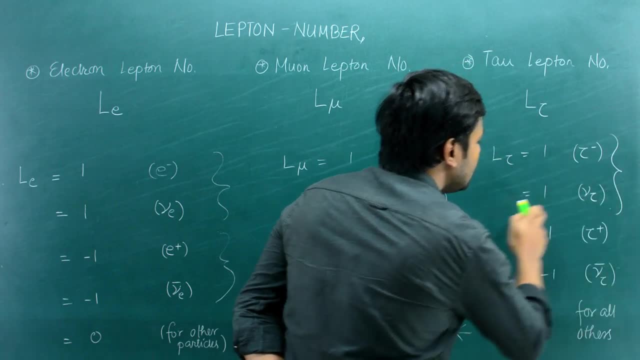 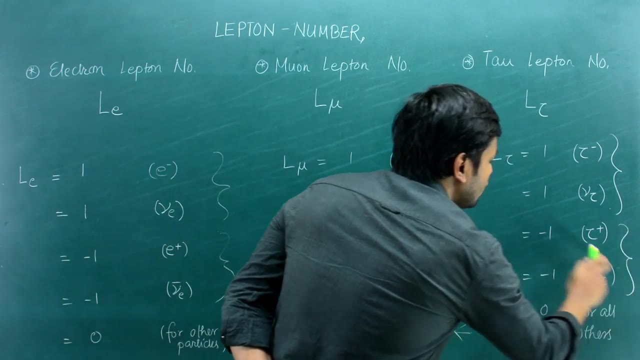 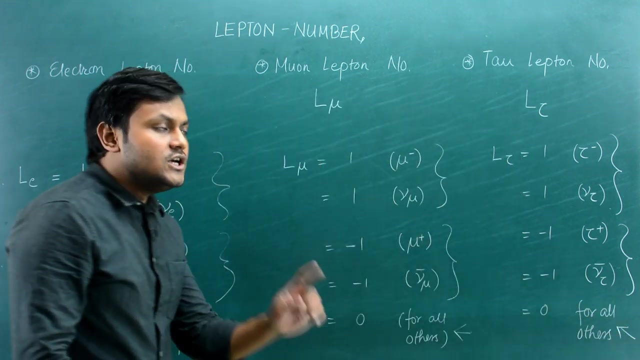 Similarly, the tau number can have a value of 1 for the tau particle and the tau neutrino, but it has a value of minus 1 for the anti-tau particle and the anti-tau neutrino. it has a value of 0 for all other particles. So, even though these three numbers are distinct from 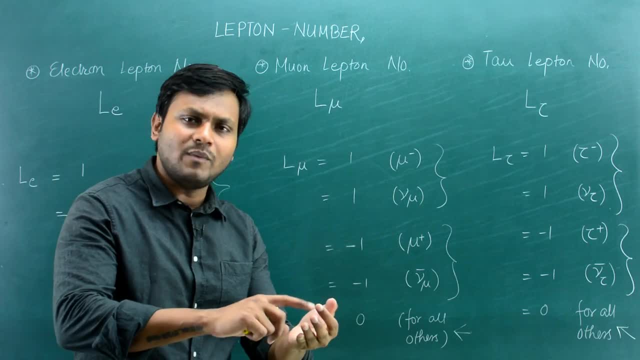 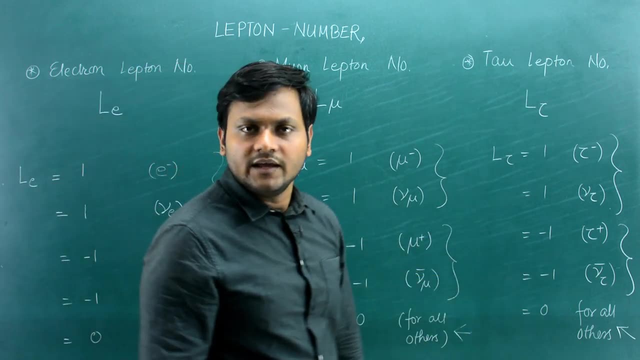 one another. their values could be similar: 1,, 0, minus 1.. 1 for the particles, minus 1 for the anti-particles and 0 for everything else. So for the electron-leptron number you have 1. for the 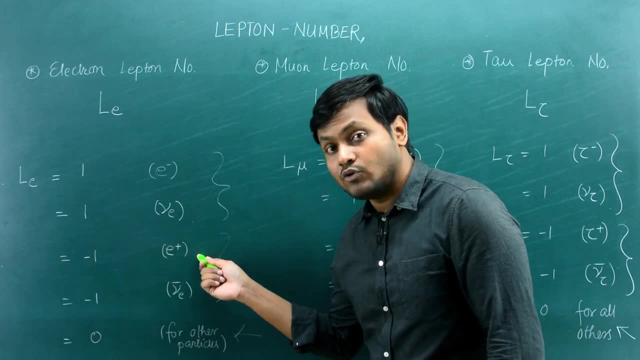 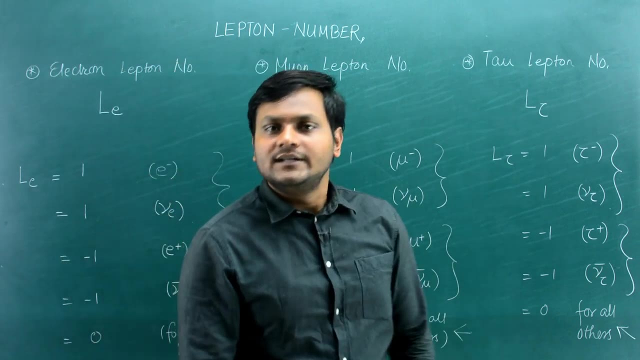 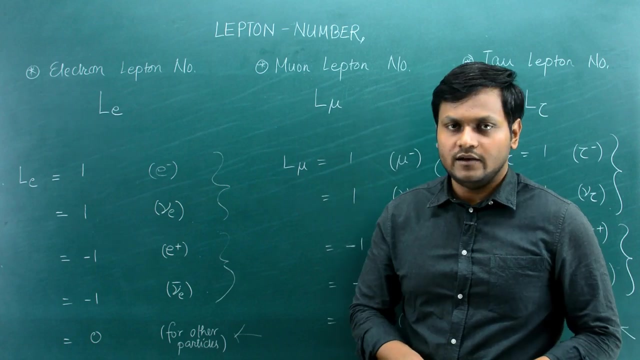 electron and the electron neutrino, minus 1 for the anti-electron and the anti-electron neutrino, 0 for all others. Similarly for the muon-leptron number and the tau-leptron number. Now we can use these numbers in different kinds of particle interactions to see that they do indeed remain. 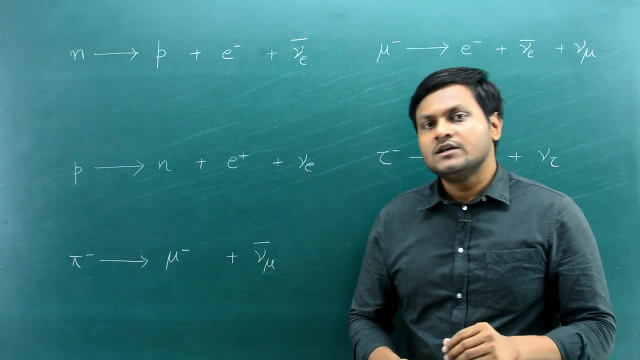 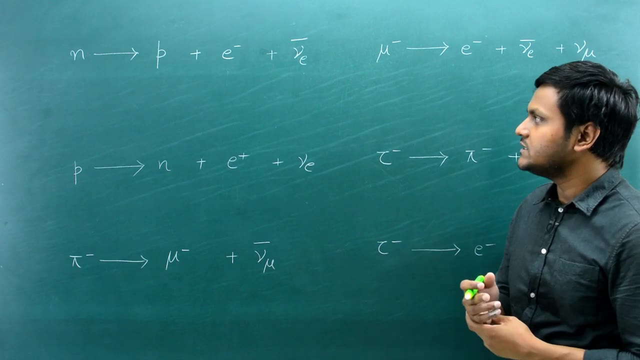 conserved. So here is a bunch of particle interactions that do happen in nature, which involve leptron particles And, based on what we just now discussed, let us see if we can associate the leptron number with the electron number. So let us see if we can associate the 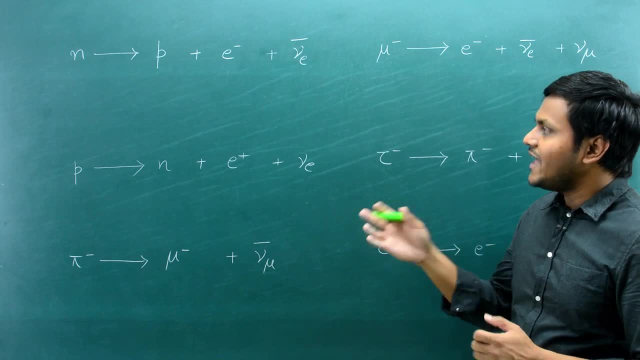 leptron number with the electron number. So let us see if we can associate the leptron number with these numbers that I talked about in these reactions and see whether or not they are conserved. So let us first start with this reaction here, or this interaction, which is: 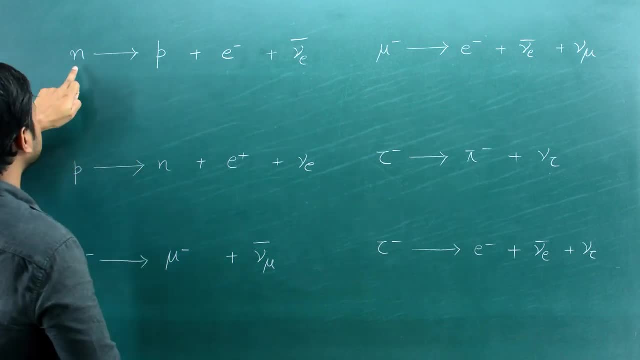 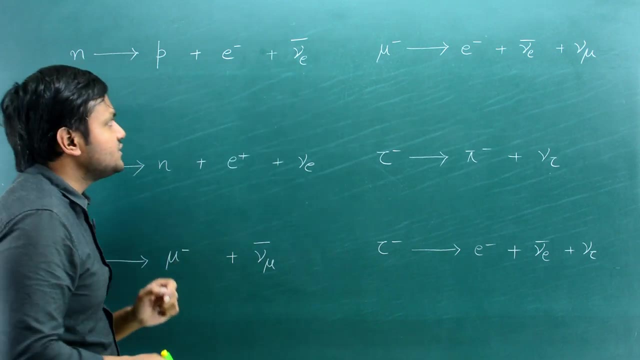 nothing but the negative beta-dk reaction, in which case a neutron becomes a proton, leads to the emission of an electron, or the beta particle, and an electron-anti-neutrino in the process. Now this interaction involves electron and electron-anti-neutrino. 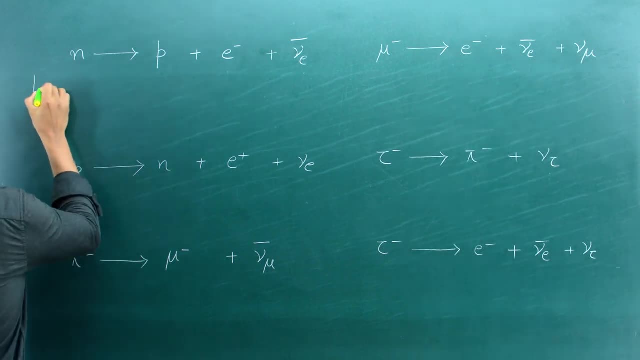 So in this case I am only going to look at the lepton number for electrons, or the electron number, right? So what is the electron-lepton number? for a neutron and a proton? They are nothing but 0, all right. For all other particles they are 0, right, Remember. 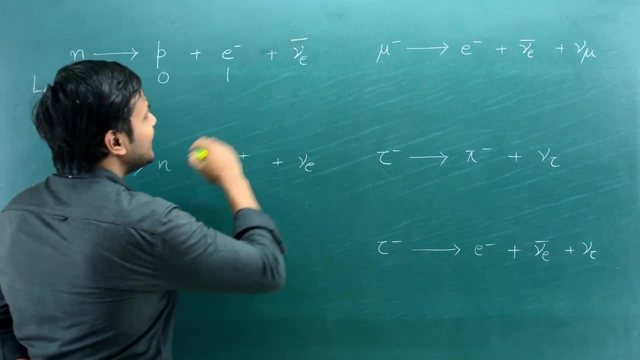 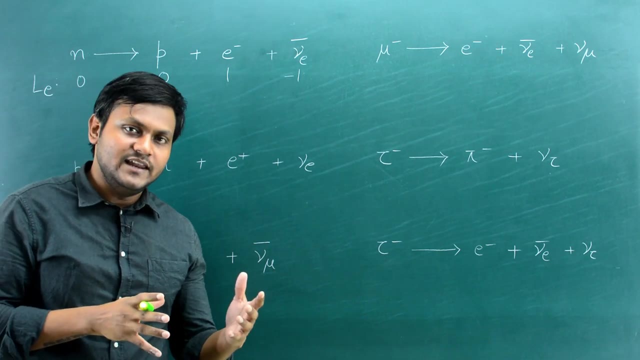 But for the case of an electron it is 1.. For the case of an electron-anti-neutrino, it is minus 1.. Now, these quantum numbers are additive in nature. additive in the sense that you can add these quantum numbers in the left-hand side and the right-hand side and you can see whether or not. 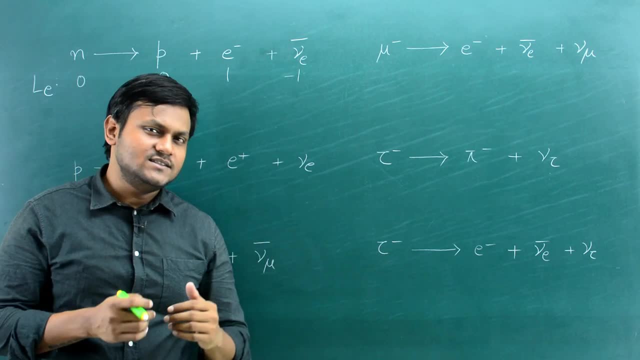 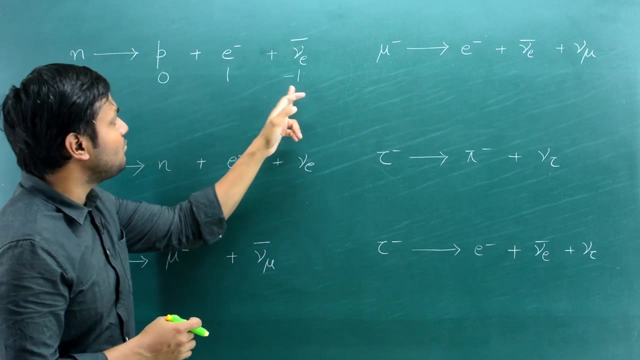 that particular summation is conserved or not. So in the left-hand side, the lepton quantum number has a value of 0.. On the right-hand side it has a value of 1 minus 1, which is nothing but 0. That means in this case: 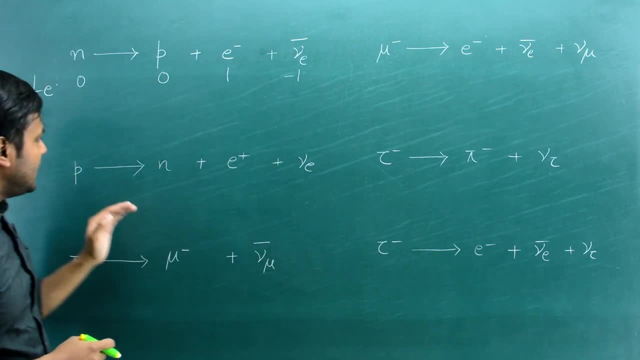 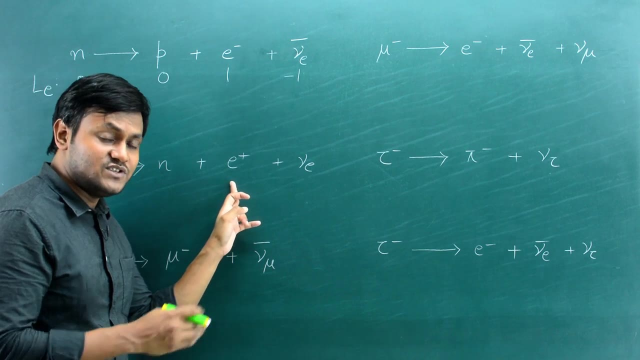 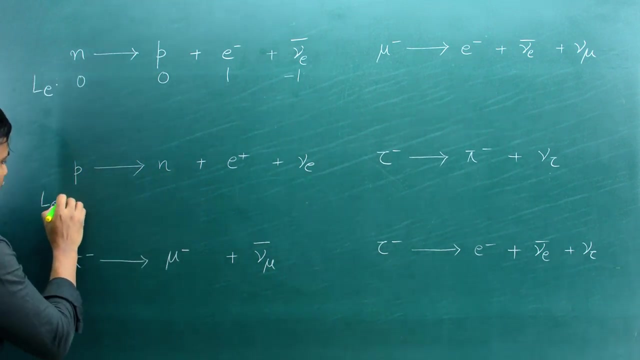 this is conserved. right Now let's go ahead to the next interaction, which is the positive beta-dk, in which case a proton becomes a neutron, leads to the emission of a positron, which is an anti-electron and also an electron-neutrino in the process. So if I look at the same electron-lepton, 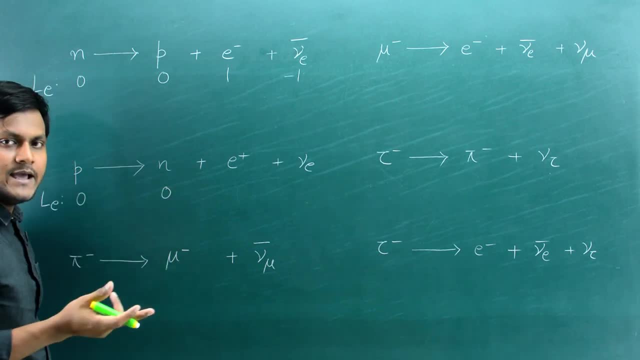 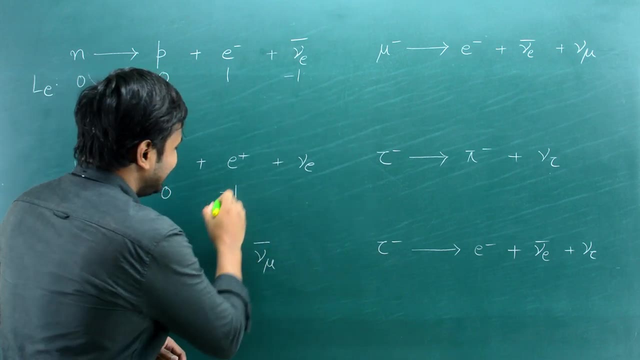 for a proton and a neutron they turn out to be 0, right, But for the case of an anti-electron, it has a value of how much, You remember, Minus 1, yes, But for the case of an electron-neutrino. 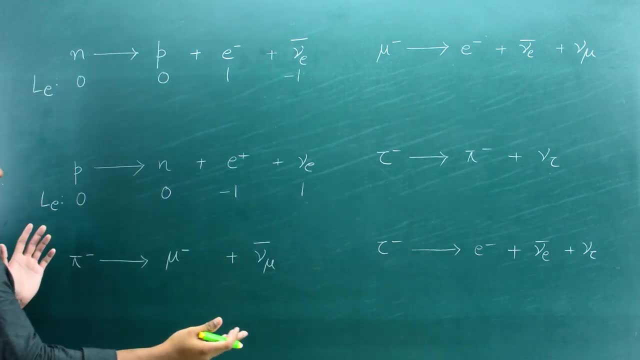 it has a value of plus 1, right Again, left-hand side, it has a value of 0.. Right-hand side, the summation of these two numbers has a value of 0. That means the lepton quantum number for. 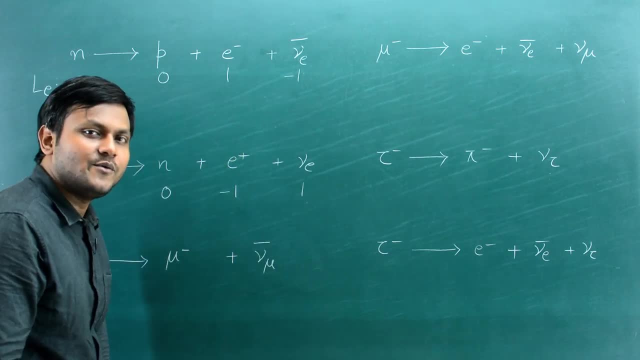 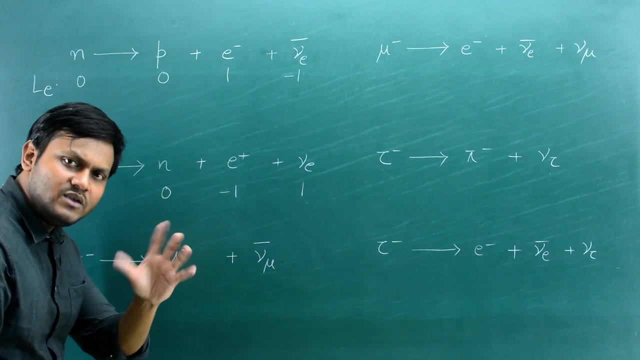 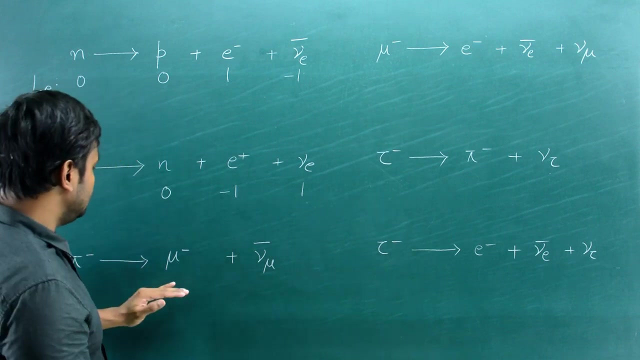 the electrons in this case- is conserved. right, Let's go ahead to the next. So this is a case of a decay involving a pi-mison, So free pi-misons can decay into muon particles and lead to the emission of an anti-muon neutrino. This interaction does not involve either electrons or 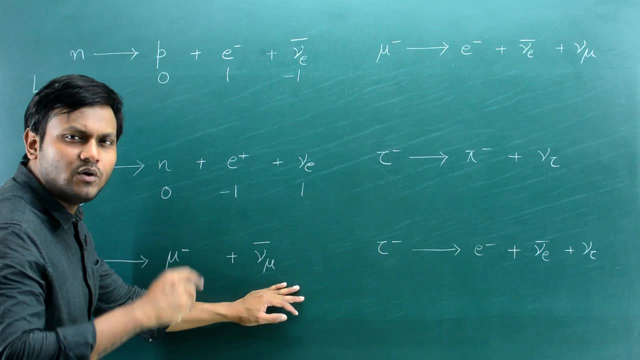 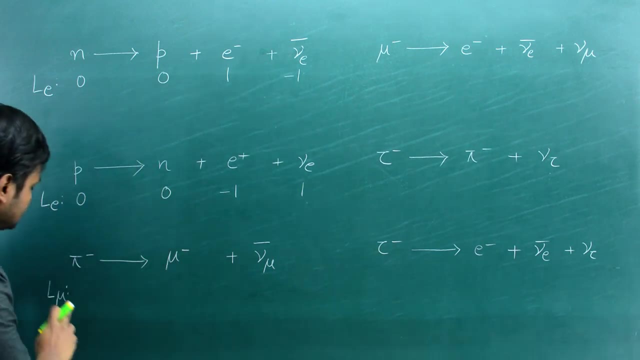 electron-neutrinos, but it involves muons and muon-neutrinos, right? So we are going to look at the muon number in this case, okay, So what is the muon-lepton number for a pi-mison? It is 0.. 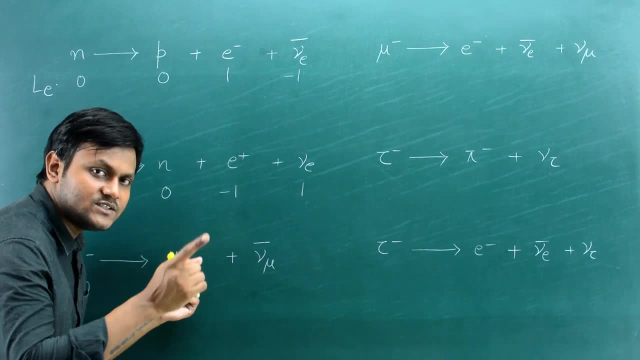 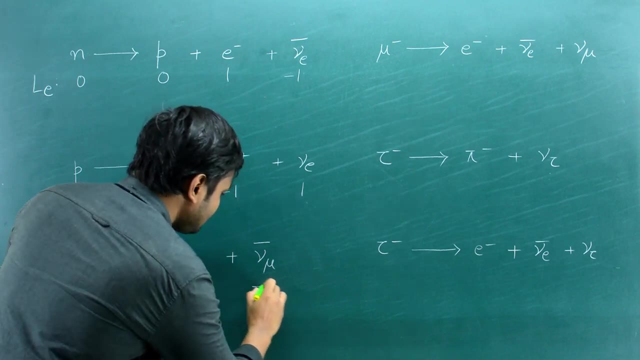 What is it for a muon particle, Remember? And what is it for a muon anti-neutrino? It is minus 1.. Again, muon-lepton numbers are additive. that we look at the sum on the left-hand side and the right-hand side. So on the left-hand, 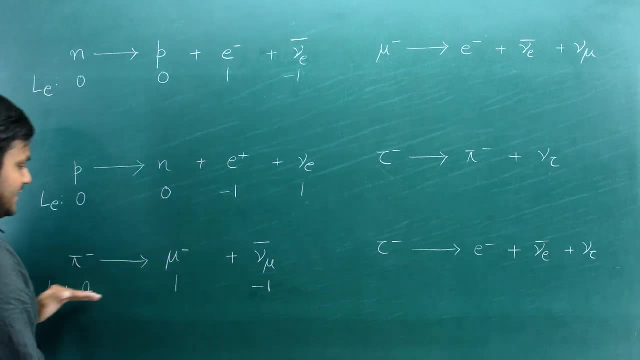 side is a value of 0, right-hand side is a value of 1 minus 1, 0.. Again, the muon-lepton number is conserved. Now what happens to a muon particle once it is formed? A free muon particle can decay. 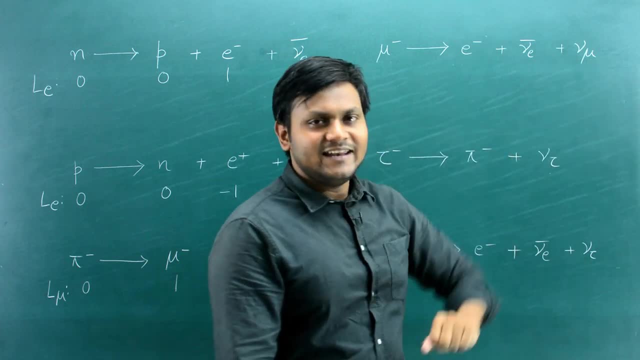 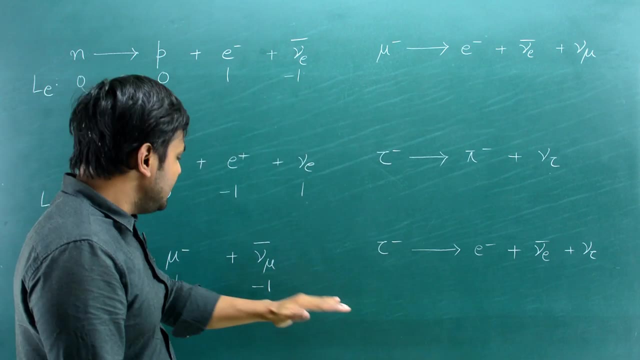 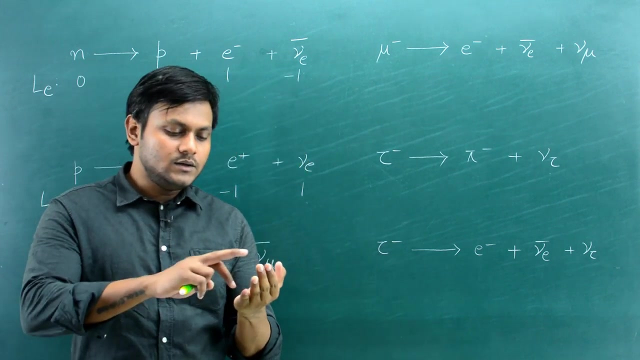 into an electron, electron anti-neutrino and a muon-neutrino. Now, this kind of an interaction involves both the particles from electron family as well as from the muon family, So we need to check them separately, because I told you that the electron number, the muon number and the tau 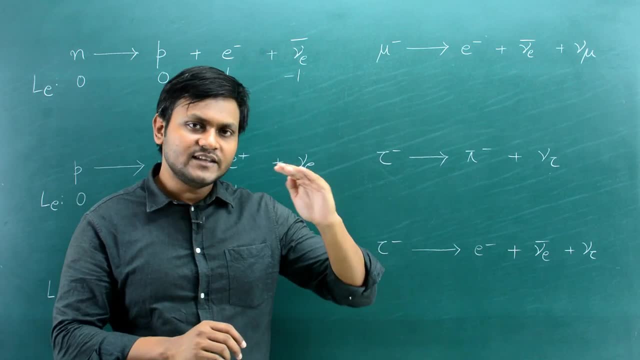 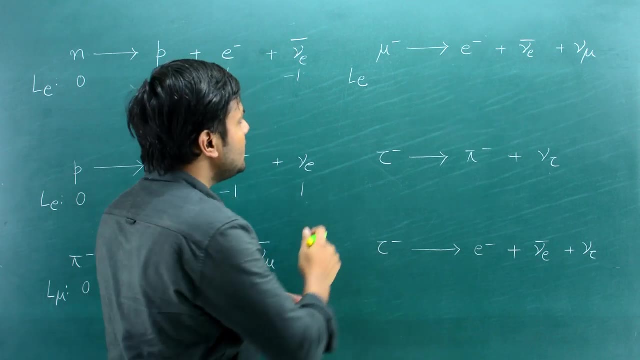 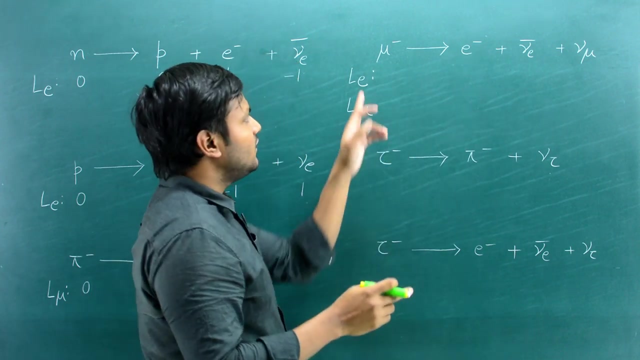 number. they are distinct and we need to check their conservation separately. So first we will check their conservation associated with the electron-lepton number and then we will check the conservation associated with the muon-lepton number. So what is the electron-lepton number for? 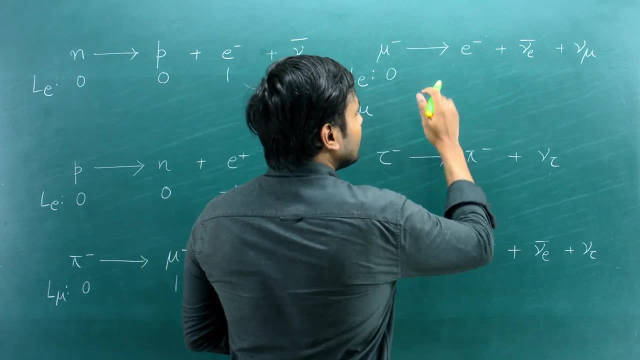 an electron-lepton particle: It is 0,. right? What is the electron-lepton number for an electron particle? It is plus 1. for an electron anti-neutrino, it is minus 1. for a muon-neutrino it is 0,. 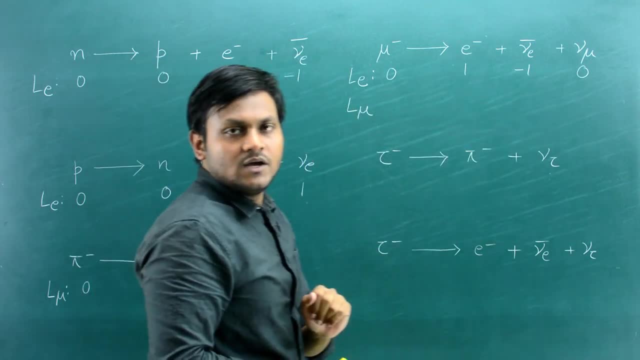 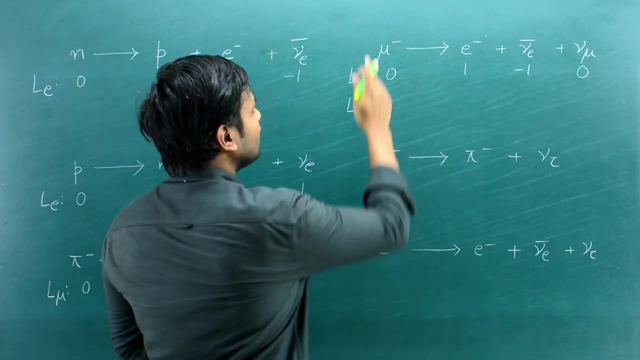 right It is conserved. left-hand side: 0,. right-hand side summation of 1 minus 1 comes out to be 0.. Now let us look at the muon-lepton number. What is the muon-lepton number for a? 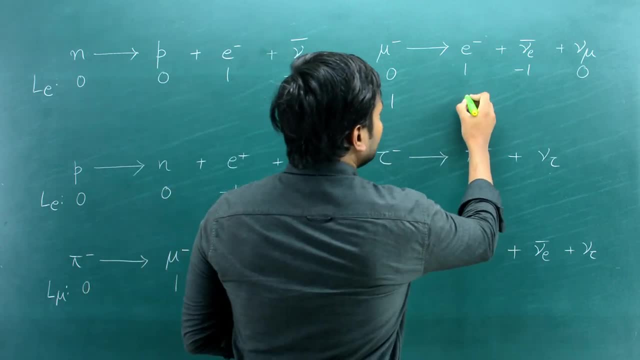 muon particle: It is 1.. What is the muon-lepton number for an electron particle? It is 0.. What is the muon-lepton number for an electron anti-neutrino? It is 0.. And what is the muon-lepton? 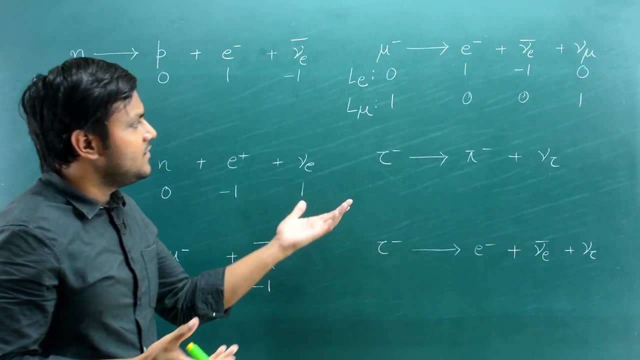 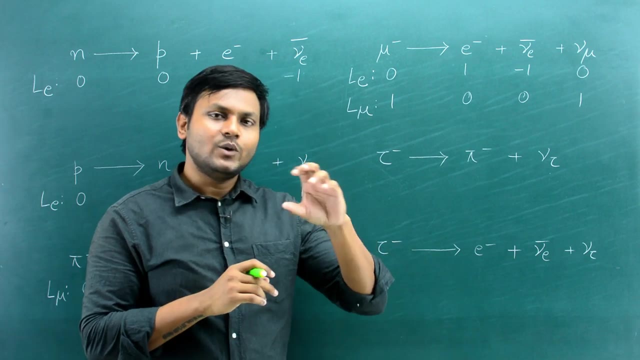 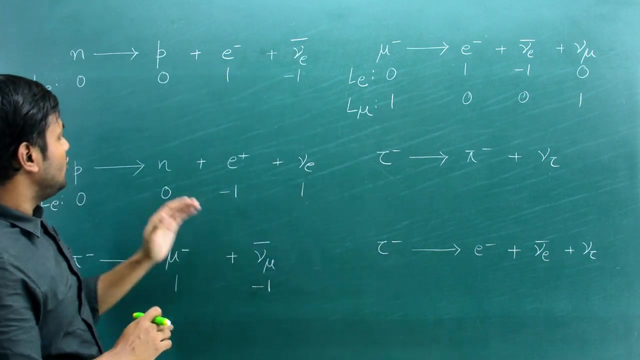 number for the muon neutrino. it's one. it's conserved right left hand side one, right hand side one. so these quantum numbers are additive. that means you can add them on the right hand side as well as on the left hand side, and you can check for their conservation now, once you get to. 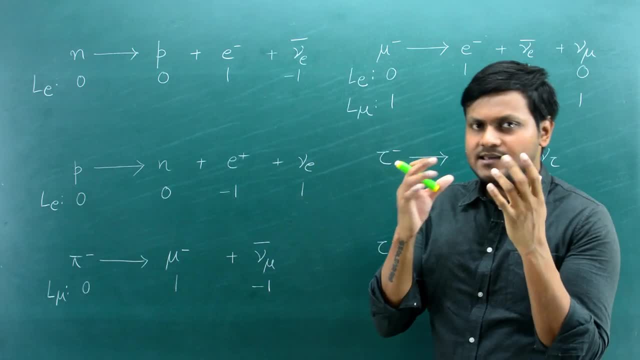 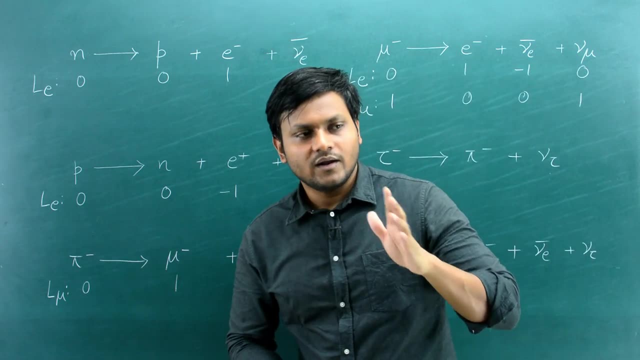 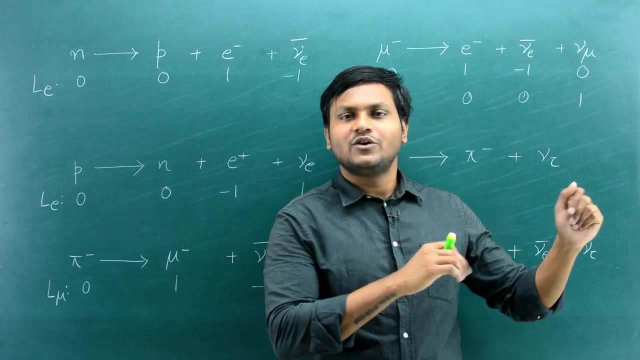 know about the electron lepton number, muon lepton number. it gives you an idea about what sort of interactions are possible and what sort of interactions are not possible, because sometimes in examinations you are asked questions about: uh okay, complete this particular reaction or tell us whether or not this reaction is possible or not possible. and once you get an idea about this, 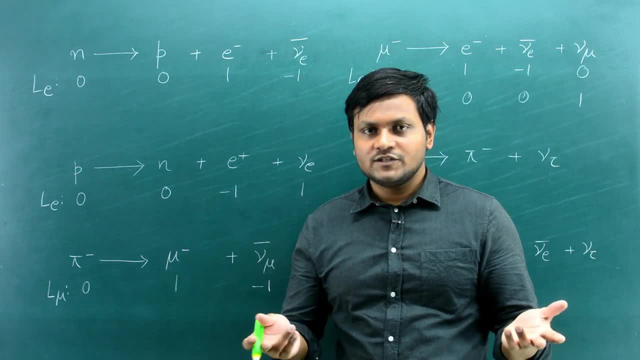 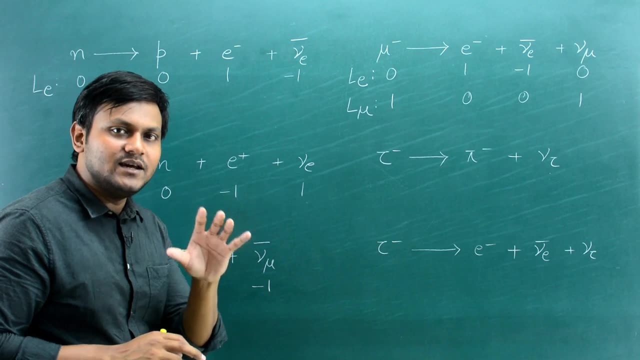 then you can get an idea about which of the reactions are possible and even predict which particle is going to involve. so let me give an example. i'm sure that every time you studied beta decay, you were confused at one point whether, along with the electron, an electron 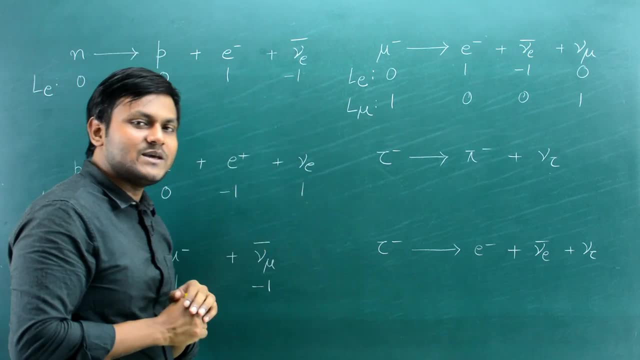 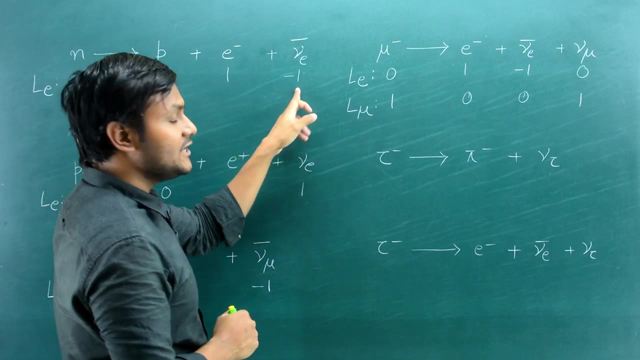 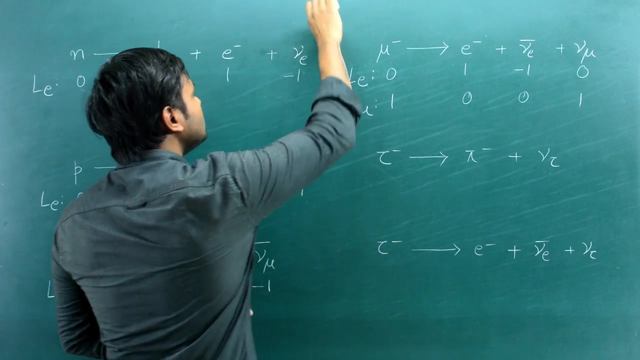 anti-neutrino was emitted or an electron neutrino was emitted. i'm sure most of you were confused at some point. so in this case, if an electron is emitted along with an electron anti-neutrino, you get one and one lepton number, which remains conserved. right, but is this reaction possible? can an electron be emitted with an? 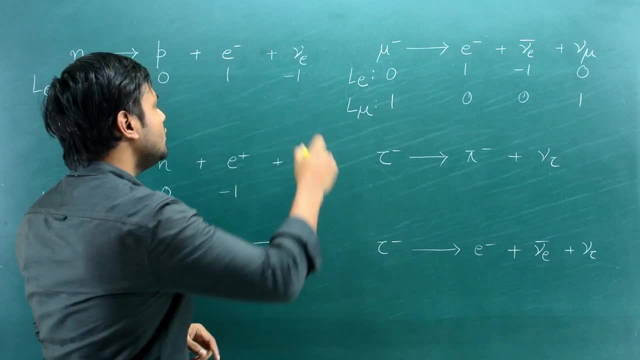 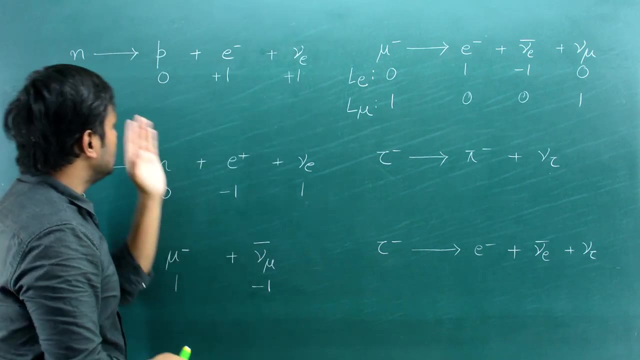 electron neutrino, because if an electron is emitted with an electron neutrino, the lepton number will be plus one and plus one in both cases, left hand side zero, right hand side. plus one plus one equals two violation of the conservation of lepton quantum number. it's not possible. this reaction does not. 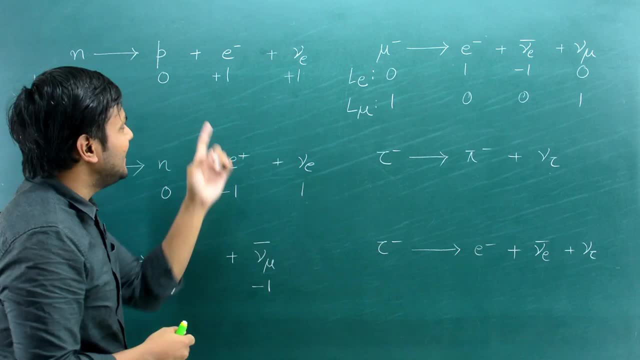 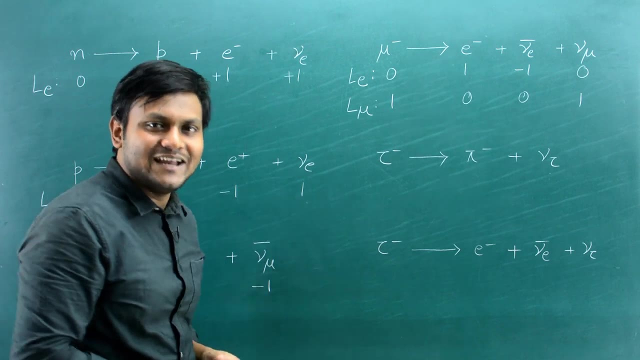 happen. this is not allowed in nature, so electron will never be emitted along with the electron neutrino, but it will only be emitted along with the anti-particle of the electron neutrino. so the anti-particle of the electron neutrino is this, which is a lepton one number of minus one. this 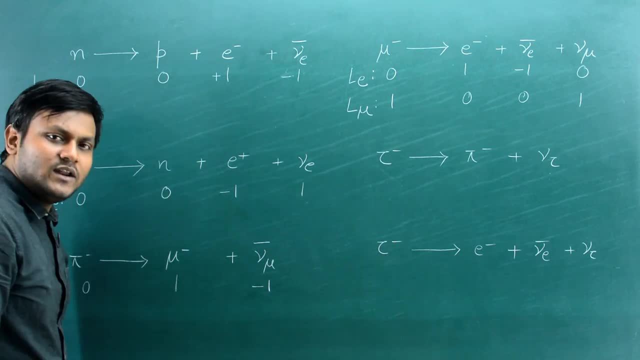 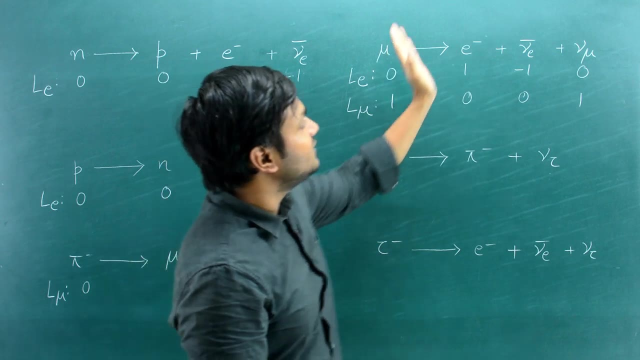 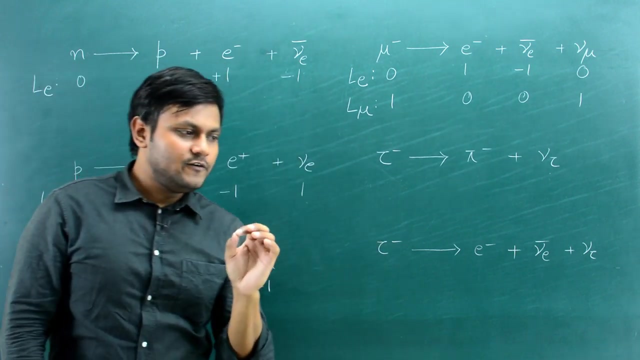 reaction is possible, same for the case of muon and the anti-muon neutrino right and whenever one of these particles, like muons, decay. in that case on the other side you can have a muon neutrino, because in that case the quantum number remains conserved. so i hope that this gives you a little bit of a clue as to 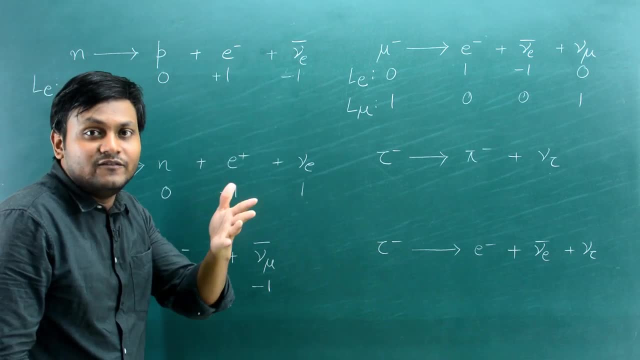 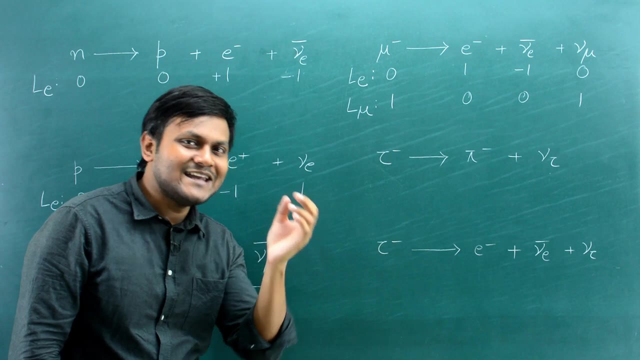 what kind of particles are involved, because as a student, even i got confused in the examination when i used to think, like, okay, with the electron, will the electron neutrino be emitted or the electron anti-neutrino? this is something really confuses you, right? so once you understand this, 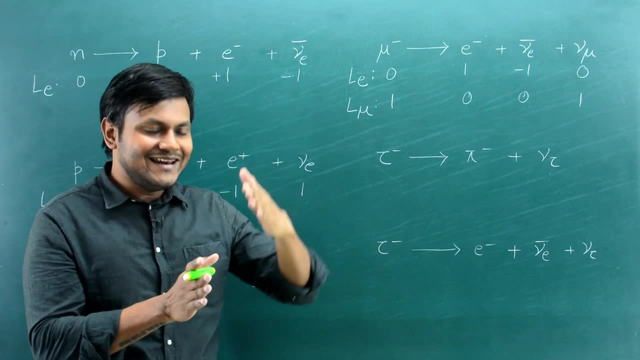 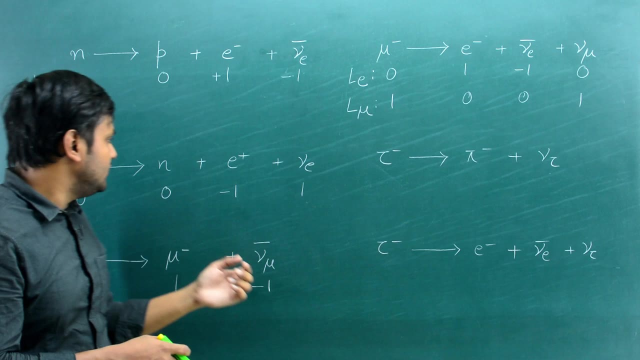 now it makes sense. along with the electron, always an electron neutrino is emitted. along with the muon, always an n muon anti-neutrino is emitted, right. same with the positron. along with the positron, electron neutrinon is emitted, right, let's go ahead. the 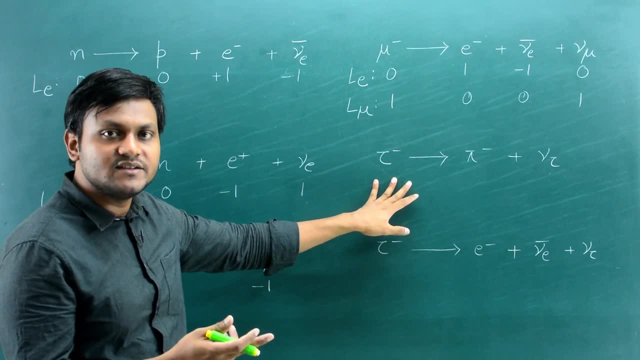 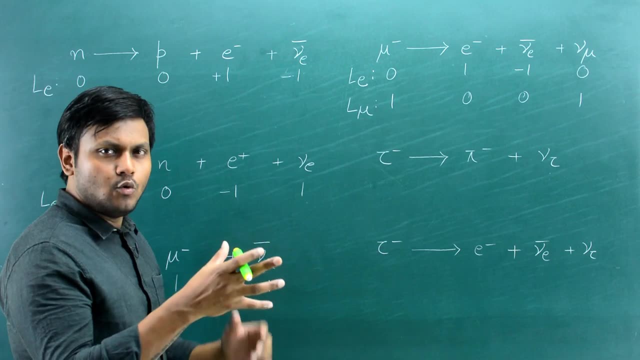 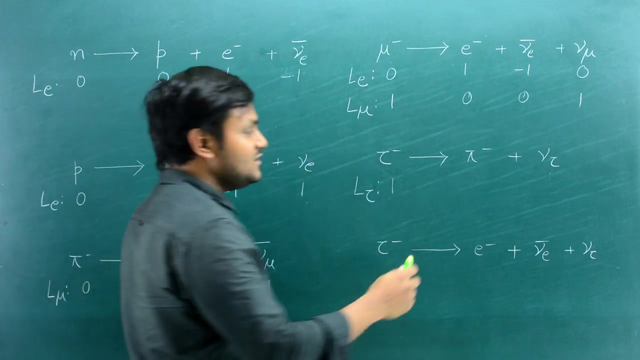 next interaction. the tau particle can decay under certain situations into a pie meson and a tau neutrino, so we will only look at the conservation of the tau lepton number, which is l tau. now, what is l tau for the tau particle? it's one. what is l tau for the pie meson? zero, zero, then that was also. 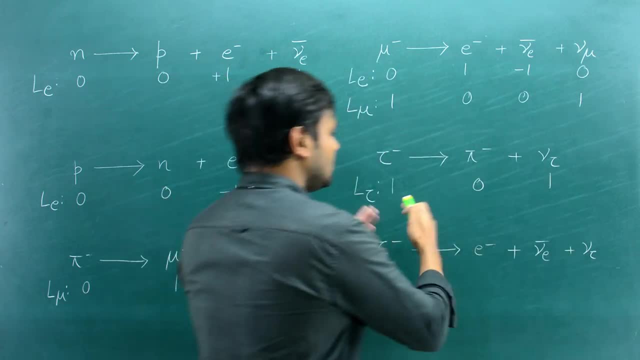 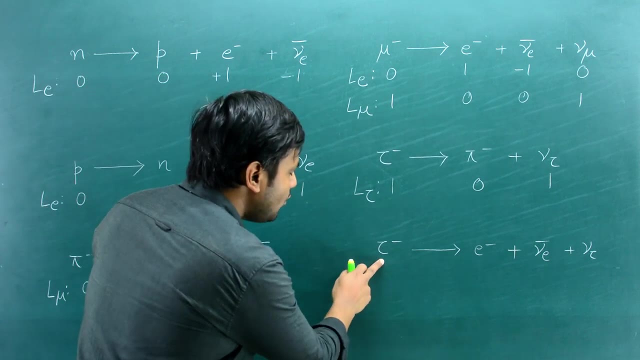 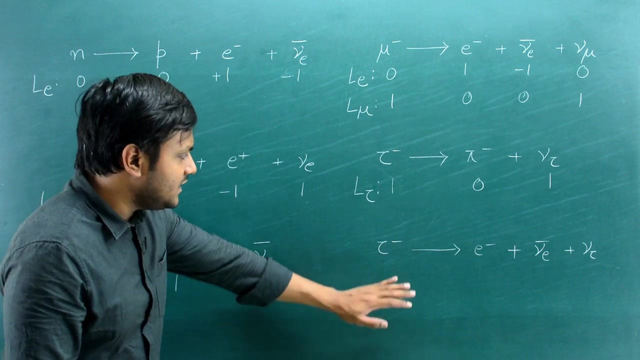 and for the tau neutrino it's: 1. Conserved right Left-hand side 1, right-hand side 1, the tau lepton number is conserved, And the last interaction I have is a tau particle can sometimes also decay into an electron, electron antineutrino and a tau neutrino. Again, here we. 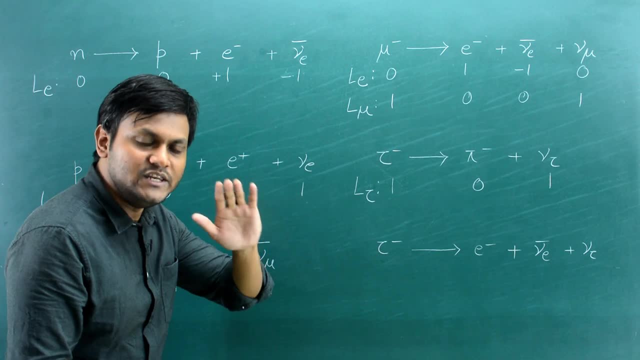 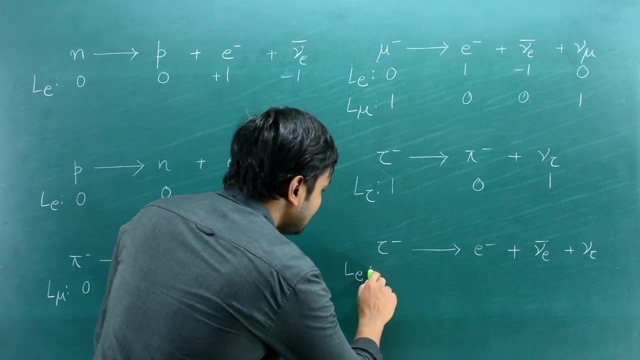 have two family of particles, electrons and the tau particles, right, So we need to check their conservation separately. So first we will look at the electron lepton number, which has a value of 0 for the tau particle, 1 for the electron minus, 1 for the electron antineutrino and 0 for 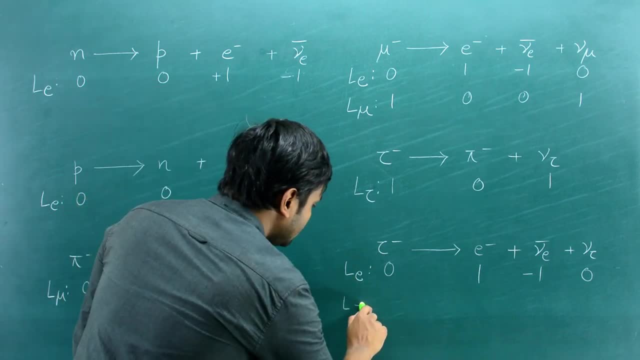 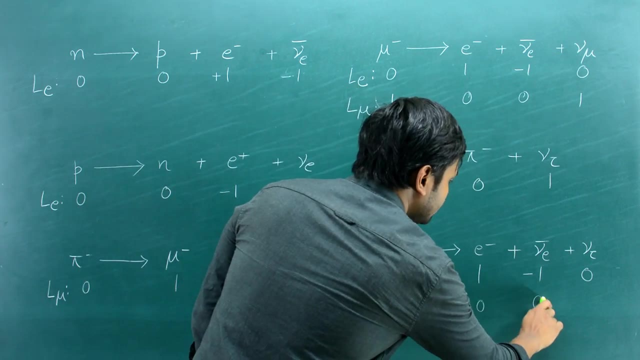 the tau neutrino. And then we have to check for the tau lepton number, which has a value of what? 1 for the tau particle, 0 for the electron, 0 for the electron antineutrino and 1 for the tau. 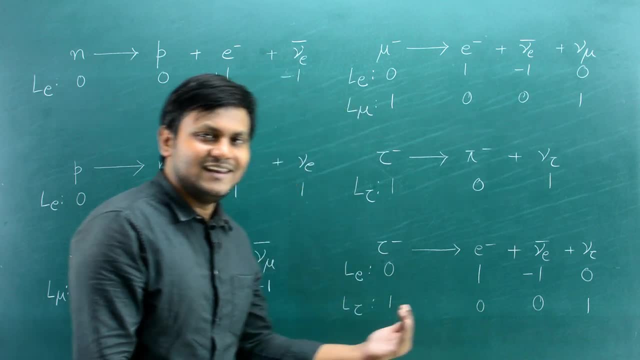 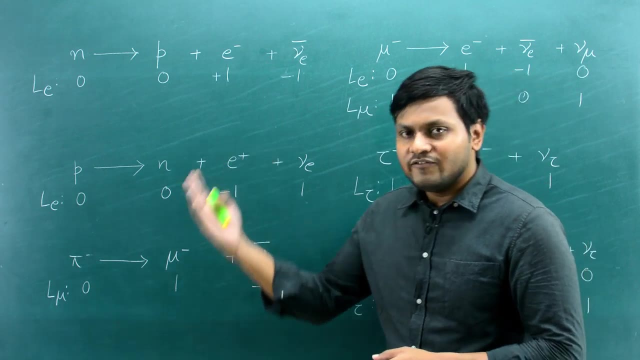 neutrino. Again, as you can see, these numbers are conserved in the left-hand side and the right-hand side. So, as it turns out, when we associate the electron factor with the tau lepton number, we get a value of 0 for the tau particle, 1 for the electron. 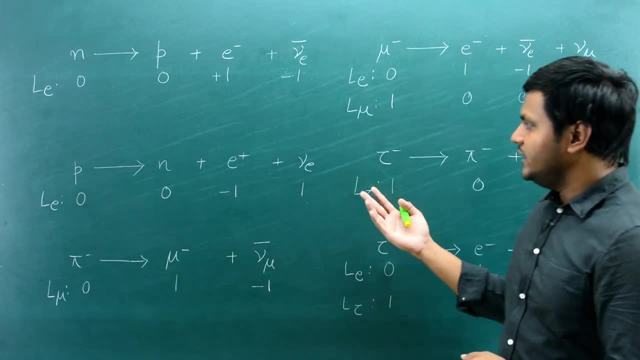 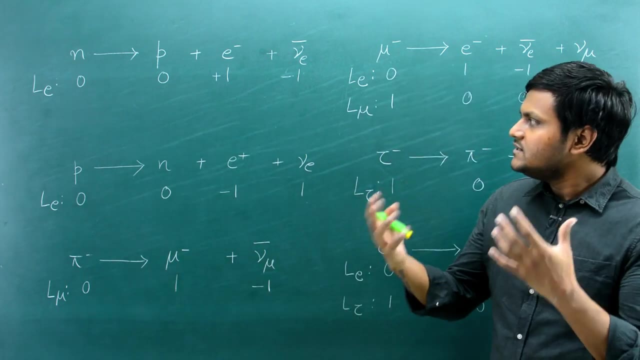 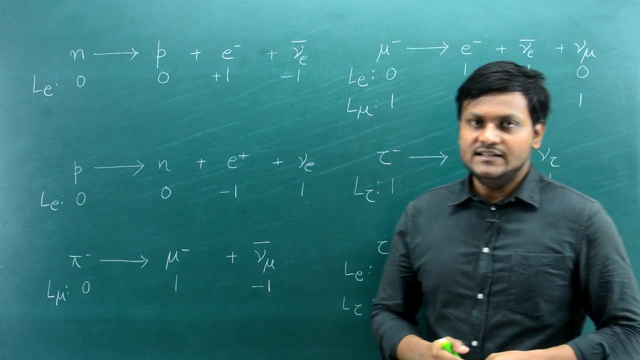 family, the muon family and the tau family, with these distinct lepton numbers, the electron number, the muon number and the tau number, Then it turns out that these quantum numbers are conserved in different kinds of particle interactions involving these particles. So in a way, 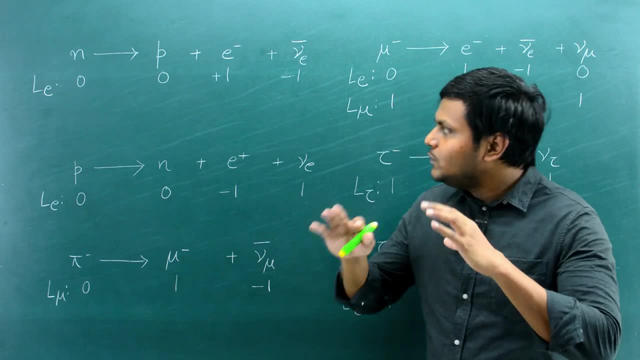 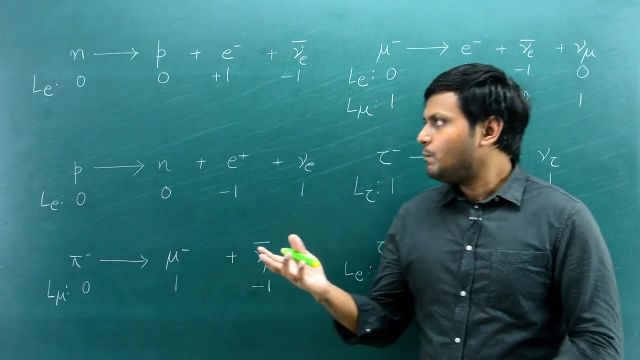 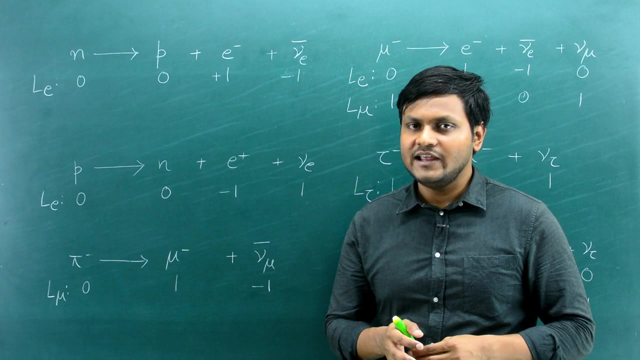 this gives you a set of rules that will help you get an idea about what kind of particle interactions are possible, what kind of particle interactions are not. So lepton quantum number is always conserved, except maybe in neutrino oscillations. So 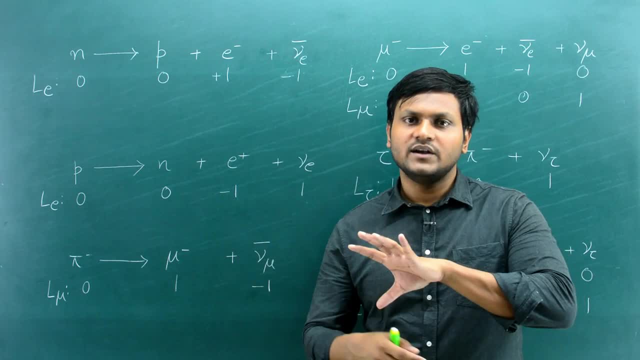 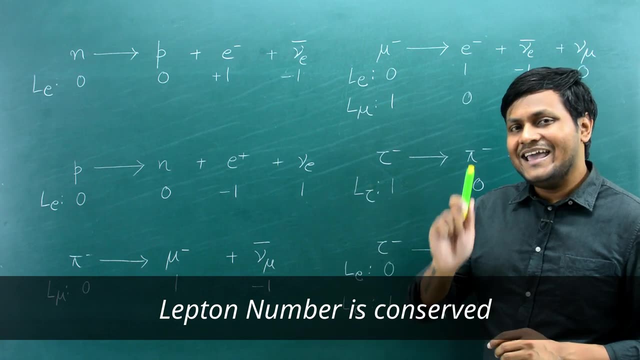 in neutrino oscillations lepton quantum number is not conserved as a particle goes from one point to another, But apart from that, in almost all other particle interactions the lepton quantum number is conserved, So this gives you a very helpful tool in sorting out different kinds of 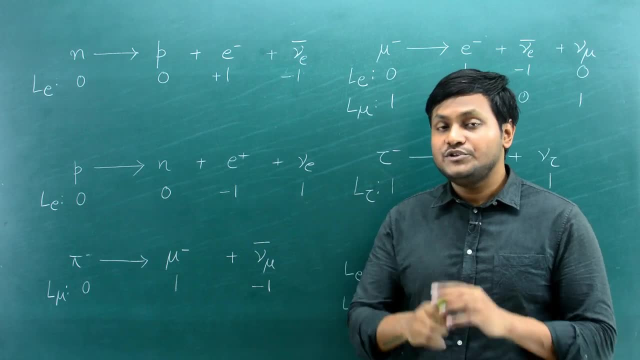 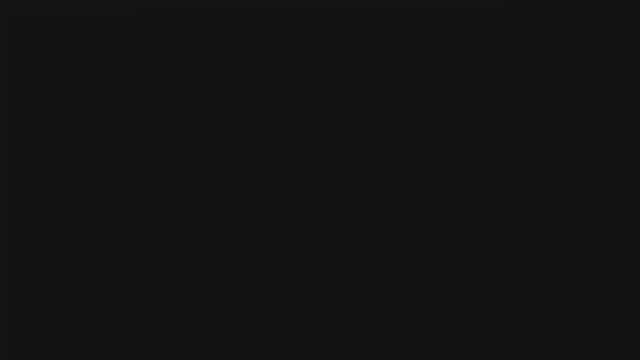 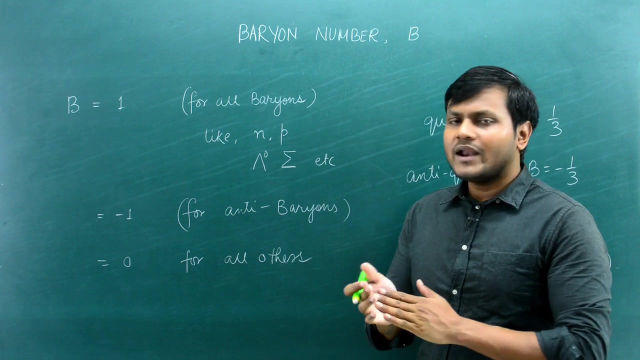 particle interactions. Now let's move ahead to the next quantum number, which is the baryon quantum number. So the baryon particles are essentially particles that consist of three quarks. Now remember I talked about leptons as those elementary particles that do not. 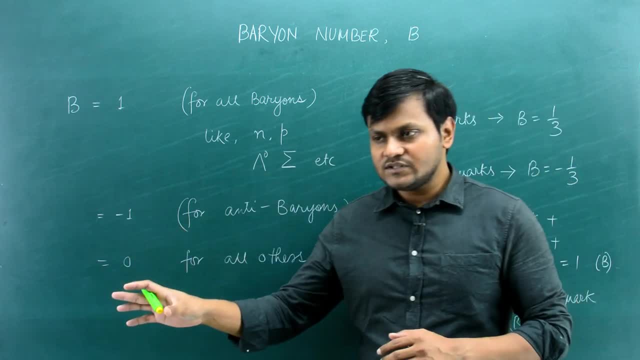 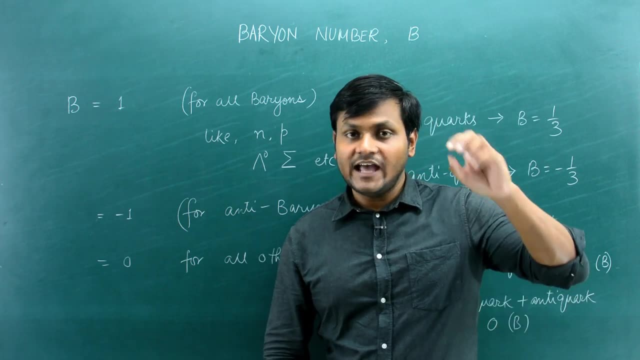 experience a strong force. Now, as opposed to leptons, there is a class of particles called hadrons, which are particles that do experience a strong force, And the hadrons can be further classified into what are called baryon particles. So baryon particles are essentially particles that 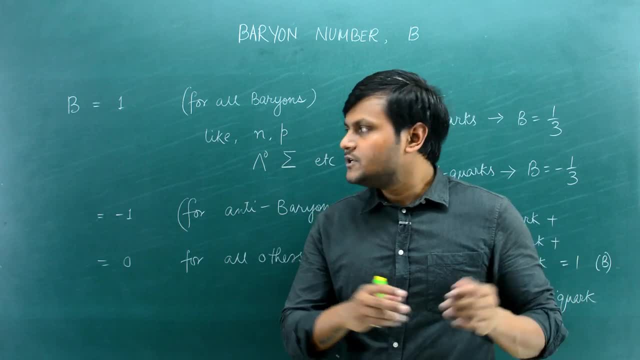 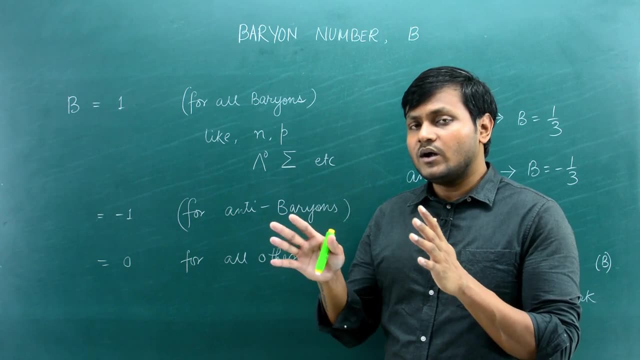 what is called baryon particles and meson particles. So baryons and these meson particles belong to a category called hadrons. I have talked in detail about these particles in one of my earlier videos. If you're interested, you can check that out. So, as it turns out, these baryon 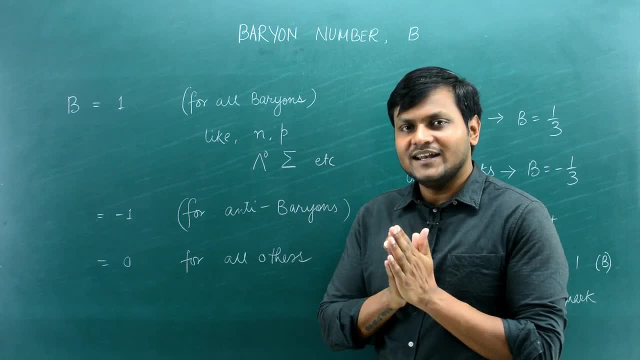 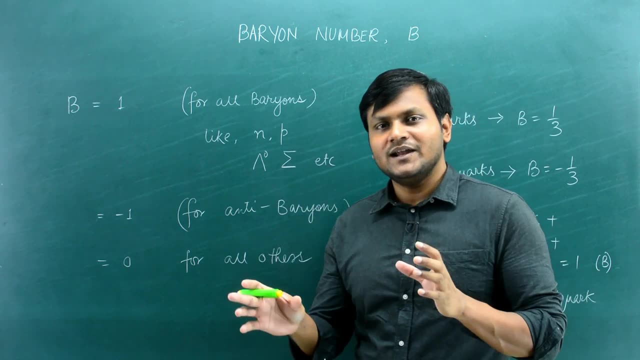 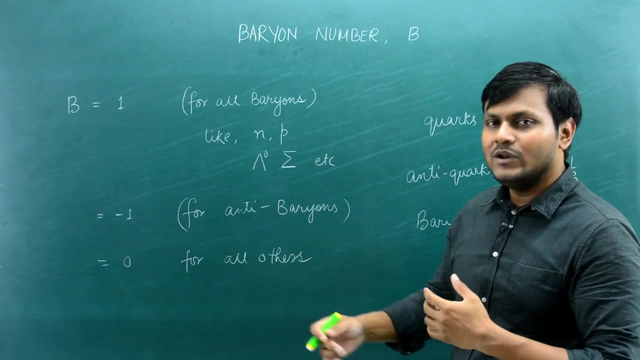 particles. whenever they are involved in some kind of a particle interaction, then we can associate a similar kind of a number with them, such that that particular number, its summation, remains valid whenever particle interactions happen. So a very simple rule is as follows: So all. 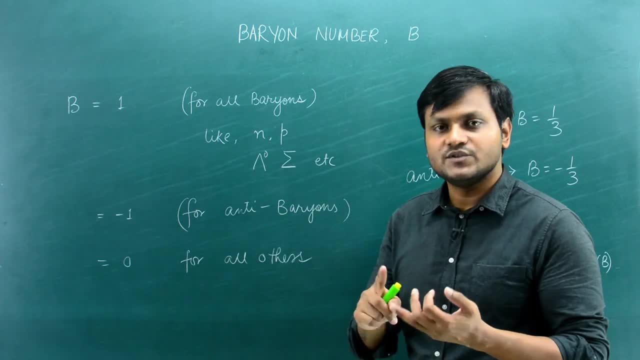 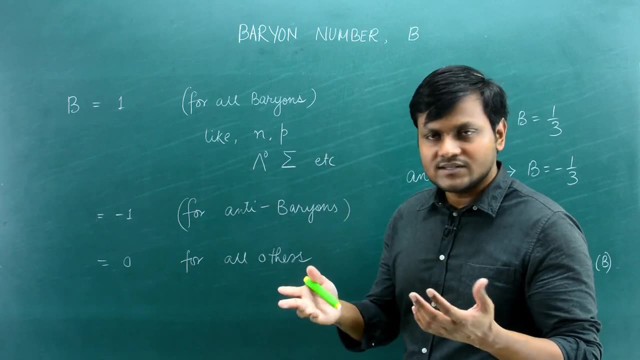 baryons. so baryons are basically like neutrons, protons, lambda particles, omega particles, sigma particles, xi particles, etc. So it consists of the nucleon particles as well as the hyperon particles, which consists of three quarks essentially. They do not include the mesons. 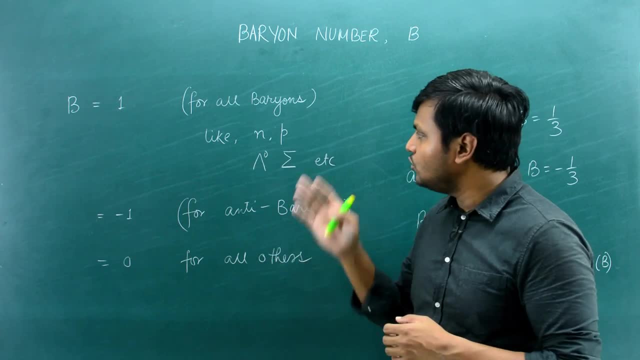 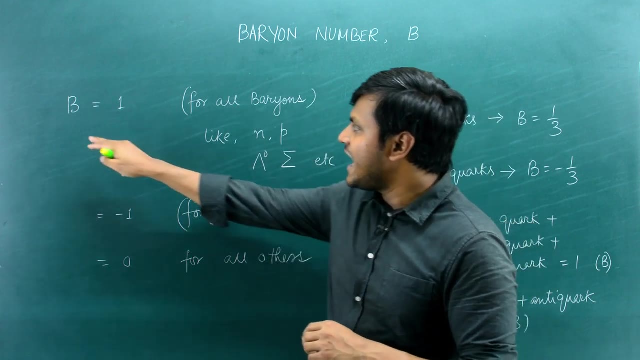 Mesons basically have two quarks in them, So they do not include the mesons. They only include the baryons, which basically include three quarks. So all the baryons have a number of equal to one that we can associate with them. This is called. 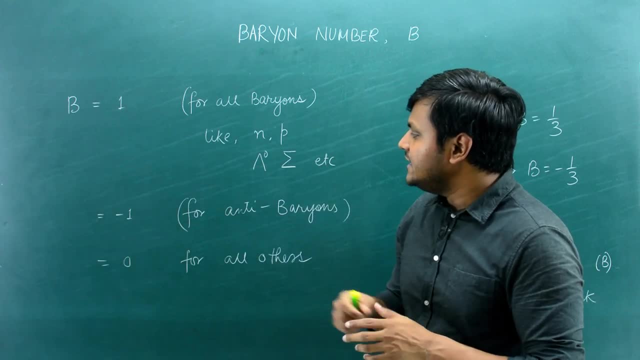 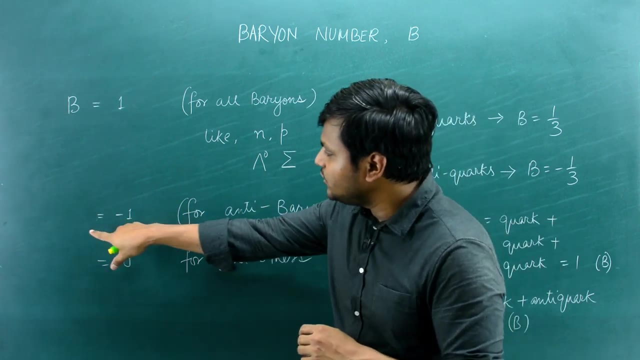 the baryon number represented by the capital B, And the antibaryons, like the antineutron, the antiproton, as well as the antiparticle version of the rest, can be associated with a number of minus one, while the rest of the particles can be associated with zero, So plus. 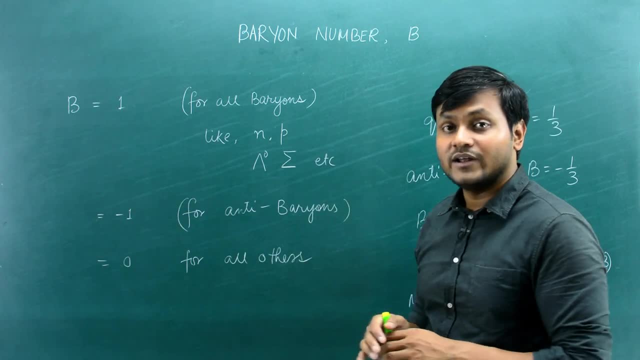 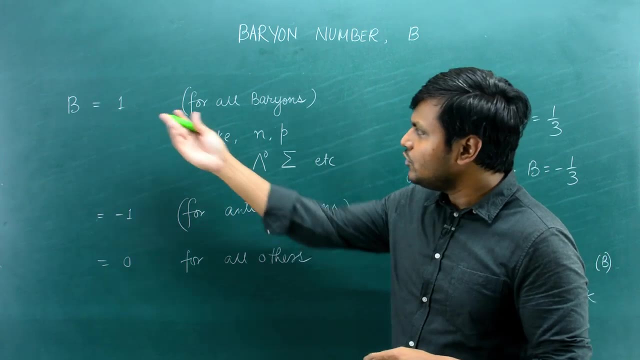 one minus one and zero for the baryons, antibaryons, and for the rest we can associate with these and look at their conservation in different particle interactions. So the baryon number essentially of one basically comes out as a result of the quarks. okay, So we can also say: 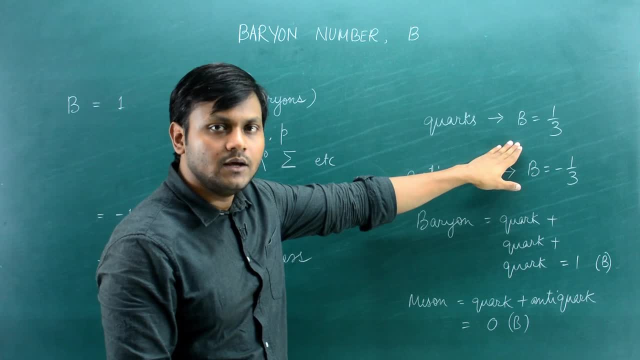 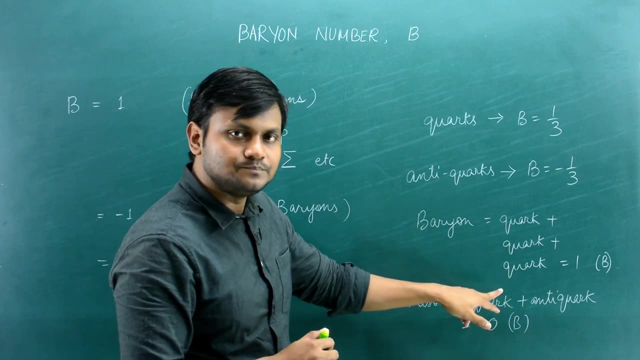 that the quarks have a baryon number of one by three, while the antiquarks have a baryon number of minus one by three. okay, So because baryons are made up of three quarks, so one by three plus. 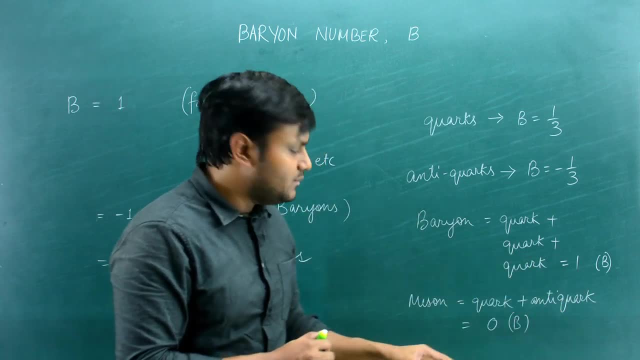 one by three plus one by three come out to be equal to one, while mesons, on the other hand, are made up of a quark antiquark. So, baryon, number of one by three minus one by three minus one by three. 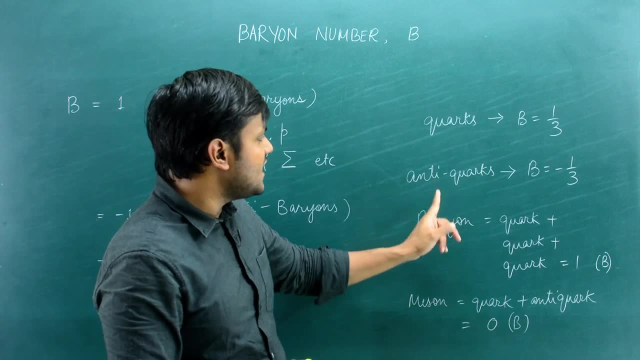 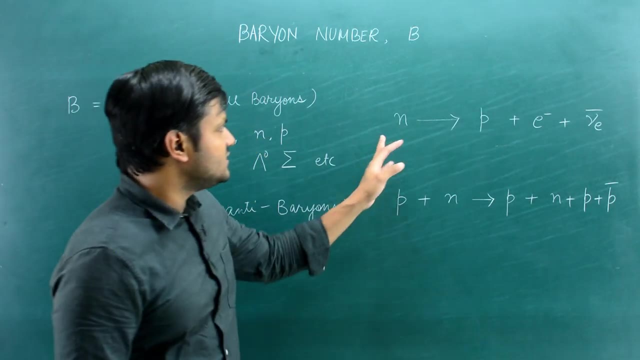 comes out to be zero. So mesons have a baryon number of zero, baryons have a baryon number of plus one. Let's look at a few interactions. okay, So here again I have this interaction which is: 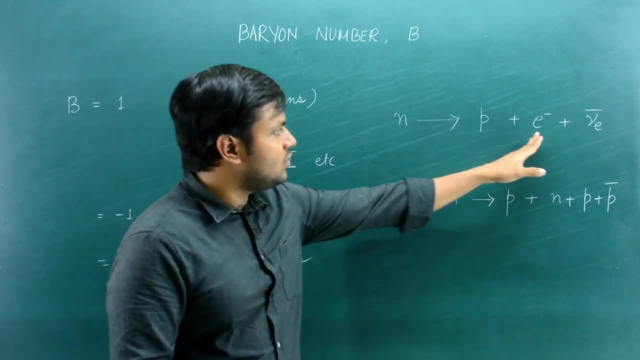 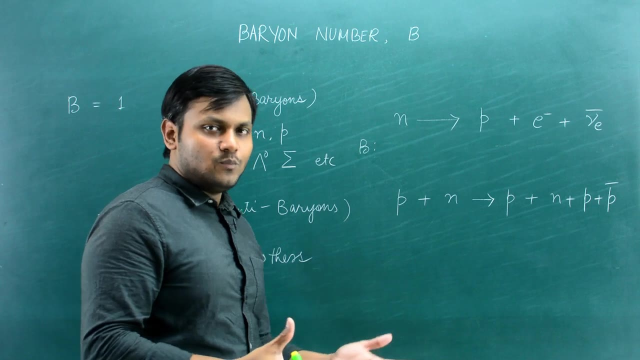 the beta decay interaction. So a neutron becomes a proton, leads to the emission from electron and electron antineutrino. So if I look at the baryon number here, so the neutron and a proton are baryon particles, so they have a value of one each. all right, The other two have a value of zero. 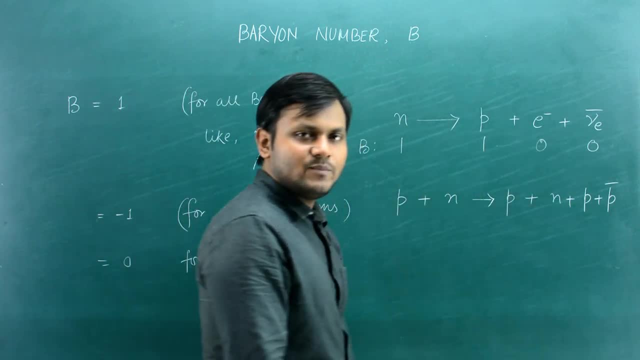 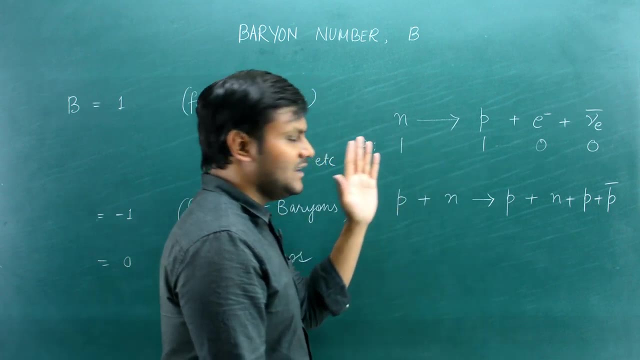 So, as you can see, the left-hand side is a baryon number one. right-hand side is a baryon number of one, So this number remains conserved right. So if there's a baryon particle on the left-hand side, there must be a baryon particle. 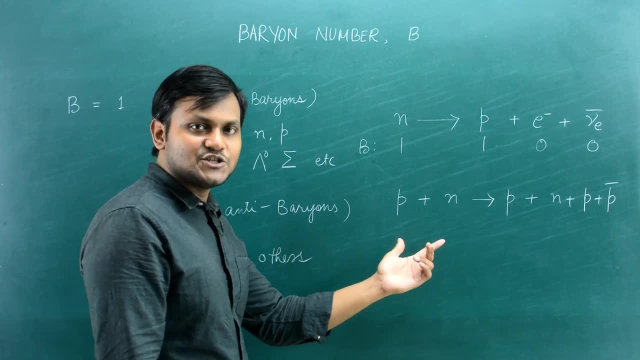 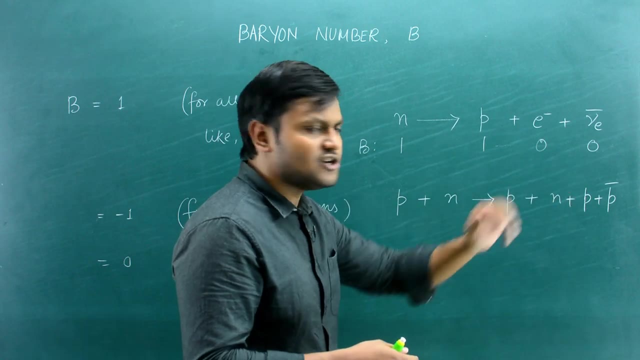 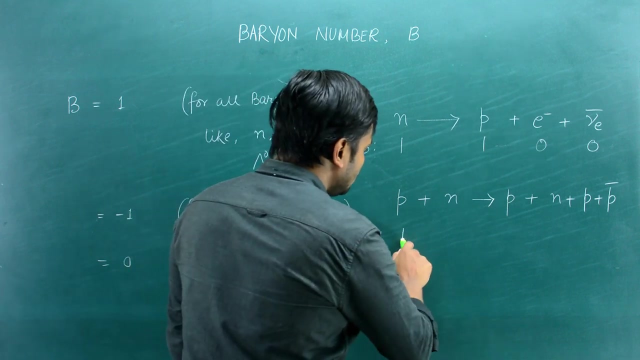 on the right-hand side. In certain kinds of high energetic reactions, a proton and a neutron may collide under extreme energy and lead to the creation of new particles like this. So let's look at this kind of a reaction. So the baryon number for a proton and neutron is equal to one. 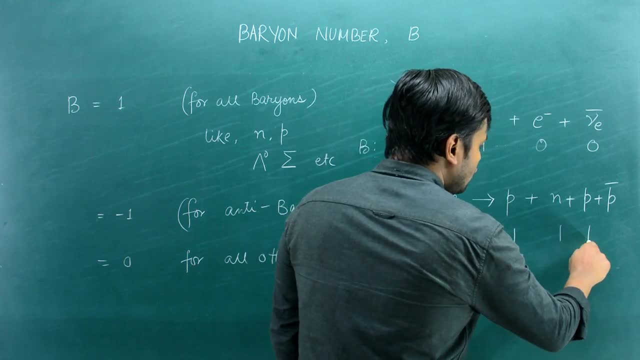 right. So let's look at this kind of a reaction. So the baryon number for a proton and a neutron is equal to one. right On the right-hand side you have a proton and a neutron and a proton and an antiproton. 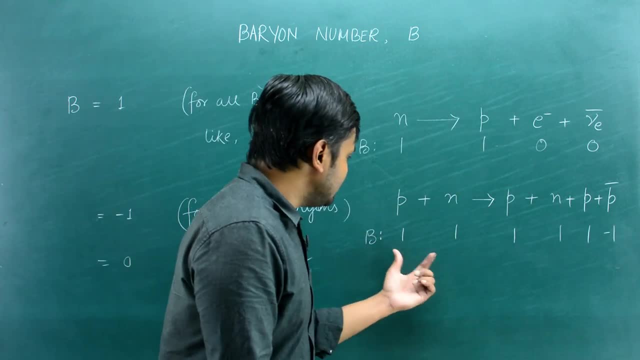 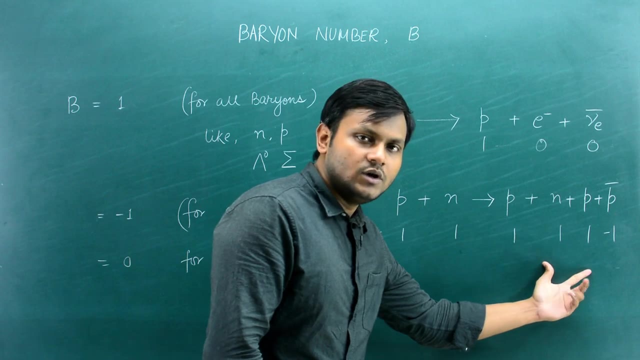 which has a value of minus one. So what is the value of baryon number? left-hand side? One plus one, two. On the right-hand side you have one plus one plus one, three minus one, two, So two, two. That means this number is conserved in this kind of a particle. 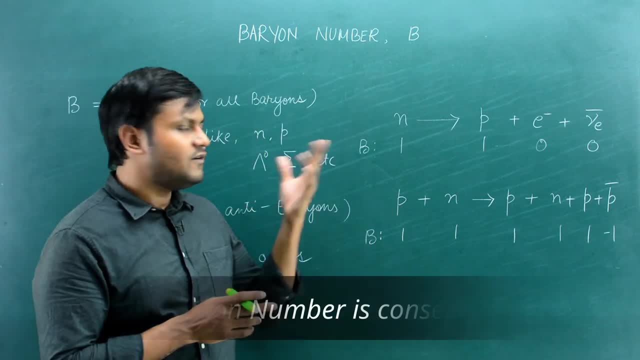 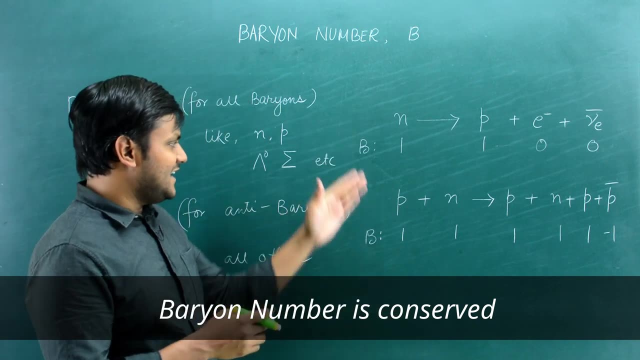 interaction. Now, as it turns out, baryon number is a kind of a quantum number that is conserved in different kinds of particle interactions. So getting an idea about this number will give you an idea about which of the reactions are possible, or 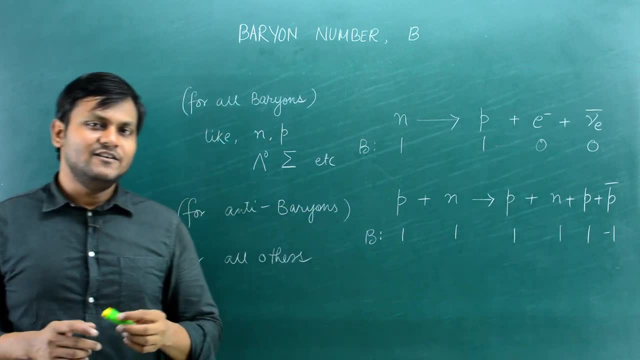 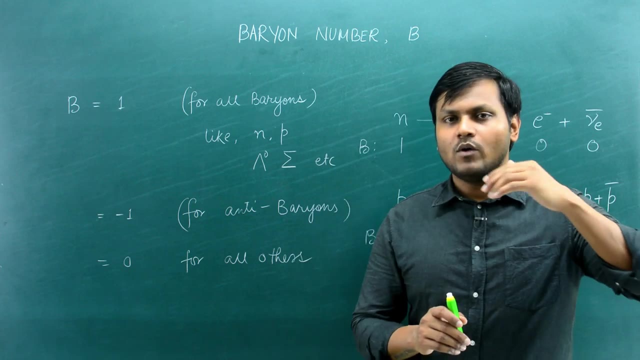 not possible whenever baryon particles are involved. And last but not the least, there is another quantum number, which is known as the strangeness quantum number. This is called strangeness quantum number because it is associated with particles that has a different kind of a. 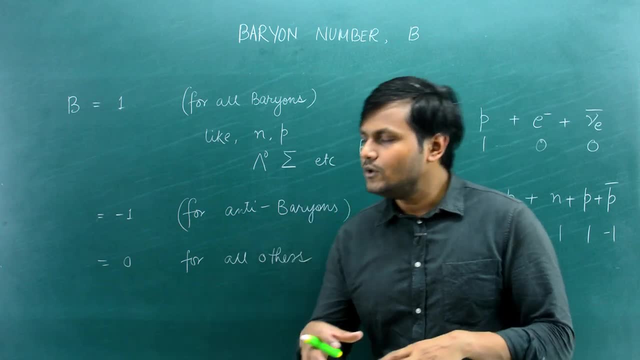 what you can say strange behavior. So scientists, when they were looking at different kinds of interactions in the last hundred years, they were looking for a different kind of behavior. So scientists, when they were looking at different kinds of interactions in the last hundred years, around 1950s or 60s, they found that there is a large number of particles which were created that behaved in a very strange manner, that were produced by either strong or electromagnetic interaction, but that decayed via weak interaction. And those particles 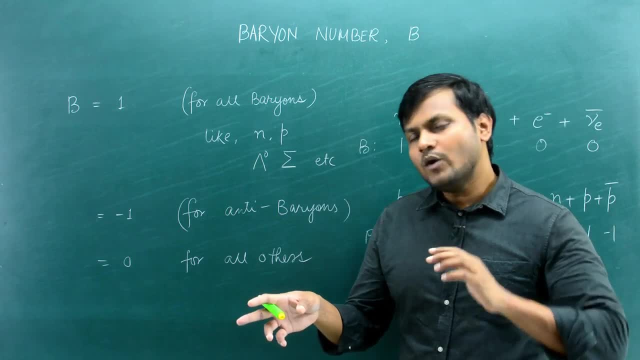 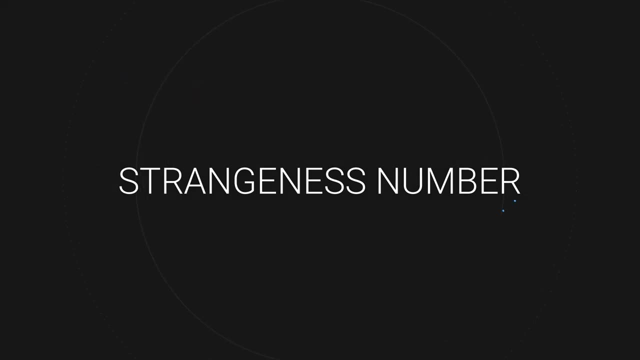 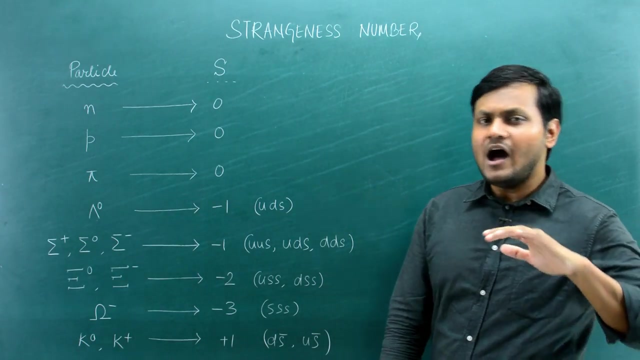 scientists named as strange particles, And there is a quantum number associated with those particles also, which is known as the strangeness quantum number. So what are the causes of strangeness quantum number? Okay, so almost half a century ago, scientists were studying the creation of newer and newer. 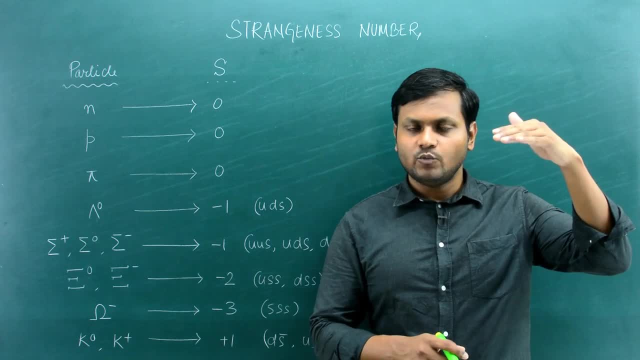 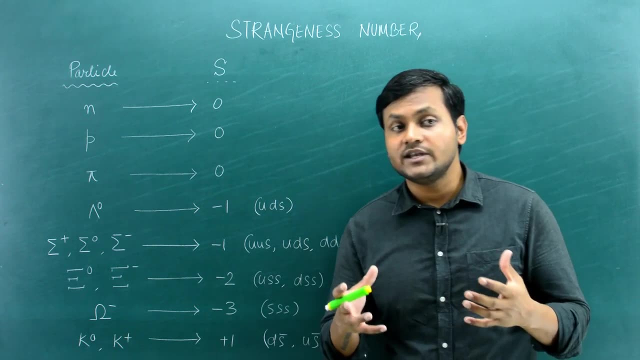 particles right. So whenever you look at cosmic rays, when they enter the earth's atmosphere, it leads to the creation of a large number of subatomic particles. Or whenever you study high energetic particle interactions in particle accelerators, you end up getting 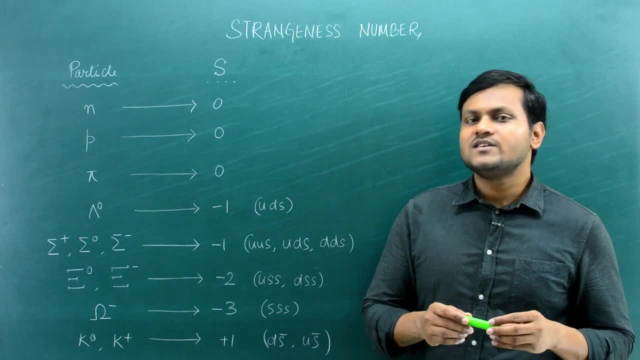 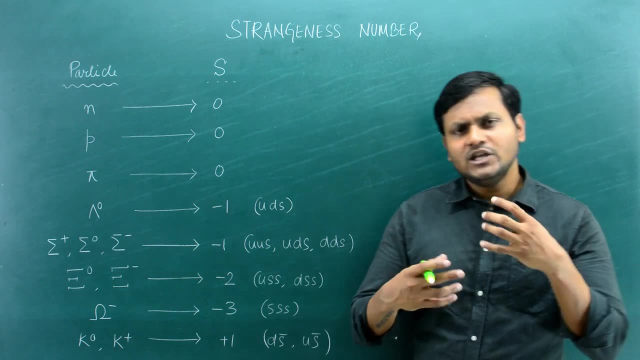 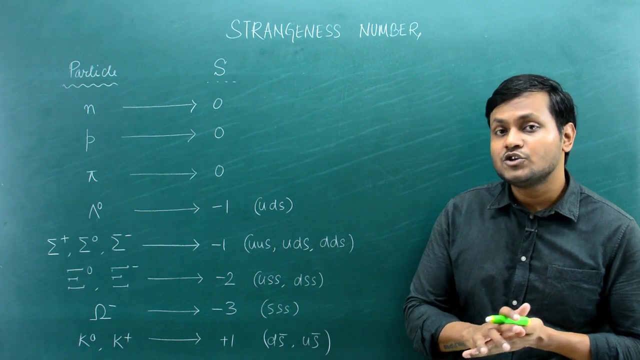 newer and newer particles. So when scientists were studying the byproducts of extremely high energetic particle interactions, then they found out that newer and newer particles were being created that behaved in a very strange manner. That is why this number is called strangeness number, So they behave in a strange manner in this particular way. They were created via. 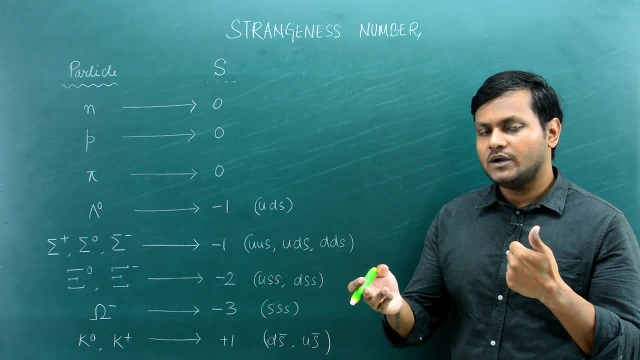 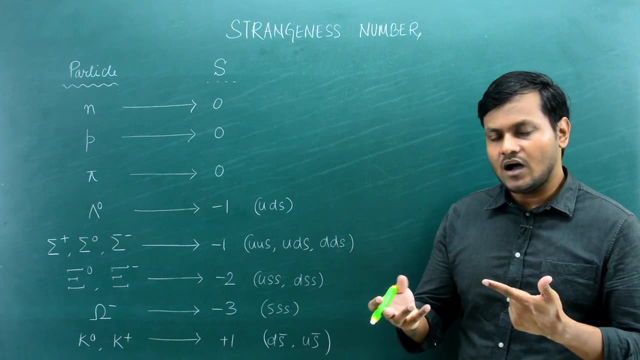 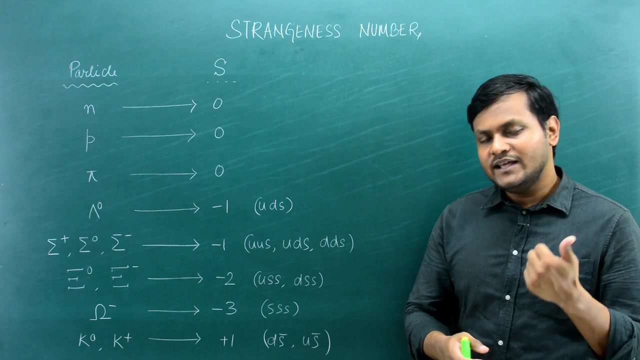 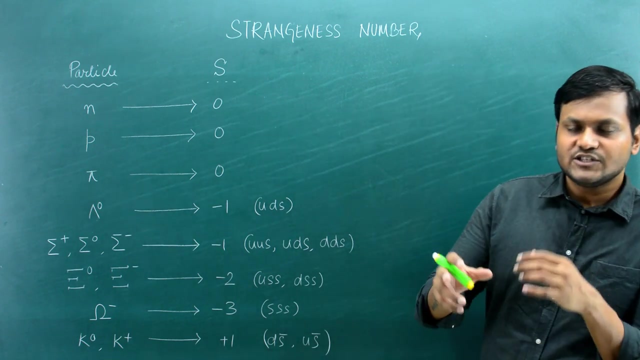 electromagnetic or strong interaction, but after they were created they decayed via weak interaction. So these strange particles are subatomic particles which are created via strong interaction or electromagnetic interaction, but they decay via weak interaction. Now, as it turns out, when we study these kind of strange particles, we can associate: 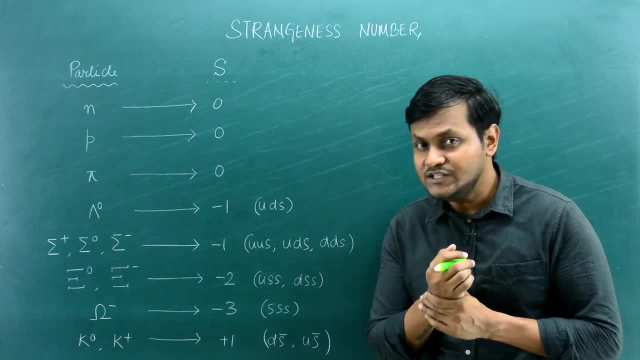 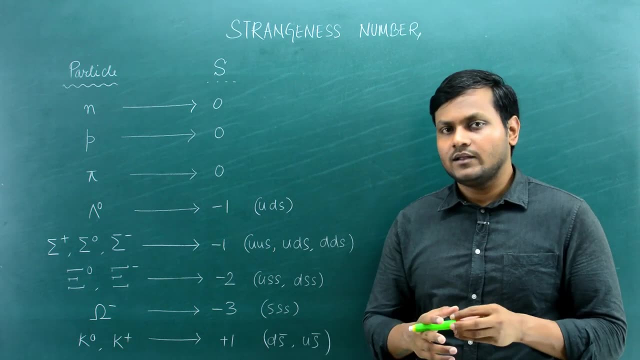 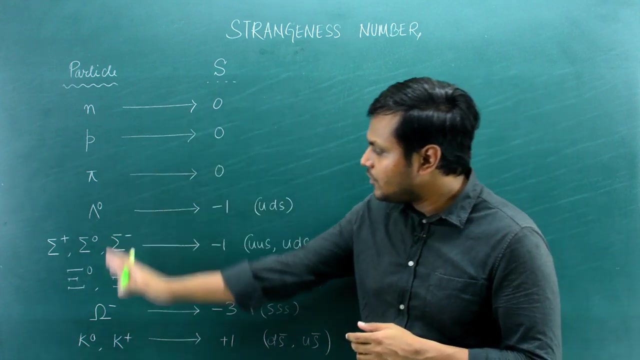 a quantum number- known as a strangeness quantum number- with these particles that remain conserved, at least in their creation, if not in their decay. So before I talk about the interactions, especially, let's look at different kinds of particles. So here I have a bunch of what is called hadron particles. So essentially, 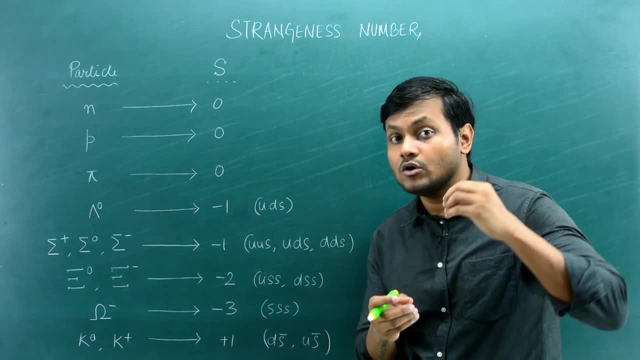 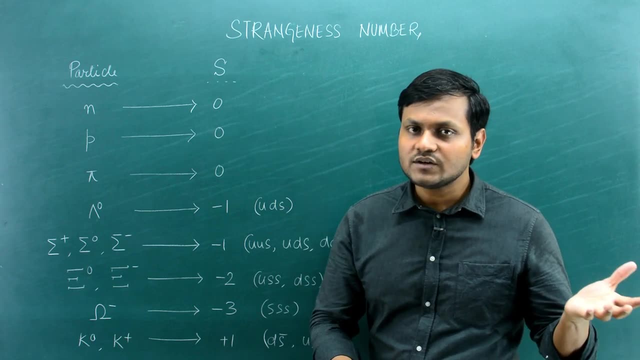 the strangeness: quantum number is a result of the strange quark. So you see, the hadron particles are made up of quarks, mesons are made up of two quarks, baryons are made up of three quarks and 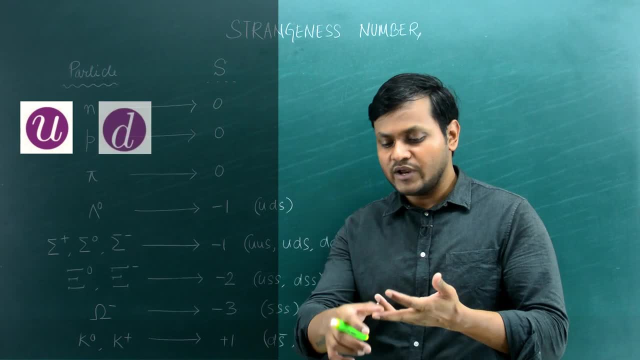 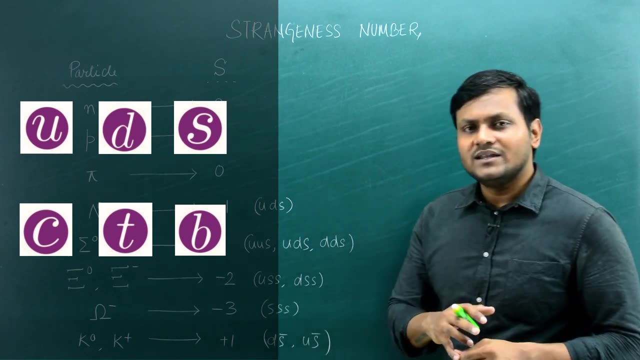 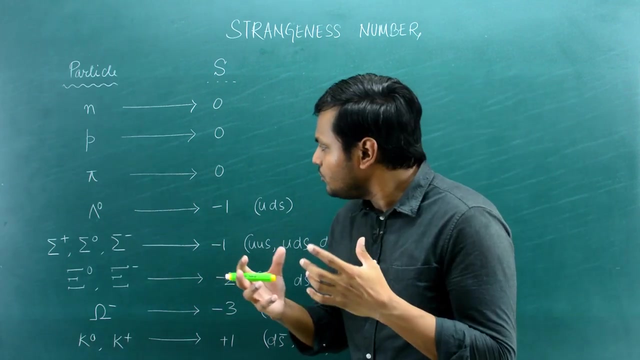 there are different kinds of quarks. You have up quark, down quark, strange quark, charm quark, top quark and bottom quark. So the strange behavior of these particles are essentially for those particles that contain what is known as the strange quark, So hadron particles that do not contain the strange quark. 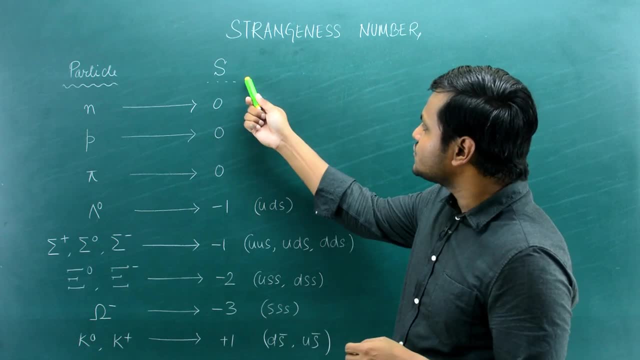 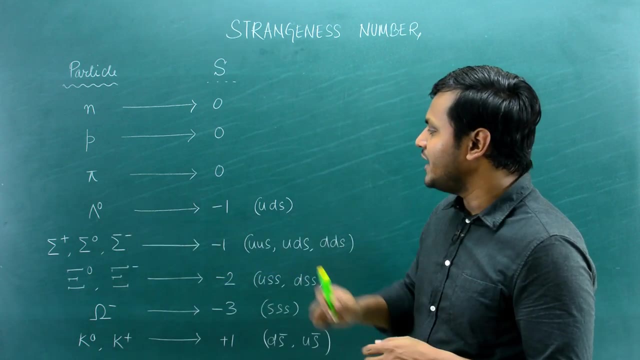 like neutron, proton and timezon, they have a strangeness number of zero. But let's look at the lambda particle. So lambda particle has a strangeness number of minus one. This is because its configuration has one up quark, one down quark and one. 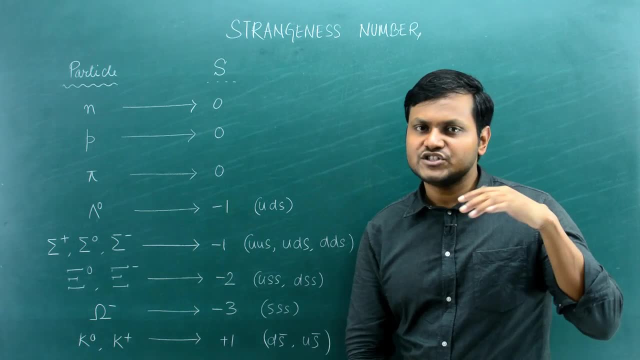 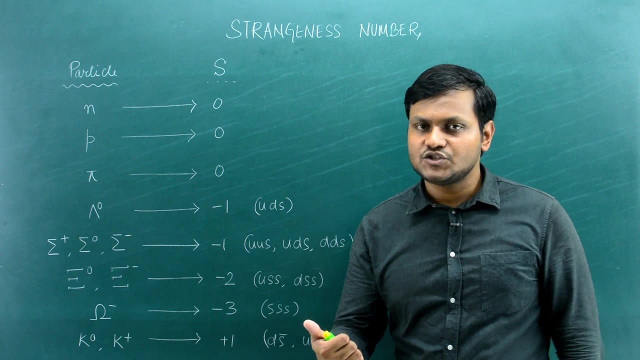 so essentially all the quarks have a strangeness number. This is what a strange quark has: a strangeness number of minus one. the rest of the quarks has a strangeness number of zero. okay, So the strangeness number is associated with the strange quark. 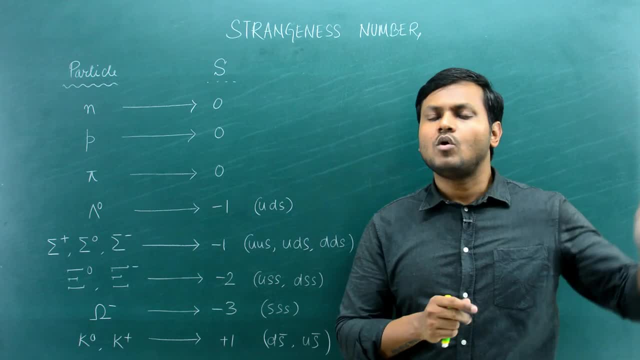 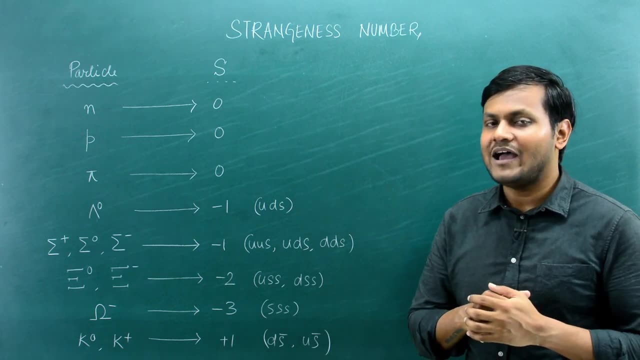 which has a value of minus one. the other quarks has a strangeness number of zero And, on the other hand, the anti-particle for the strange quark has a value of plus one. okay, So whenever you have hadron particles created by the strange quark, you end up getting some kind of a. 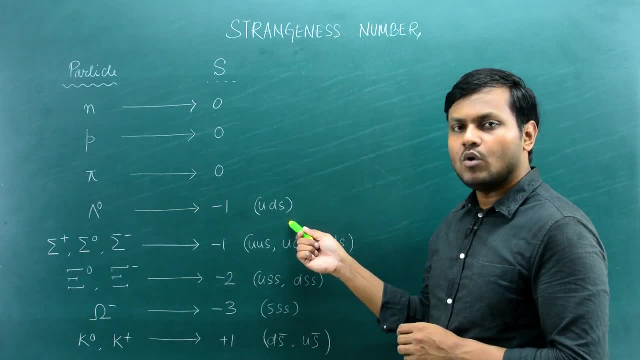 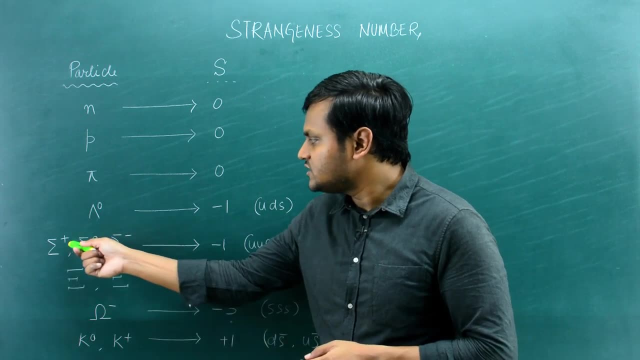 strangeness number. so lambda particle which contains one strange quark has a strangeness number of minus one. similarly you can have sigma particle, sigma plus, sigma zero, sigma minus. so superscript basically tells us about the charge. it also has a strangeness number of minus one. 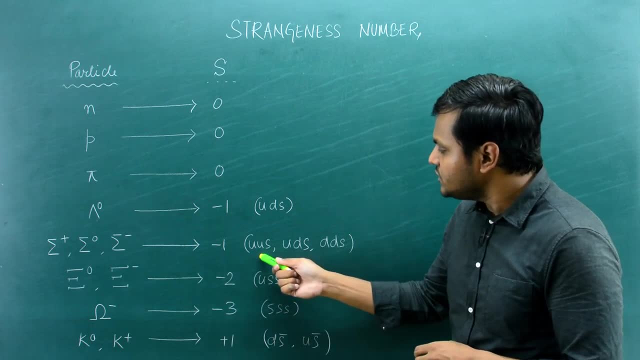 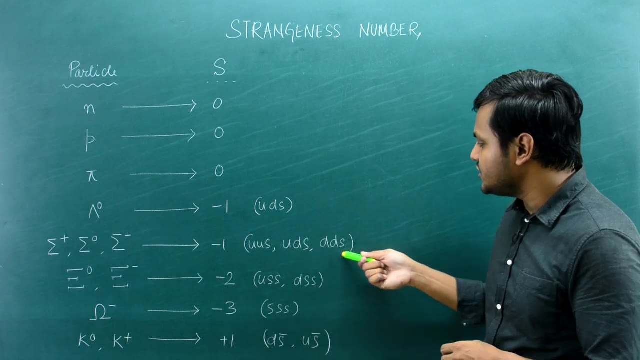 because, if you look at their configuration, they contain one strange quark each. okay, so this is the configuration for sigma plus, this is the configuration for sigma zero and this is the configuration for sigma minus one. now, if you look at the xi particles, xi zero and xi minus one, 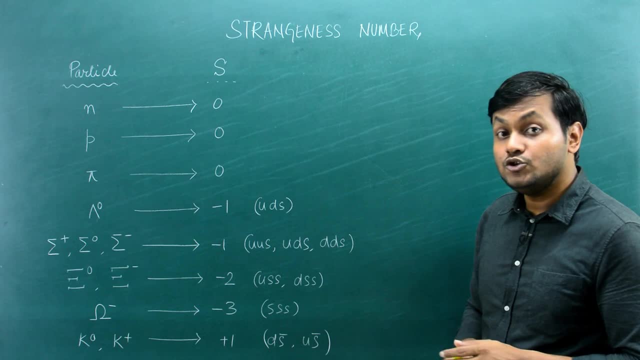 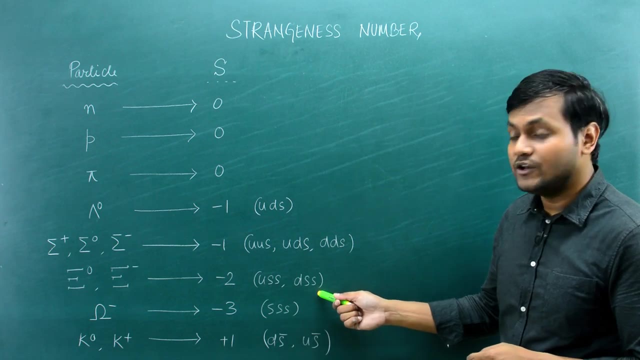 they have a strangeness number of minus two because they contain two strange quarks. the xi zero has up quark and two strange quark and the xi minus has one down quark and two strange quark. so it has a strangeness number of minus two. and on the other hand, the omega particle, which contains 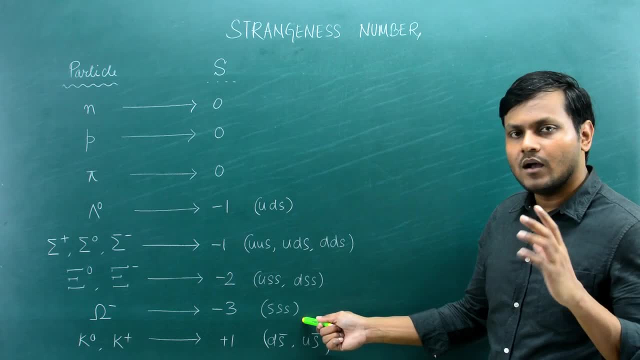 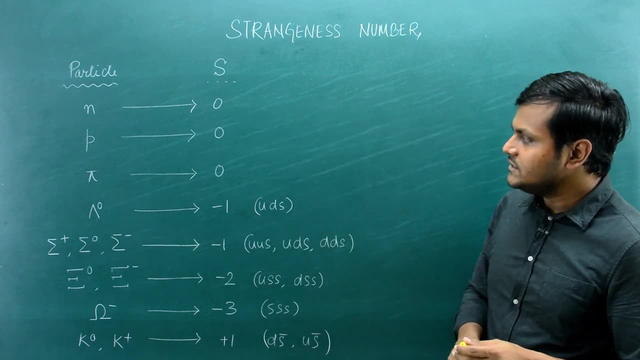 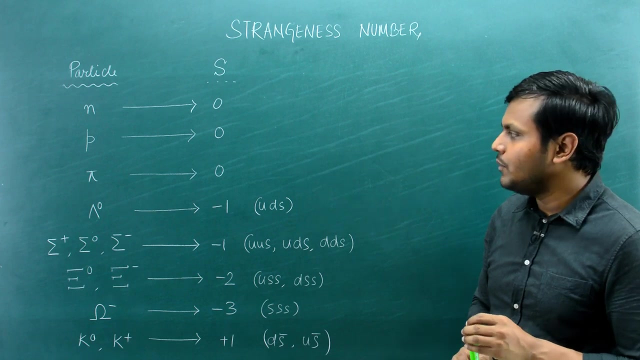 three strange quarks. so the omega minus is composed of three strange quarks, has a strangeness number of minus three. Now, apart from these baryon particles, the pi meson, as well as other meson particles, can also have a strangeness number. The pi meson is not made up of a strange quark, so it has zero. But what about k-on? 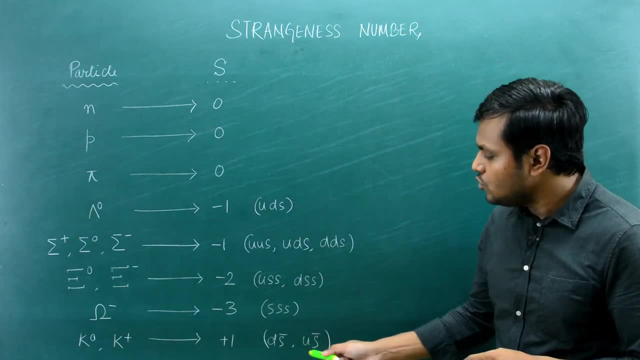 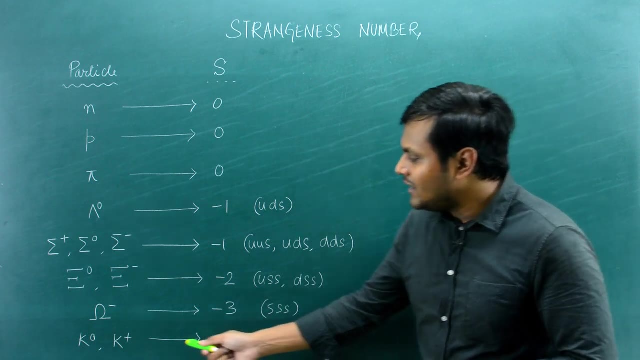 particles. k-on particles are mesons. that means they are made up of two quarks. So k0 is made up of one down quark and one anti-strange quark, while k plus has one up quark and one anti-strange. 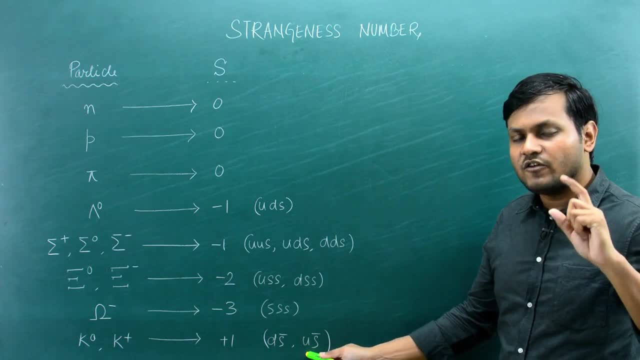 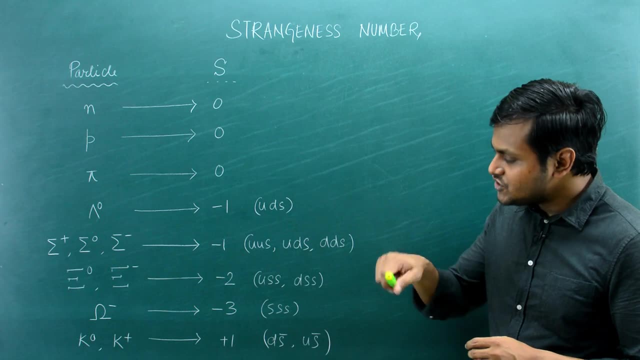 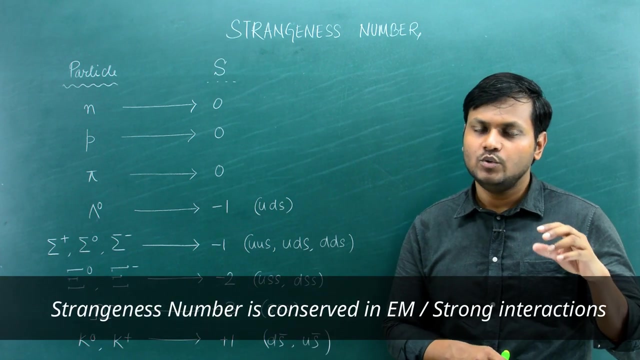 quark. So the anti-strange quark has a strangeness number of plus one. So these two particles have a strangeness number of plus one. On the other hand, k minus will have a strangeness number of minus one. So the strangeness quantum number is conserved only in those cases which involve. 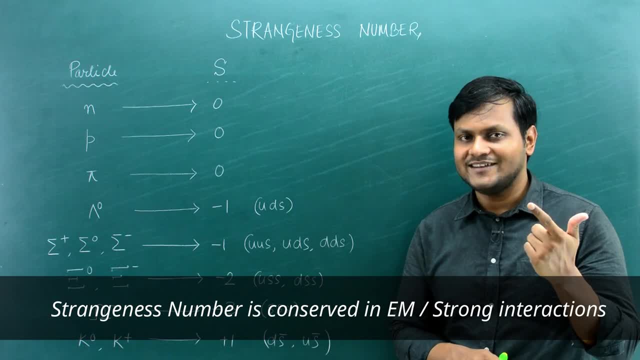 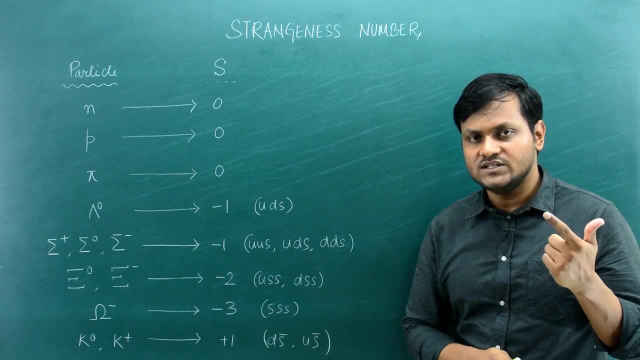 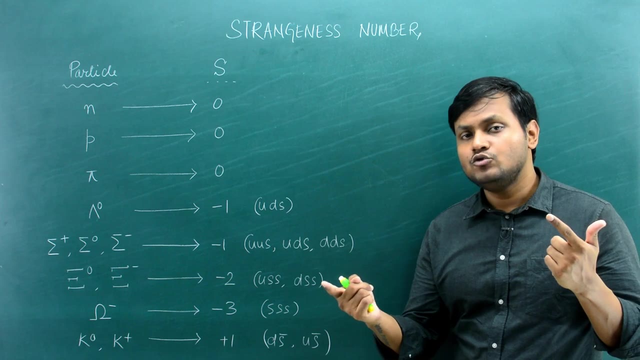 either the electromagnetic ray interaction or the strong interaction, So interactions which involve electromagnetic force or the strong force, only in those cases the strangeness number is conserved. But whenever we look at decay processes where the particle may decay into further particles, in those cases where a weak interaction is involved, 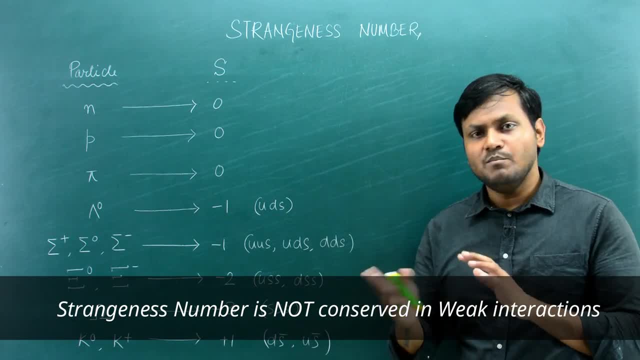 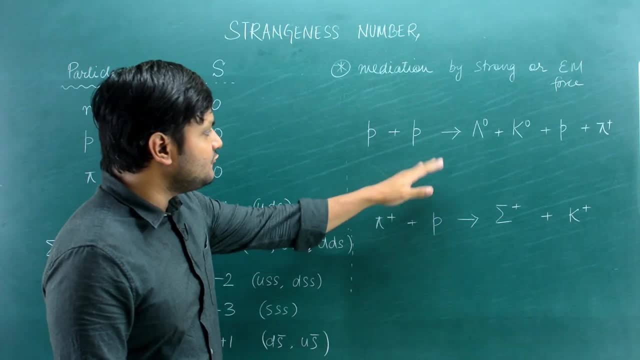 the strangeness number is not conserved. It may change if it involves the weak interaction. So let's look at a few examples. So, for example, here I have two interactions that involve a mediation by either a strong force or an electromagnetic force. So in these cases, 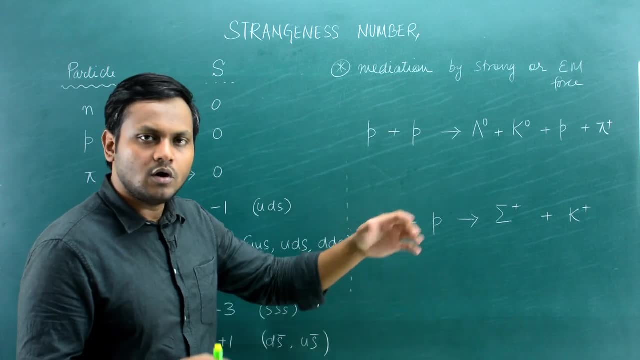 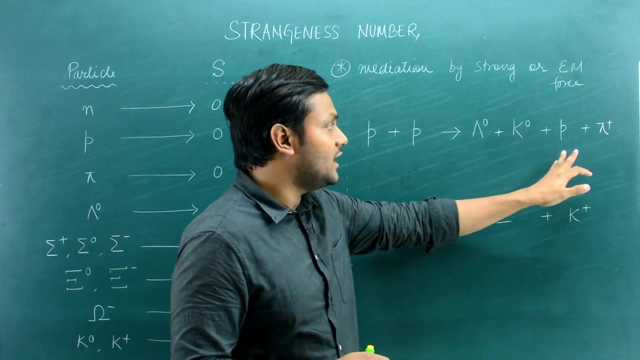 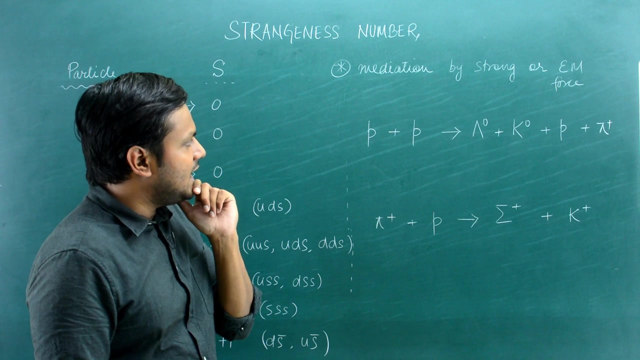 the strangeness number is conserved. So a proton and a proton may collide in particle accelerators to create further particles Like, let's suppose, a lambda naught k0 particle and a proton and an anti-Pyme zone. So if this kind of an interaction is happening, let's say we want to check for the 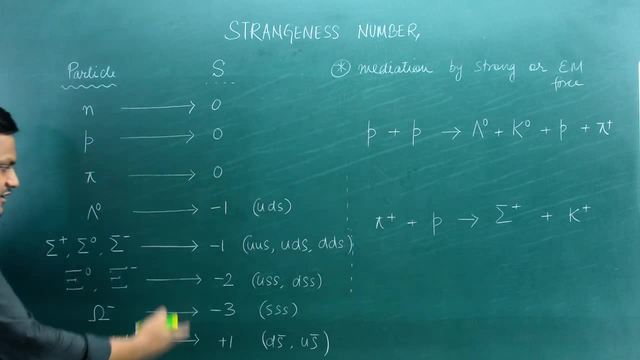 conservation of strangeness number. So we can apply these numbers that I've associated with these different particles. So we can apply these numbers that I've associated with these different particles. So we can apply these numbers that I've associated with these different particles. 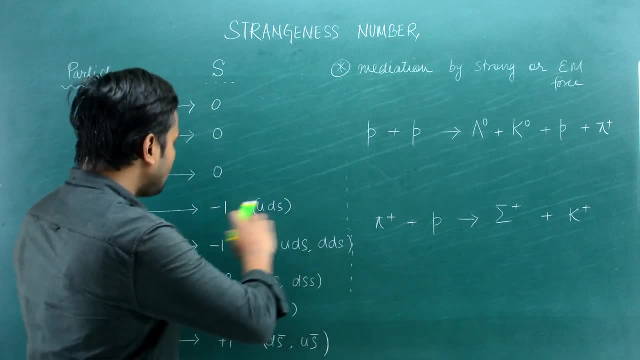 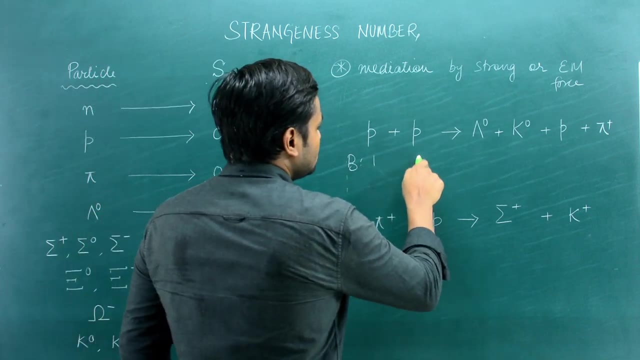 and put the values there to see what's going to happen. Now, before I apply the strangeness number, let's apply first the baryon number right, which I discussed earlier. So baryon number for a proton is 1 right. In the case of a proton, it is 1 right. Now, the lambda naught is also a baryon particle. 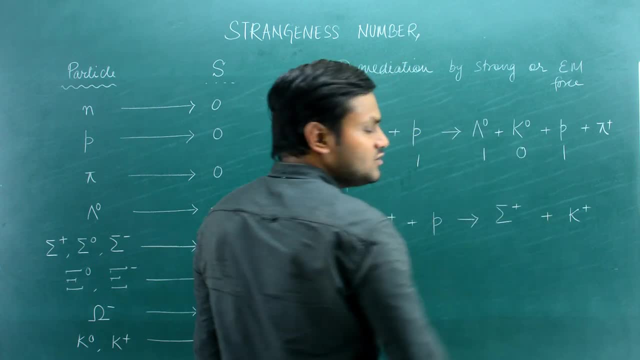 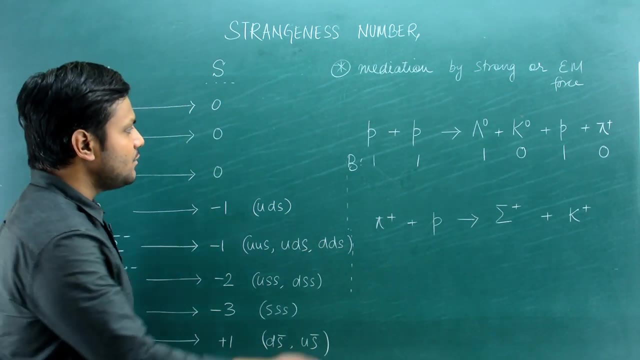 so that also has 1.. K naught is a meson particle, so it has a baryon number of 0.. Pi plus is a meson particle, so it is a baryon number of 0.. Now if you look at the strangeness number protons have 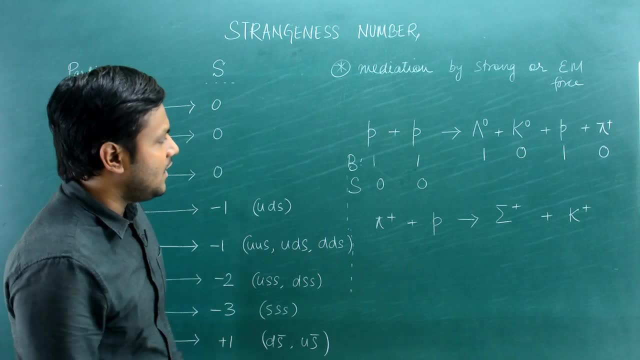 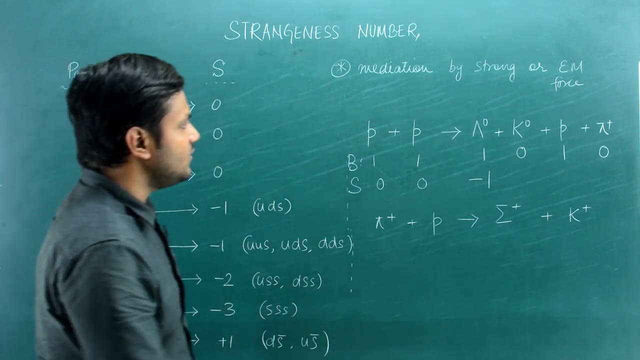 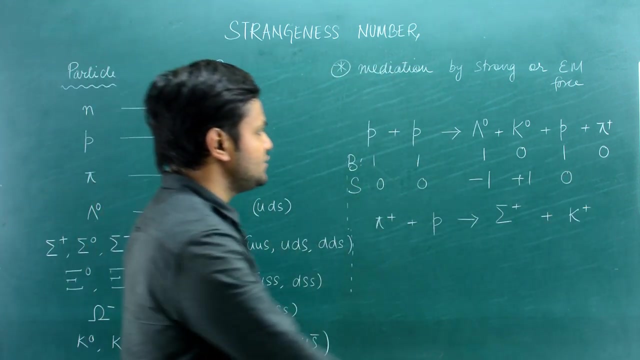 a strangeness number of 0. right, The lambda naught has a strangeness number of minus 1. okay, K naught has a strangeness number of plus 1. all right, Proton has a strangeness number of 0 and pi mesons have a strangeness number of 0.. So, as you can see, the baryon number is, of course. 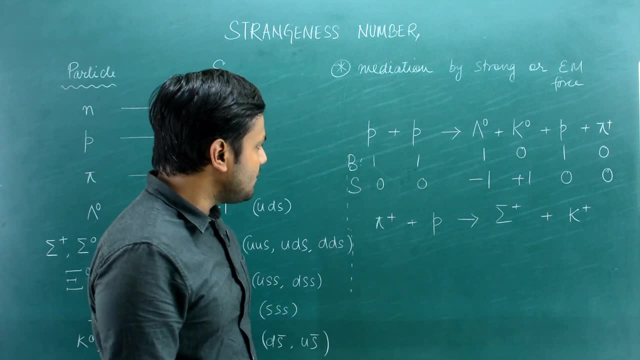 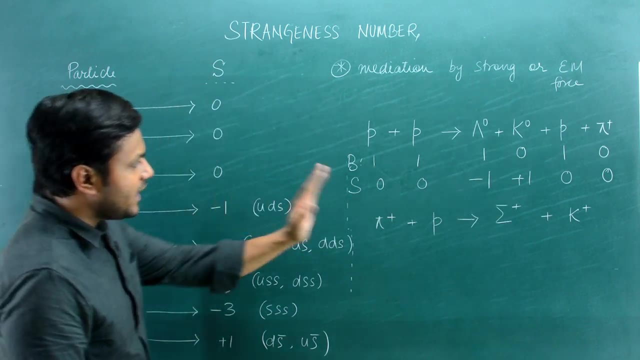 conserved: left hand side 2, right hand side 2.. The strangeness number: left hand side: 0. right hand side: 1 minus 1, 0.. So the strangeness number is also conserved In this particular case. now let's go ahead and look at this next interaction, where a pi meson or 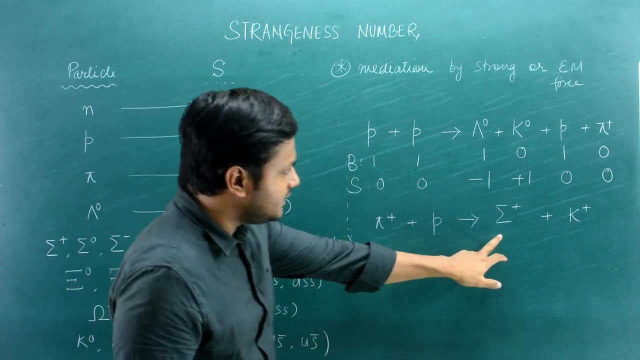 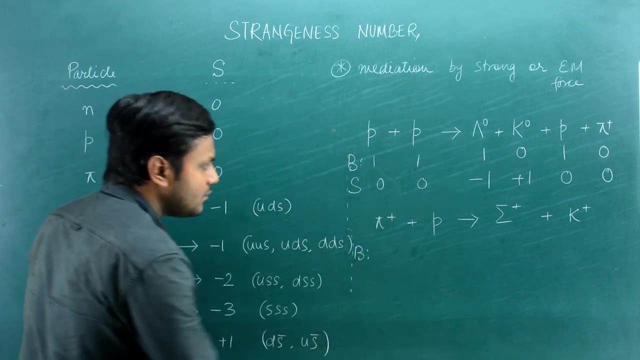 an entire pi meson interacts with a proton to create this kind of a sigma particle and a k1 particle. okay, So again I can associate the baryon number here. So a baryon number of a pi meson is 0.. 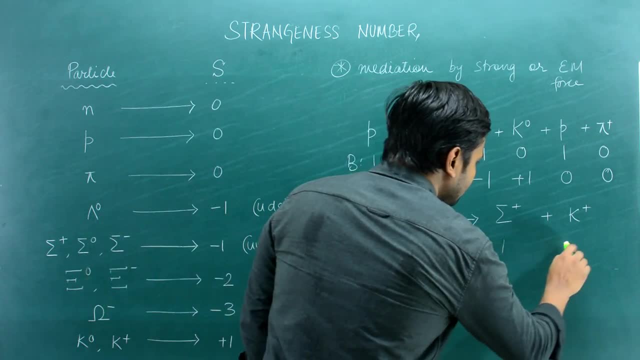 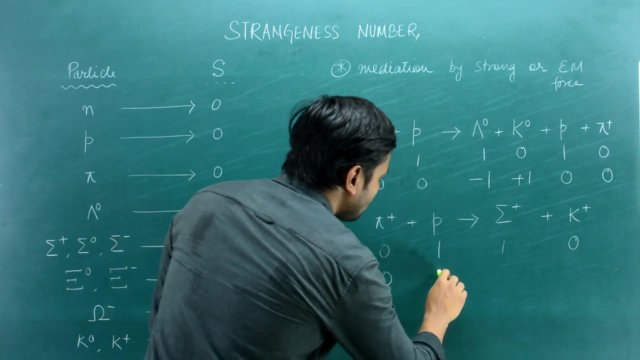 For a proton, it's 1.. For a sigma particle, it's 1.. For a k1 particle, which is nothing but a meson, it's 0.. And the strangeness number for a pi meson is again 0.. For a proton is again 0.. For a sigma. 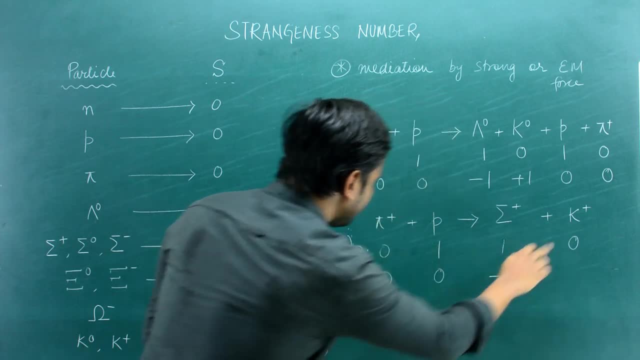 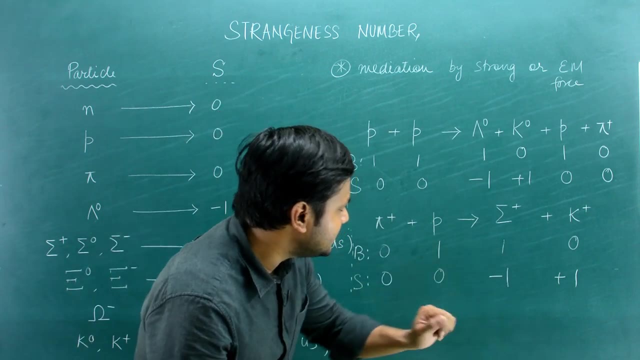 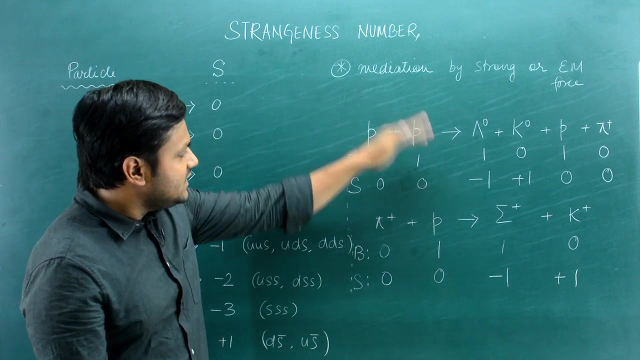 particle is minus 1 here and for a k plus particle is again plus 1.. So, as you can see, the baryon number is one left hand side, one right hand side. it's conserved. So, strangeness, number is 0 left hand side, 0 right hand side. it's conserved. So in these interactions, which are usually 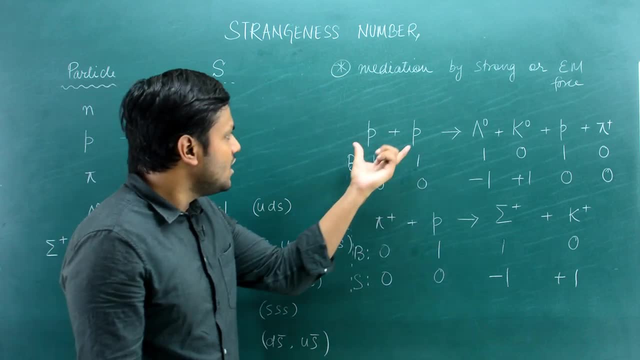 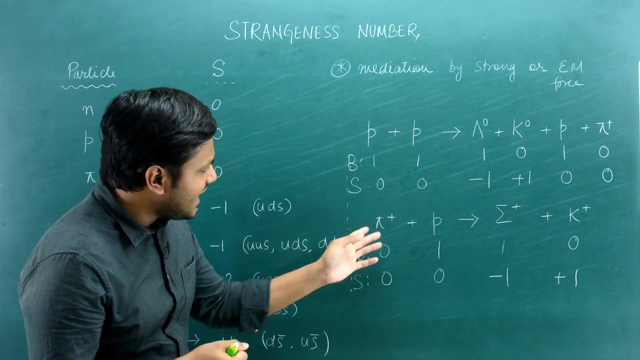 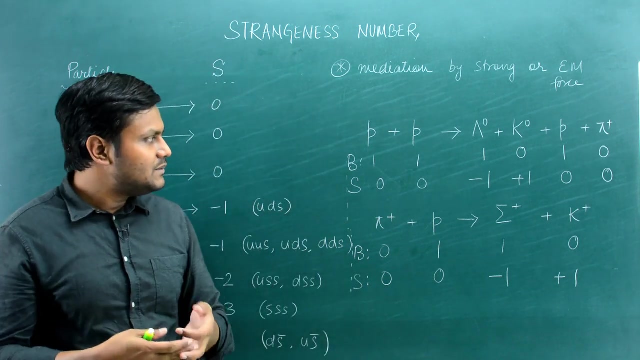 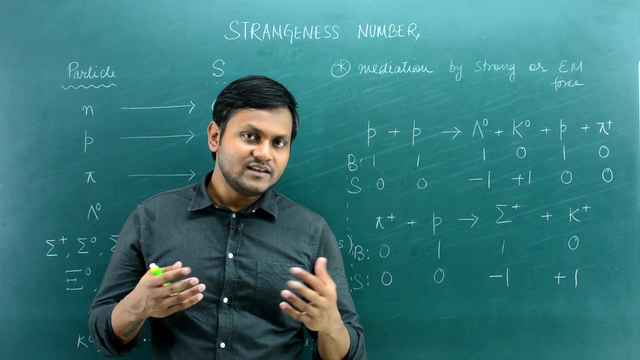 mediated by either a strong interaction or an electromagnetic interaction. So a proton and proton colliding is basically strong interaction and and also involves electromagnetic interaction, And same goes for the next one. in these kind of cases that strangest number is usually conserved. But if we look at particles like the baryon, particles decaying via weak interaction, So if 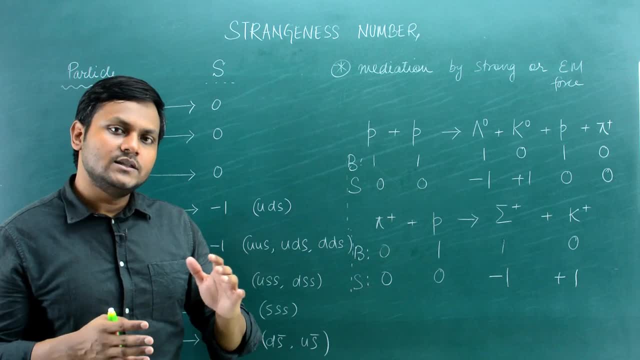 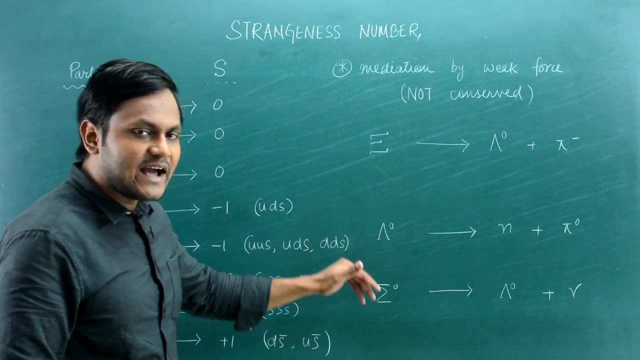 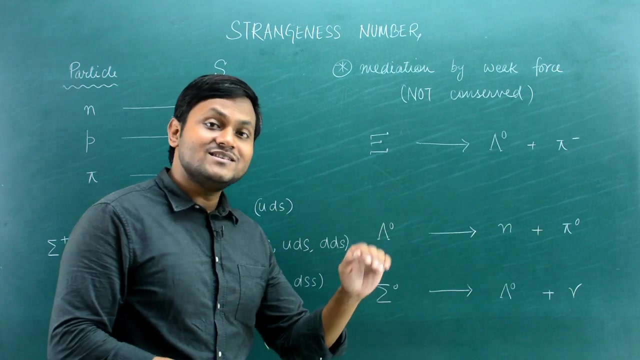 a strange particle decays via weak interaction, then in those cases the strangest number is not conserved. So again, let's look at a few examples. So here we have a couple of interactions that involve decays of strange particles, interactions. now, as it turns out, in weak interactions the strangeness number is not. 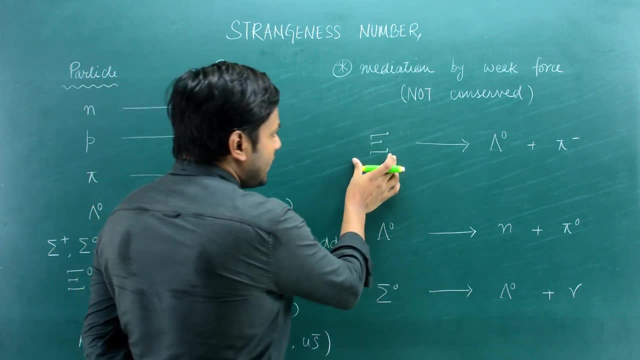 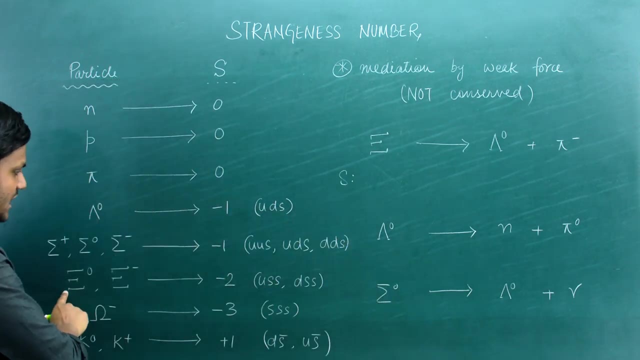 conserved. okay, so if you look at this particular interaction where xi particles becomes a lambda particle and a pi meson, so if you look at the strangeness number as it turns out, the xi particle has a strangeness number of minus 2 right, while the lambda particle has a strangeness number of. 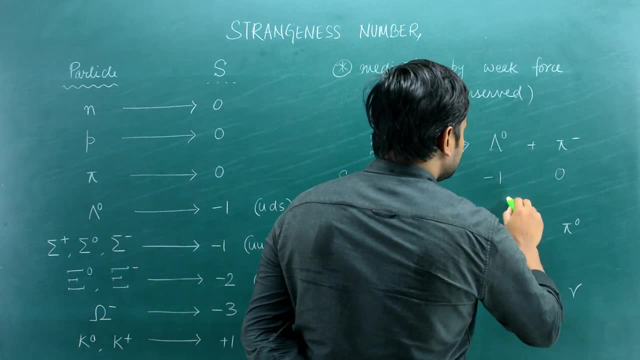 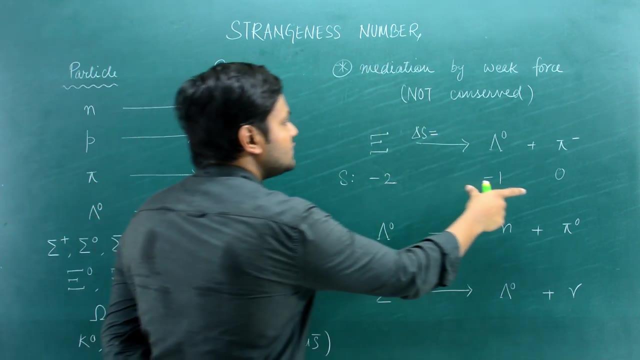 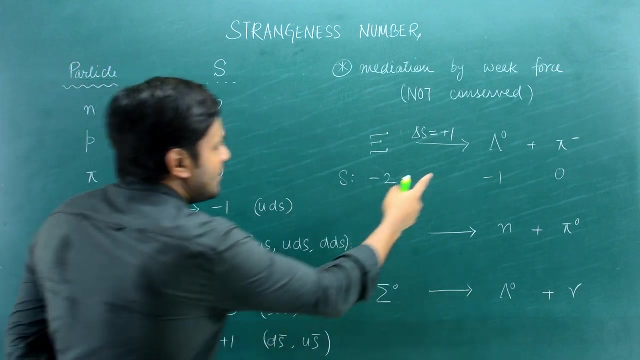 minus 1 and pi meson has a strangeness number of 0. so what is the change involved here? so what is the change in the strangeness number? so minus 2 becomes minus 1, so it is plus 1, so the overall the strangeness number changed by a value of plus 1, the lambda, not particle, may further decay. 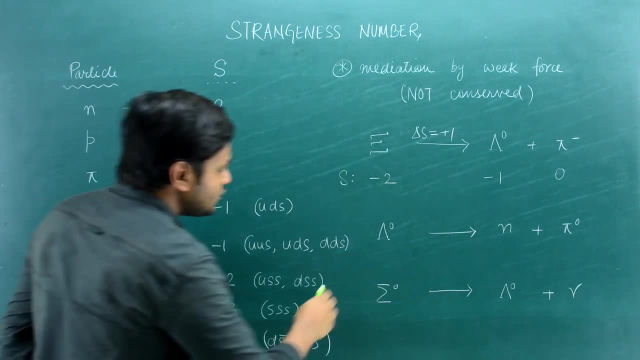 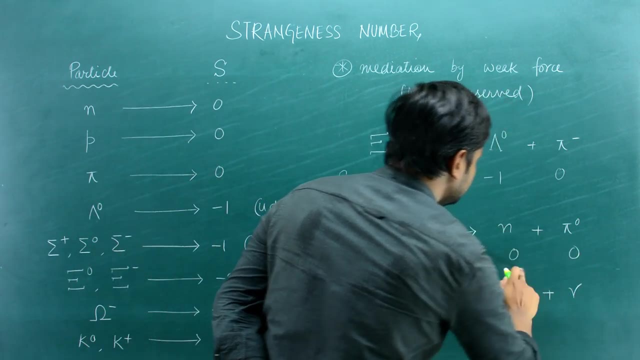 into a neutron and a neutral pi meson. so in this case the strangeness number will have a value of minus 1 right and 0: 0. okay, neutron and pi meson have values of 0: 0 for strangeness number, so in this case also left. 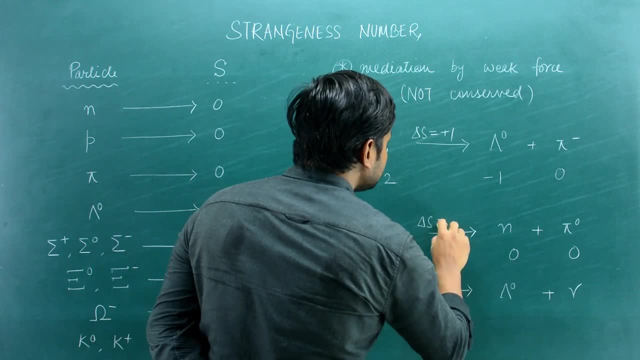 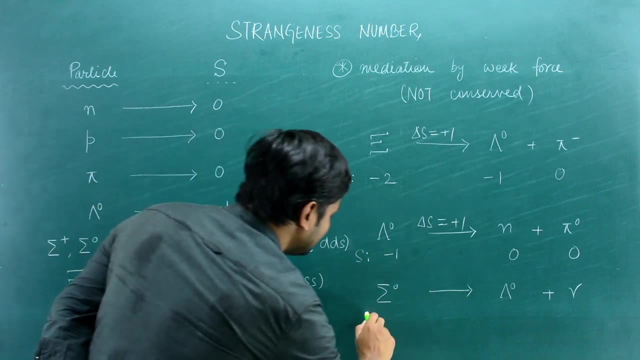 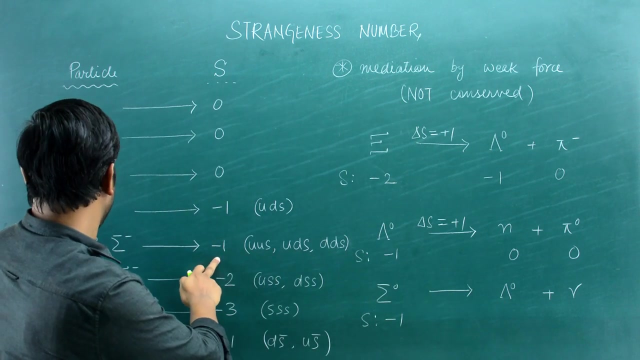 hand side minus 1. right hand side 0. so there is a change in a strangeness number by plus 1 right. in the last case we have the sigma particle, which also has a strangeness number of minus 1. it becomes a lambda particle which has a value of minus 1, and a gamma photon, which is a strangeness. 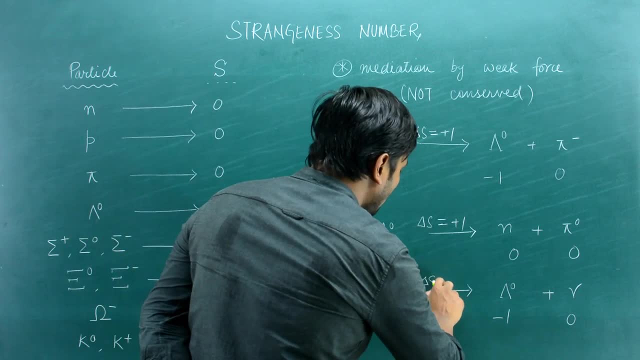 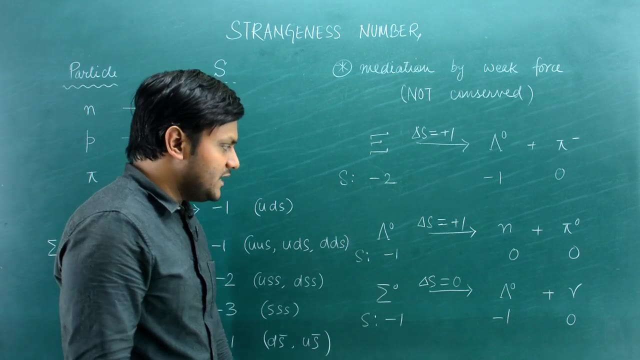 number of 0. in this case, however, the strangeness number did not undergo any change. so there is a change of 0- left hand side also minus 1. right hand side also plus 1. left hand side also minus 1. right hand side also minus 1. so as it turns. 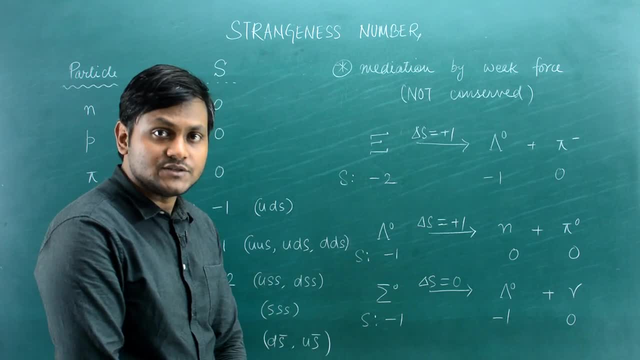 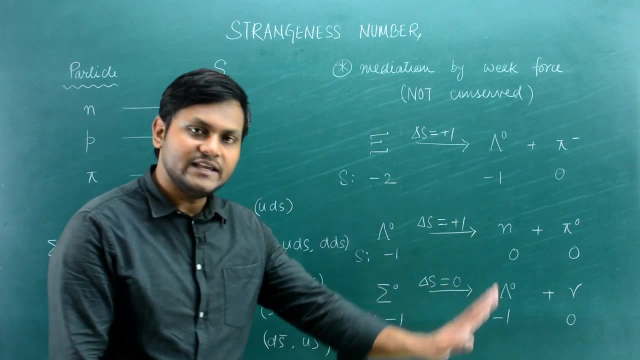 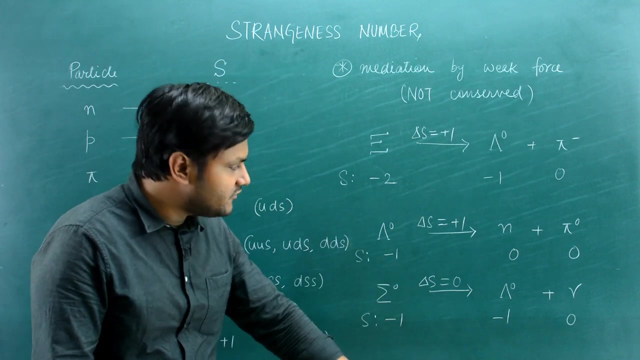 out in the case of weak interactions, where strange particles or particles that involved a strange quark undergo decay via weak interactions, then we cannot definitely say that the strangeness number is going to be conserved. in some cases it is conserved. in some cases it is not conserved. 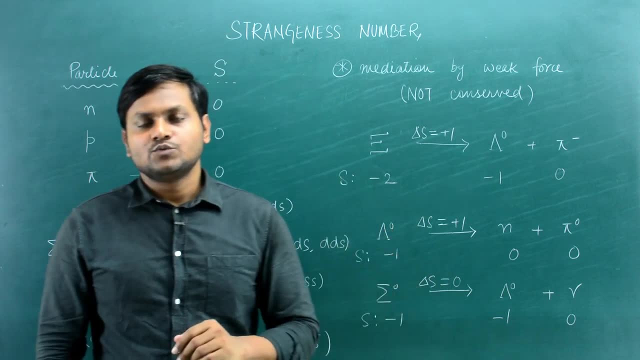 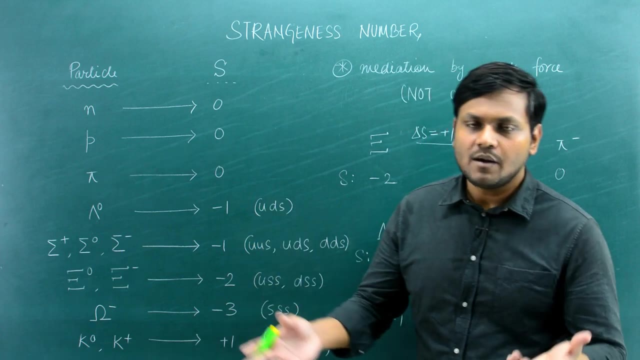 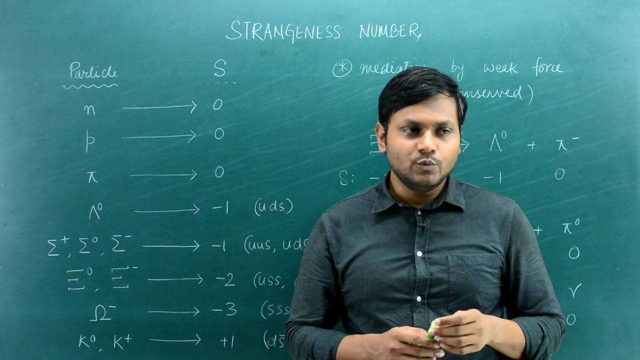 they may change by either plus 1 or minus 1. so that is all. this lepton number barrier number and the strangeness number are basically a set of rules based on studies over the last 50 years, which gives us an idea how different kinds of subatomic particles 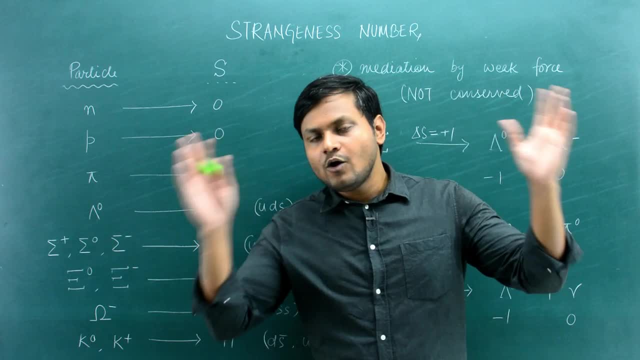 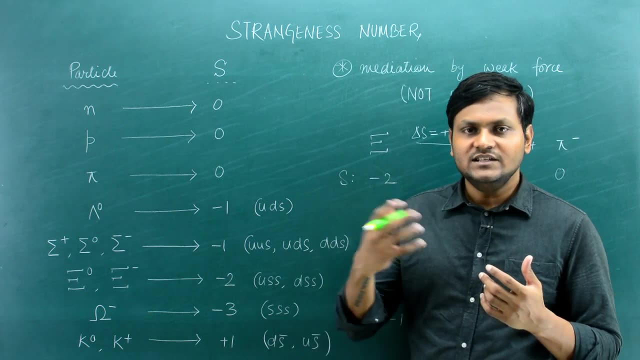 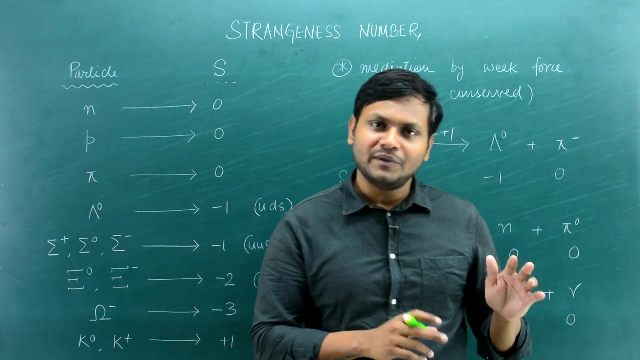 interact all right. so, out of all the chaos and diversity of different particle interactions, we have got some idea about these numbers that helps us get some confidence about what is happening and what sort of interactions are happening, what sort of interactions are allowed, what sort of interactions are not allowed. so before i finish the video, i want 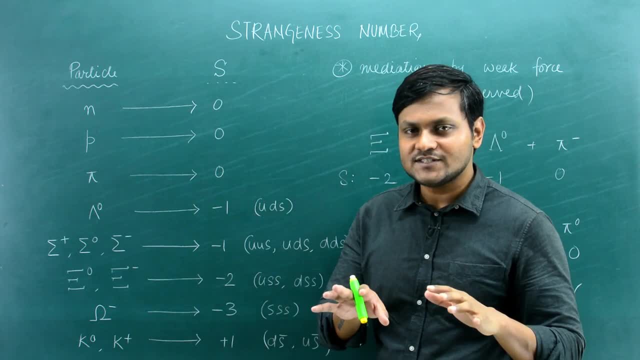 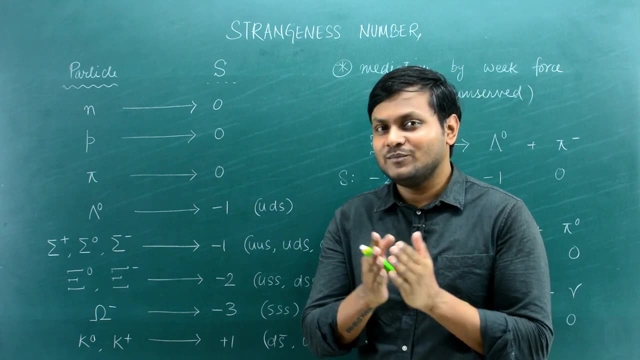 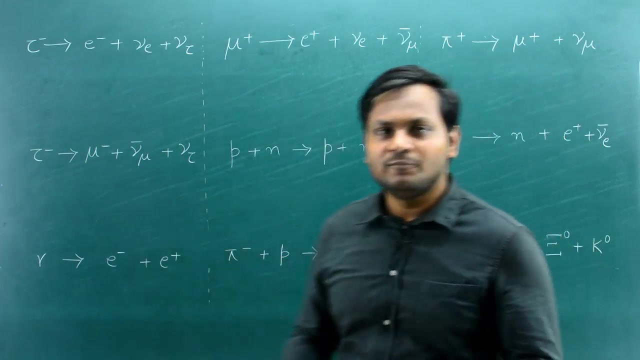 to do a little bit of a test. okay, so i'll give you a couple of interactions, some of which are allowed, some of which are not allowed, and you tell me whether or not they are possible or not based on what we just now discussed. okay, okay, so i have here a couple of particle interactions. 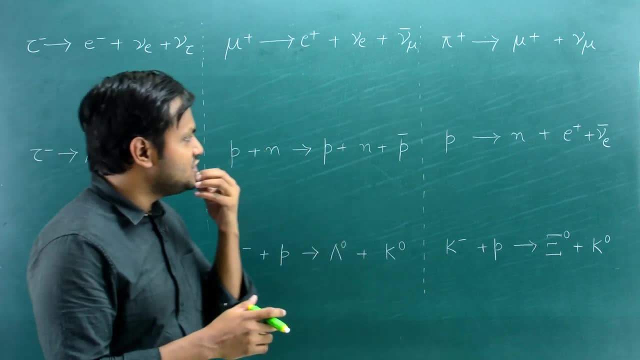 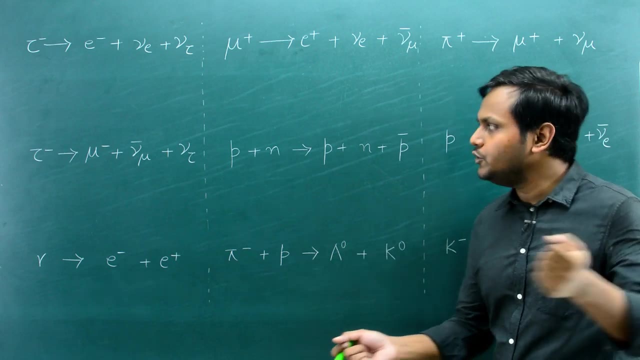 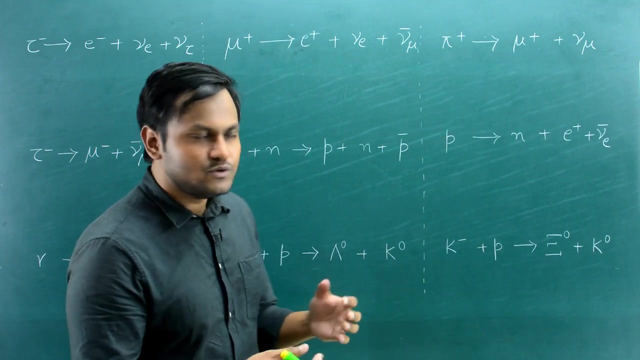 uh, some of which are possible in nature, some of which are not possible, and think of this as a kind of a test: based on what we just discussed in this video, can you determine which of these are allowed, which of these are not allowed, which of these happen in nature, which of these do not happen? 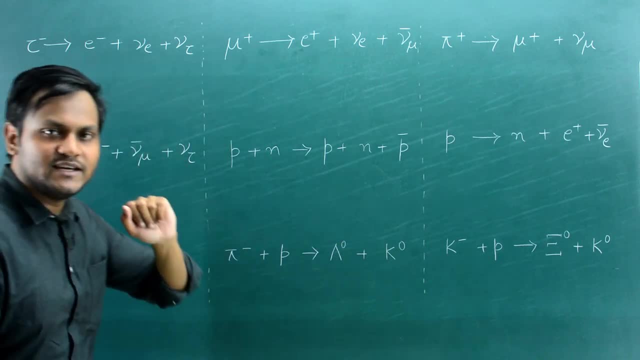 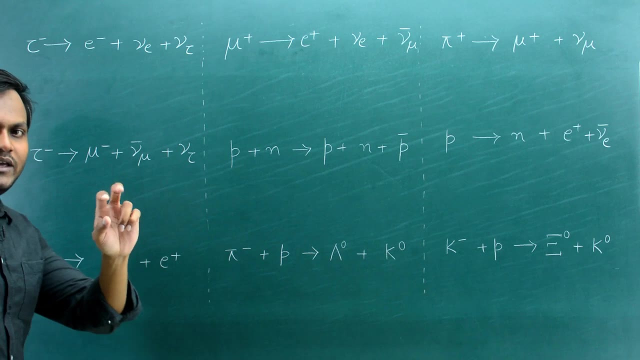 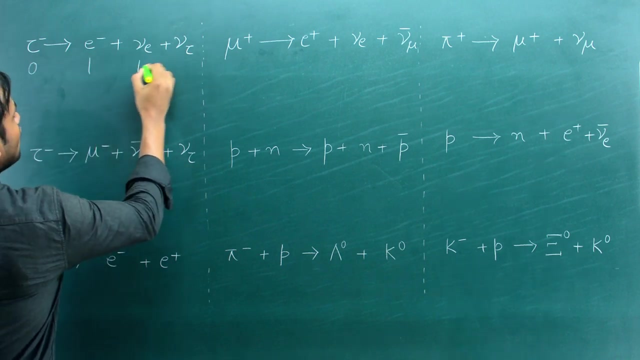 so let's look at them one by one, okay. so let's start with the first interaction. a tau particle becomes an electron and leads to emission of an electron neutrino and tau neutrino. okay, we here. we have to check the electron number and the tau number. so if you check the electron number, it turns out to be zero, one, one, zero, right. 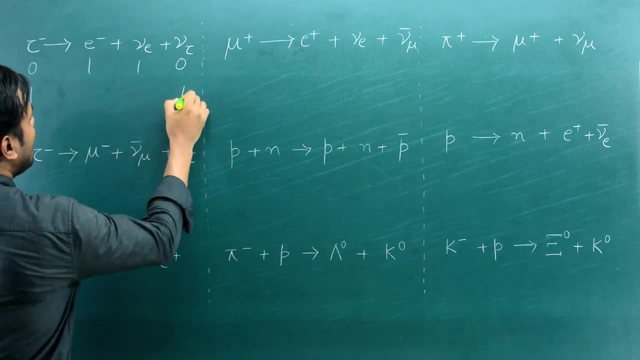 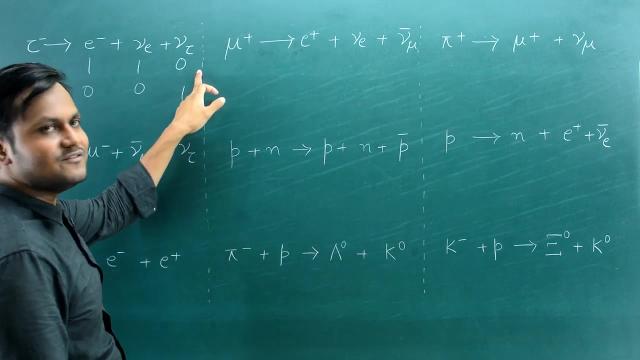 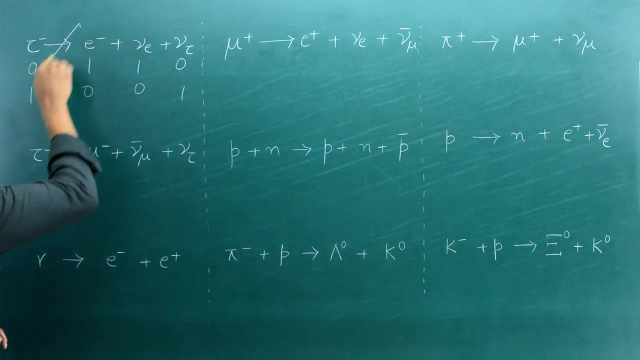 if you look at the tau lepton number, it comes out to be one one zero, zero. so the tau lepton number is conserved, but the electron lepton number is not conserved. the electron is being emitted along with an electron neutrino, which is not possible. so this is a reaction which does not happen in nature. let's 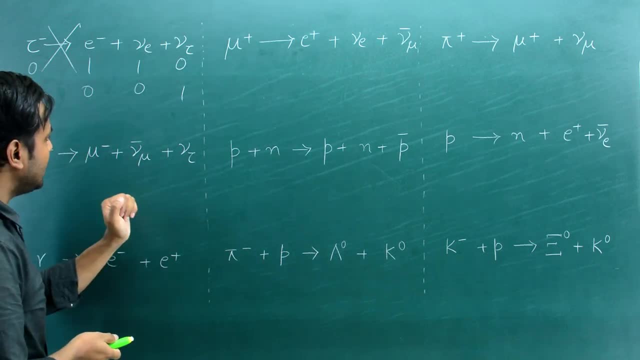 look at the second one. a tau becomes a muon and a muon entire neutrino and a tau neutrino is produced. so we will have to check the muon number as well as the tau number. so the muon number is zero one for the entire muon. 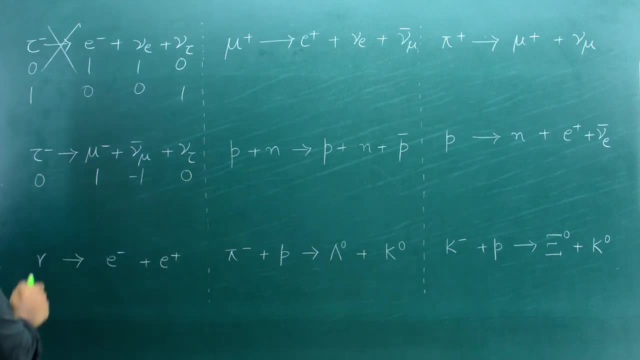 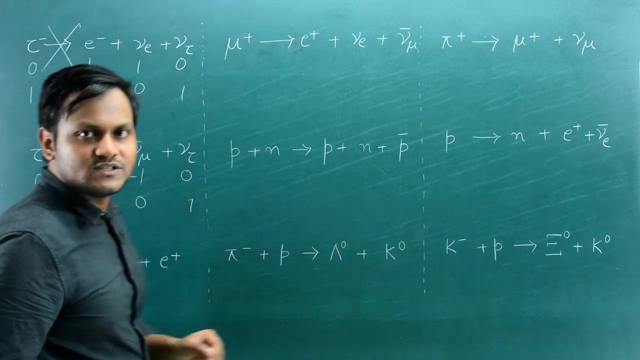 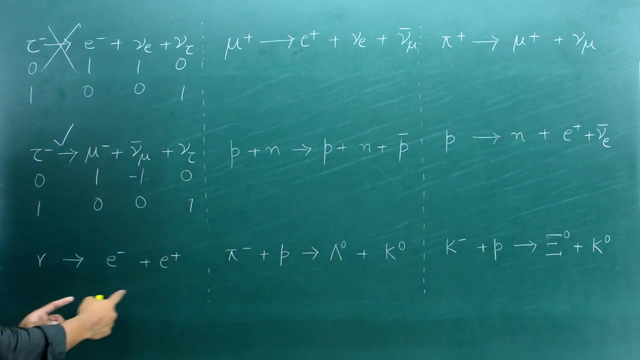 neutrino minus one and zero. right, the tau number is one and one zero zero. here. can you see, can you figure it out? so the muon number is conserved, one minus one zero. the tau number is also conserved. this is possible, see, right? the next is simply pair creation. a gamma photon becomes an electron and a positron. 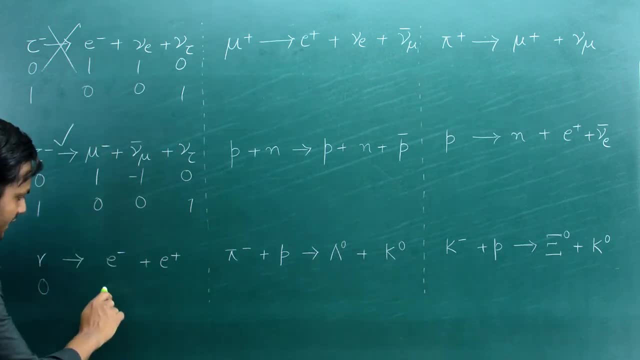 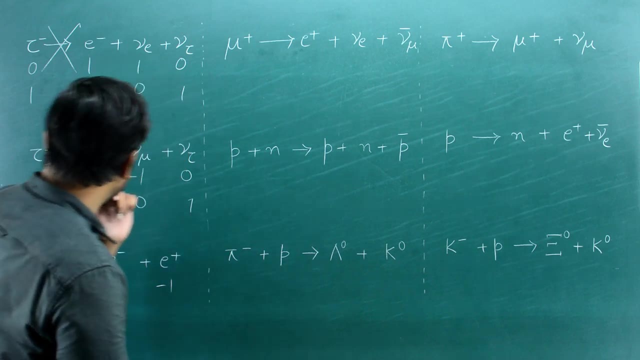 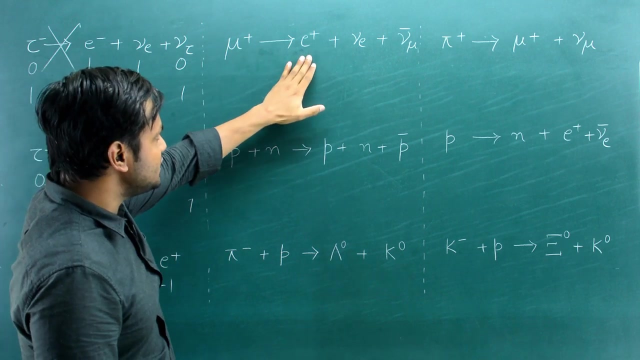 so if i look at the electron lepton number, the gamma photon has zero, electron has uh one and positron has minus one electron lepton number is conserved. this is allowed, so this is something that is allowed in nature. let's look at the next one. a muon anti-particle becomes a positron. 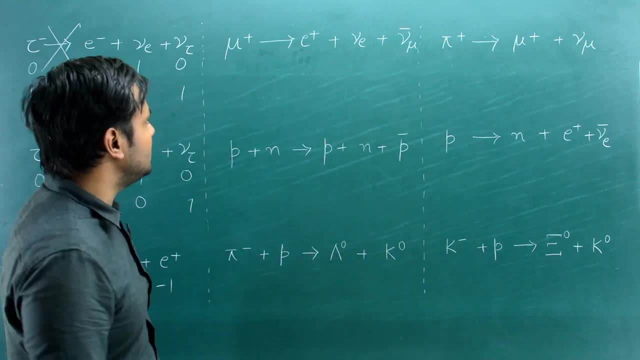 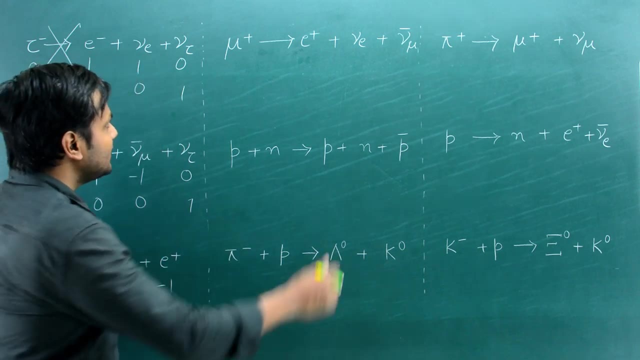 and electron neutrino and anti-muon neutrino is emitted in the process. so here we will have to check what the muon number and the electron number right? so let's look at the electron lepton number first. it is zero minus one one and zero right for the positron. 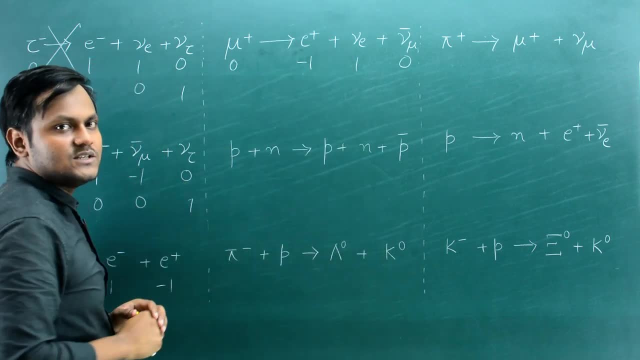 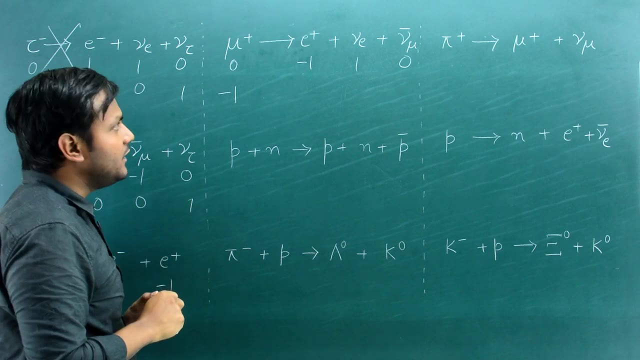 the electron lepton number is minus one. for electron neutrino it is plus one. now, what about the muon lepton number? it is minus one because mu plus is the anti-particle of a muon, all right, and the anti-muon neutrino is also minus one and zero, zero here. so here, 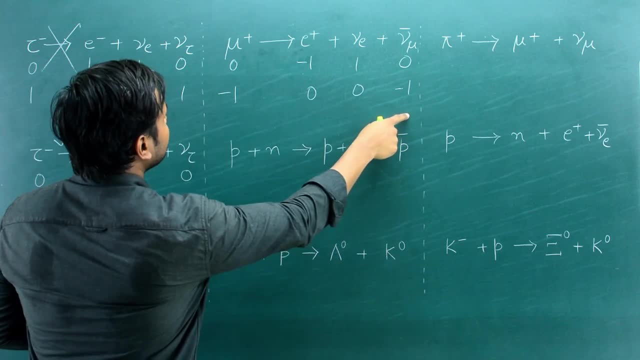 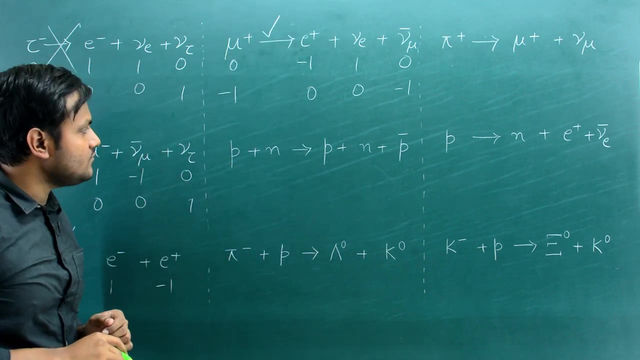 it seems that both are conserved, minus one. minus one here for the muon number, and minus one plus one zero for the electron number. so this is the interaction which is allowed. let's look at this one. this consists of protons and neutrons, so we'll have to check for what we'll have to check for. 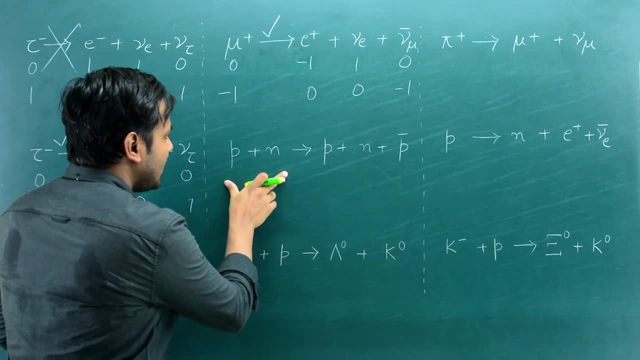 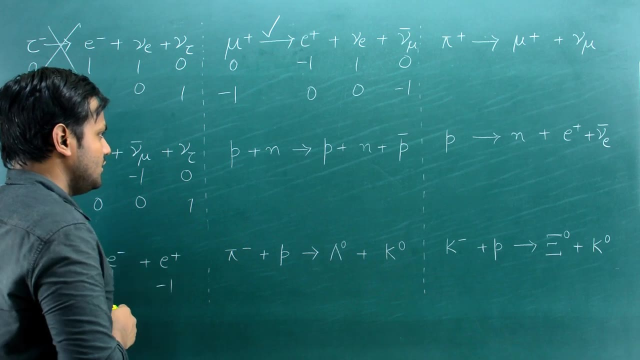 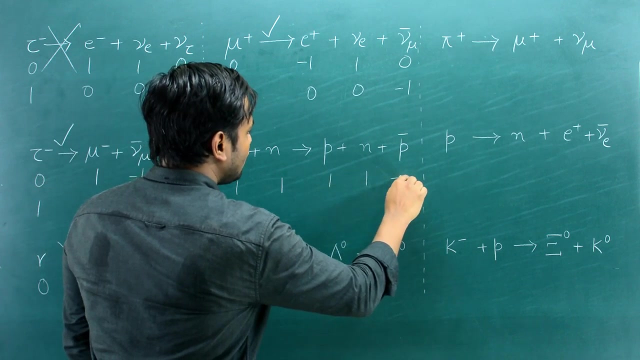 the barrier number in this case. okay, so proton and a neutron under high energetic interaction leads to the creation of a proton and neutron and an antipositron- sorry, anti-proton, all right, so if we have a proton and a neutron and a neutron it's one. so the barrier number for a proton and 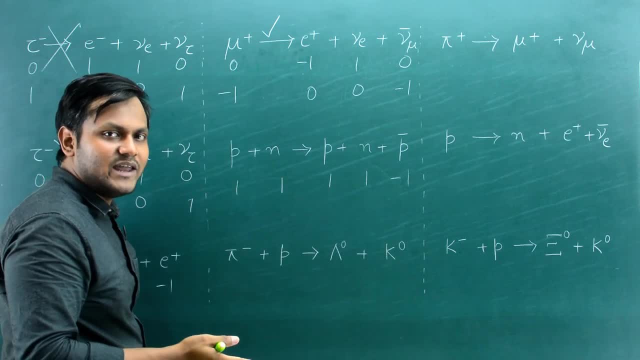 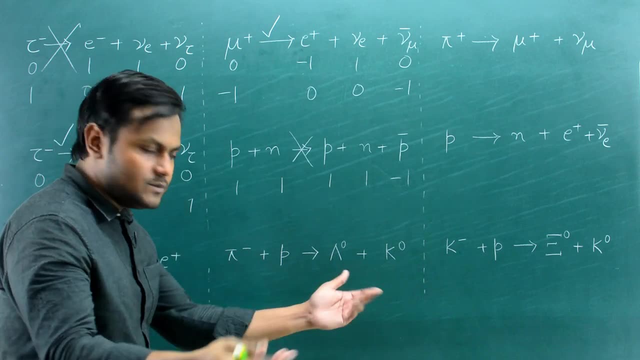 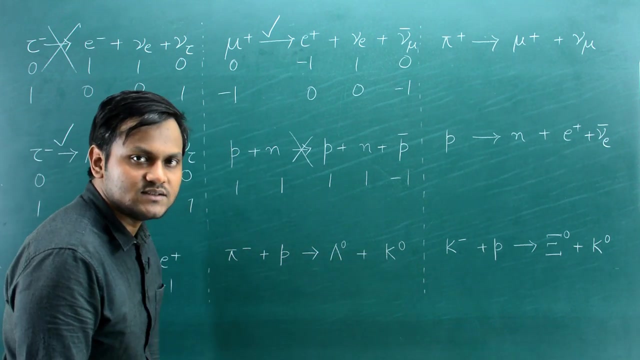 neutron is one. proton neutron is one. anti-proton is minus one left hand side two, right hand side one. this does not lead to the conservation of barrier number, which is not seen in nature. okay, barrier number is always conserved, so this reaction is not possible now. let's look at the next one now. 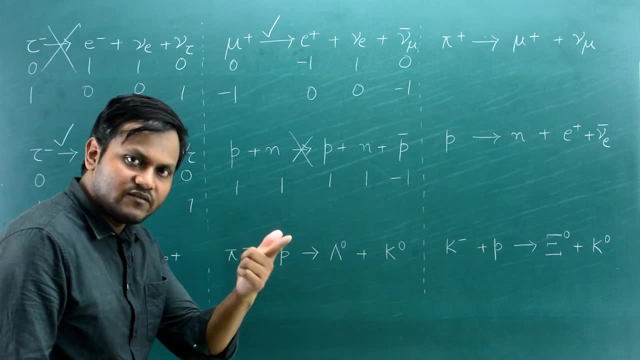 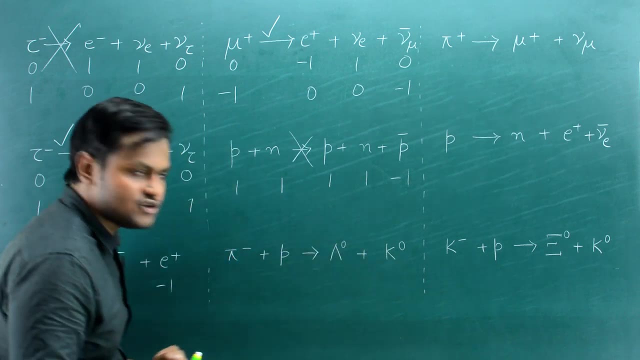 this involves not only baryon particles, but also strange particles, the hyperion particles. that strangeness conservation Now, because a meson and a proton are interacting. so this is a strong interaction. So I expect that strangeness number should be conserved, if this reaction does indeed. 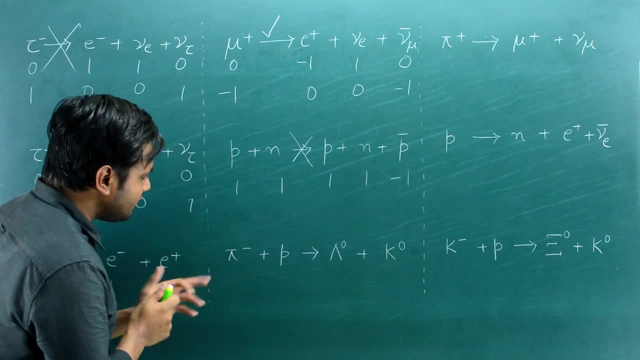 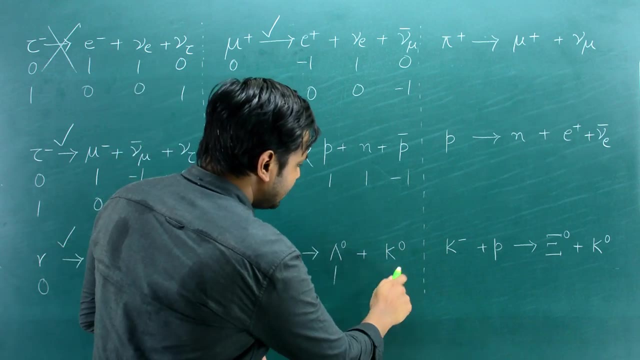 happen in nature. So first let us look at the baryon numbers. A baryon number for a pi meson is what 0.. For a proton is what 1.. Lambda naught is a baryon particle, so it is 1.. K-on is a meson. 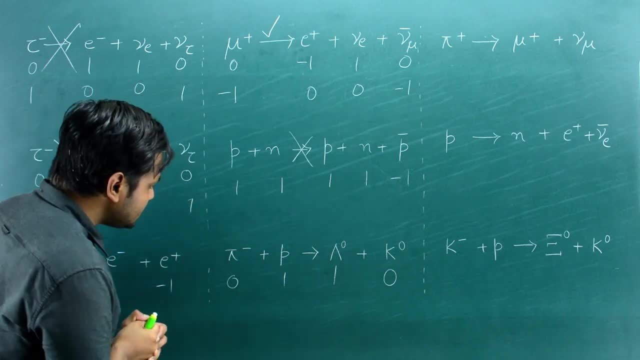 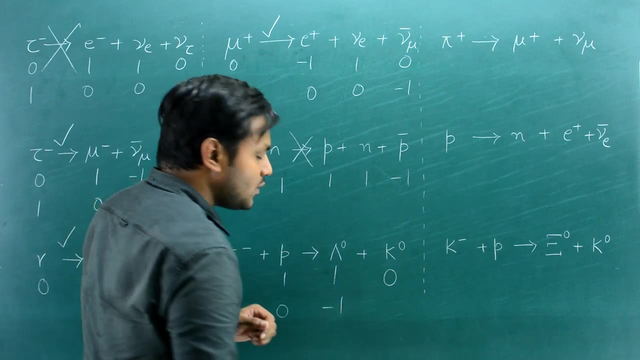 particle, so it is 0.. Let us look at the strangeness number. Strangeness number for a pi meson, as well as a proton, is 0 and 0.. The strangeness number for a lambda is minus 1, but for k naught it is. 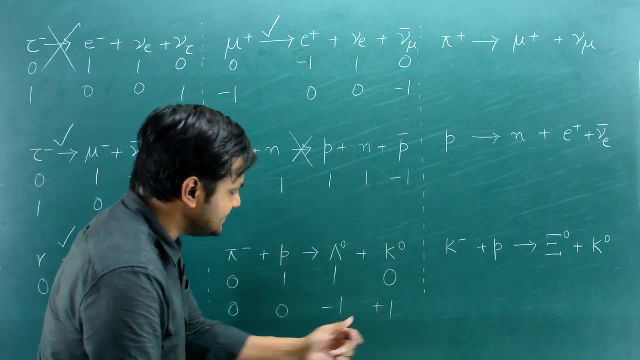 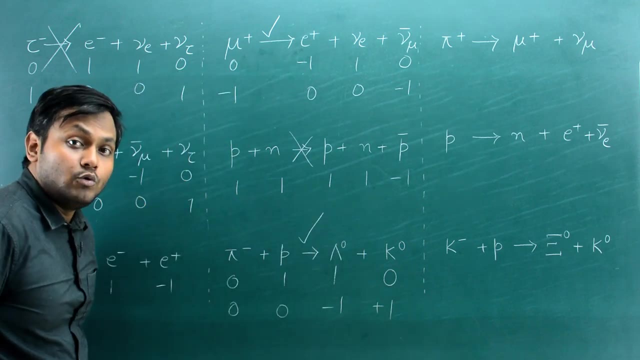 plus 1.. So the strangeness number is conserved. Okay, minus 1 plus 1,: 0 right hand side, 0 left hand side. So this, indeed, is a interaction that is allowed in nature. Now let us go to the next. 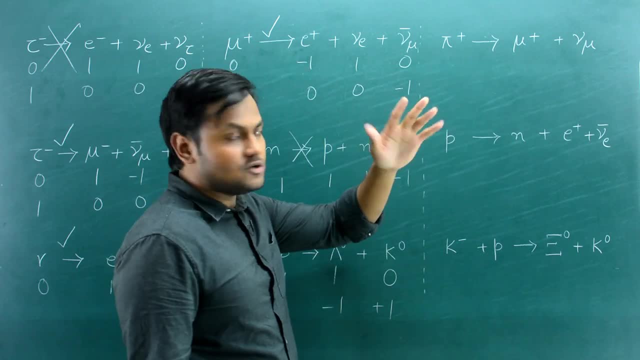 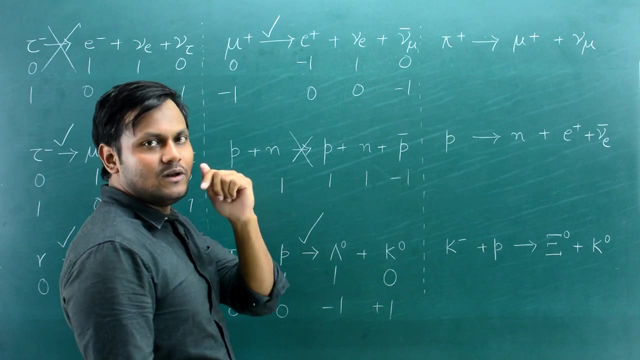 one, A anti-particle for a pi meson or anti-pi meson becomes an anti-muon and leads to the emission of a muon neutrino. So here we will have to look up muon lepton number right. So the muon lepton number for a pi meson. 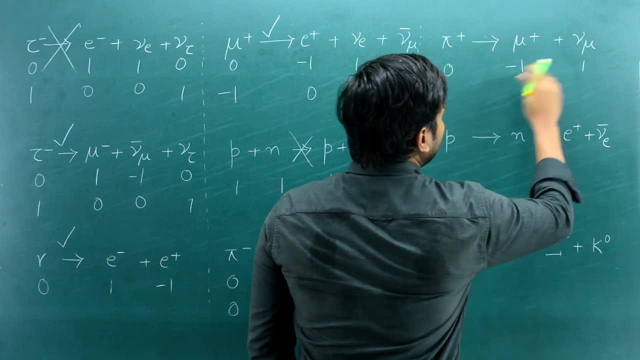 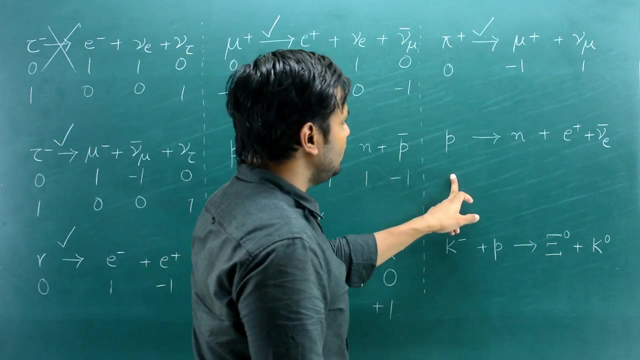 is 0.. For an anti-muon is minus 1 and for a muon is 1.. So this muon lepton number is conserved. This is allowed. Now let us look here. Here we need to check both the lepton numbers for electron. 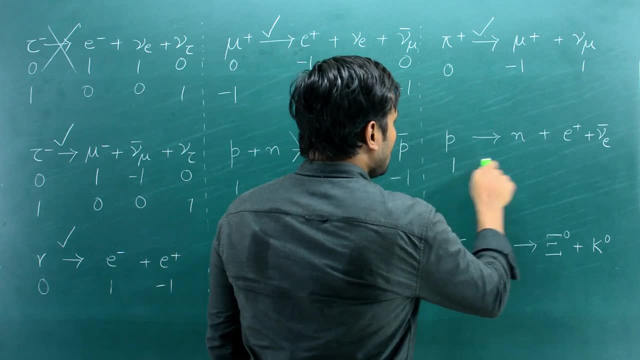 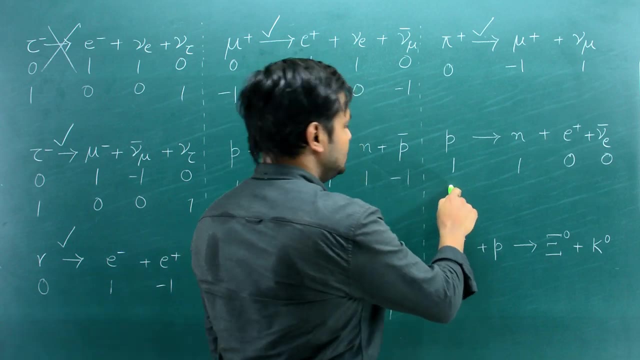 as well as the baryon number. So the baryon number is 1 and 1 is conserved. Okay, but what about the electron lepton number? Electron lepton number for a proton is what? 0.. Neutron is what? 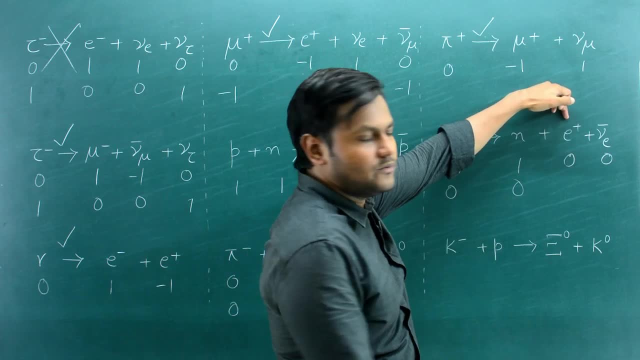 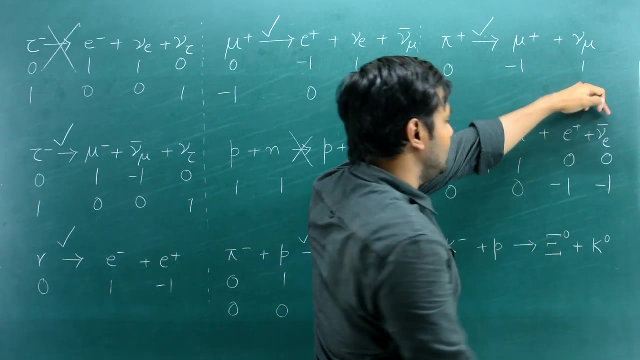 What is the electron lepton number for a positron Minus 1, right? What is the electron lepton number for an anti-electron neutrino Minus 1, right? The electron lepton number is not conserved. 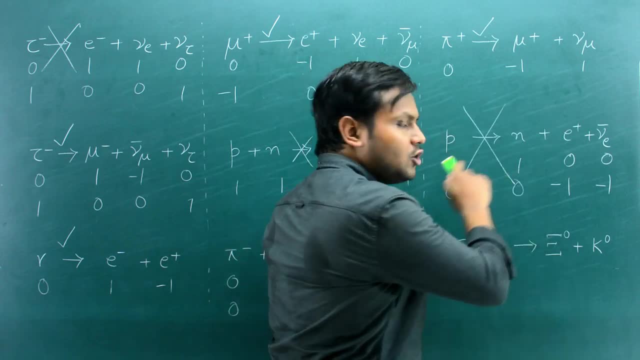 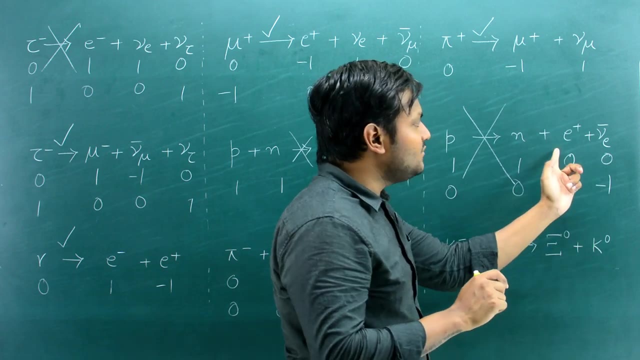 Left hand side is 0, right hand side is minus 2.. This is not possible, So a positron and an electron anti-neutrino will not be emitted together. okay, Electron can be emitted with an electron anti-neutrino and positron can be emitted with an electron neutrino. 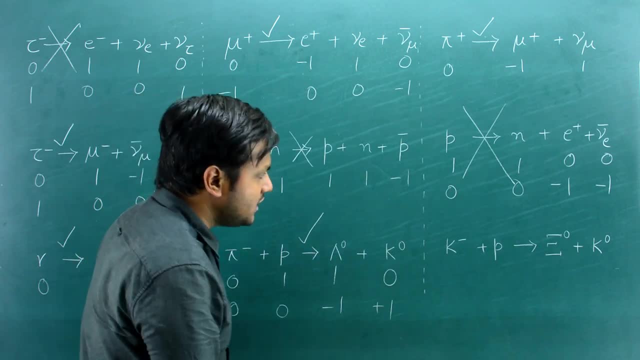 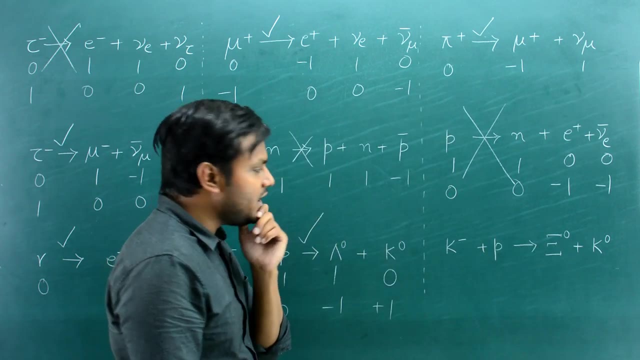 But this is not going to happen. So this is a reaction that does not happen at all. Finally, we have this kind of a K1 particle: proton leads to a xi particle and another K0,. all right, So here we will have to check the baryon number. The baryon number is 0 for K0,. 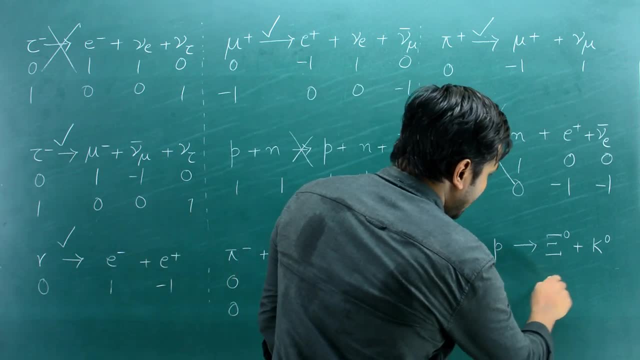 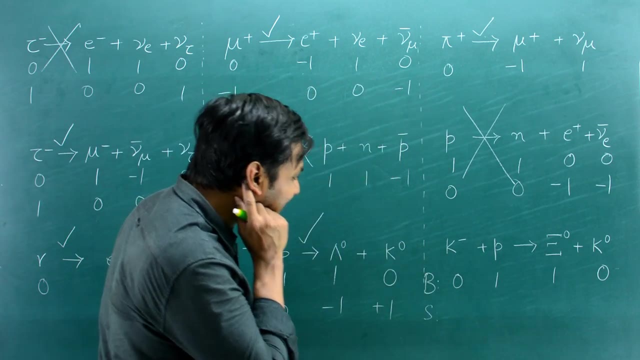 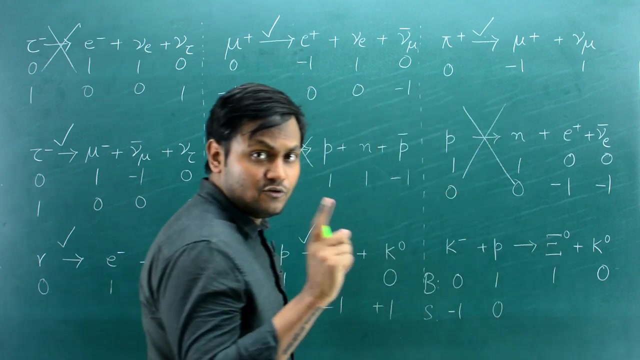 K minus, which is a meson particle, 1 and 1 and 0, okay, So the baryon number is conserved, But what about the strangeness number? The strangeness number for K minus is basically 0 for a xi particle, If you remember from my table previous that I have shown is minus 2. 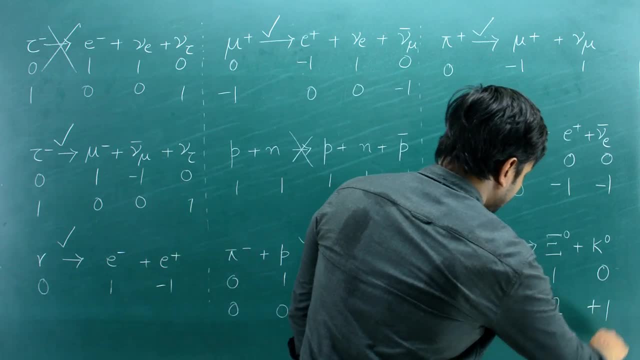 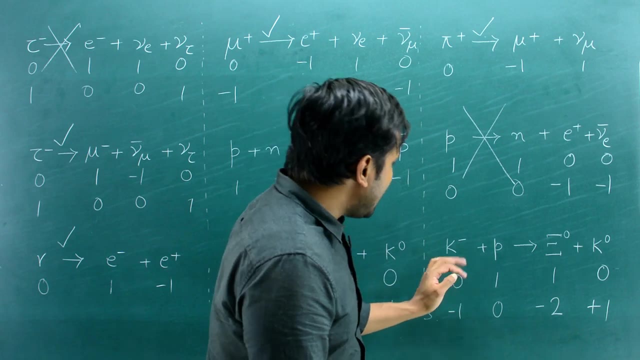 and for K, naught is basically equal to plus 1.. So strangeness number is minus 1 left hand side and minus 2 plus 1 is also minus 1 right hand side, So strangeness number is also conserved, and I see that this is a strong interaction. So therefore this reaction is possible. 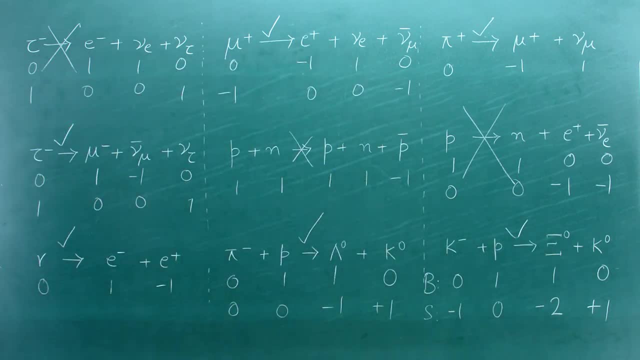 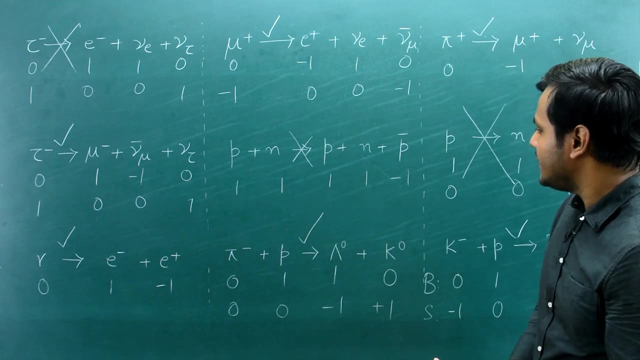 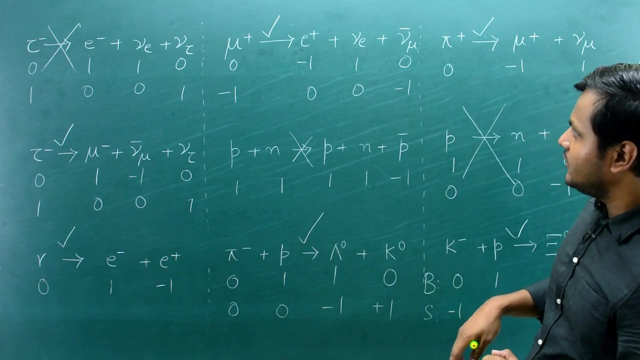 So, as you can see here, I had a set of different kinds of particle interactions and by applying the lepton number- conservation- the baryon number- conservation- and the strangeness number- conservation for strong interactions, I can figure out which one of them are allowed and which one of them. 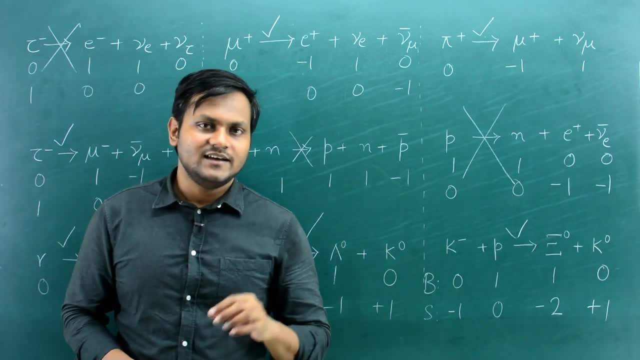 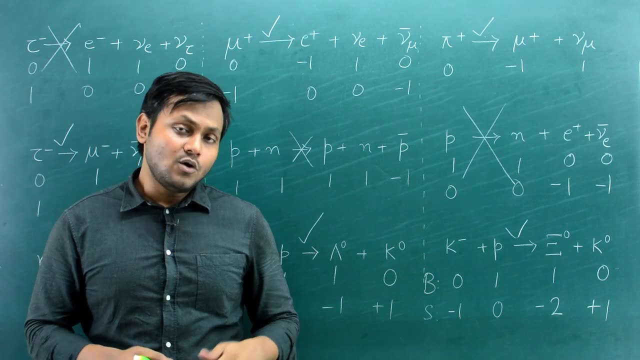 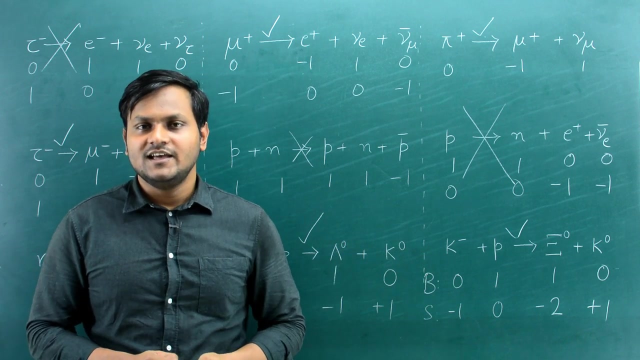 are not. So, in a sense, these quantum numbers give you an idea about which of these particle interactions do indeed happen or not. So, in a way, giving you a clue, a kind of a confidence in the chaos of particle interactions. So that is all for today.